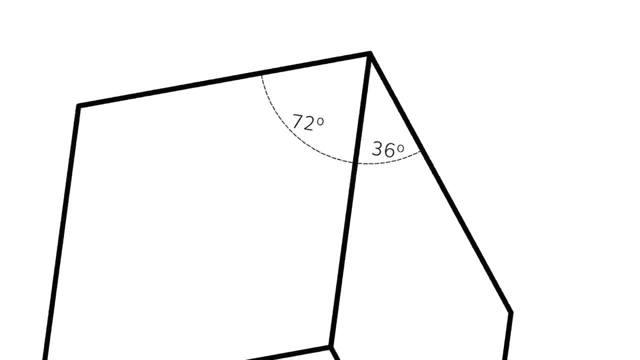 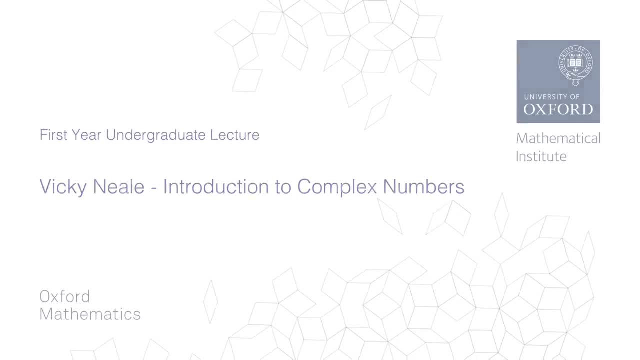 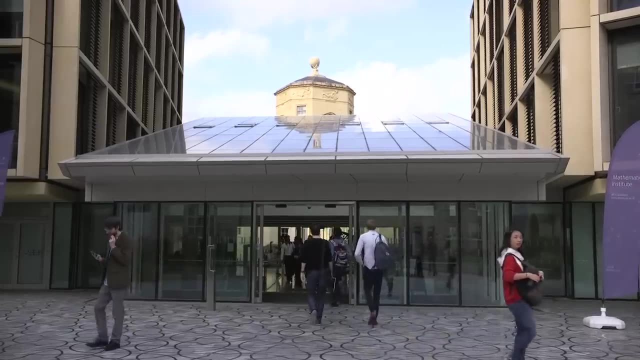 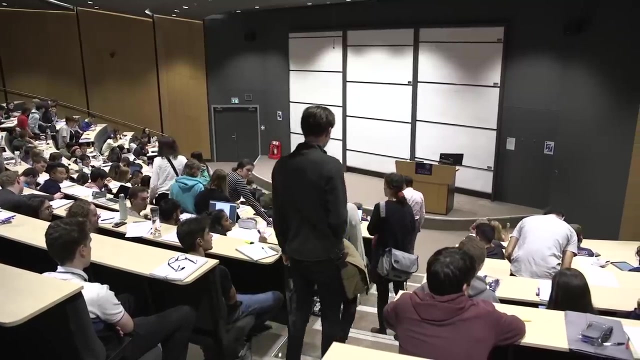 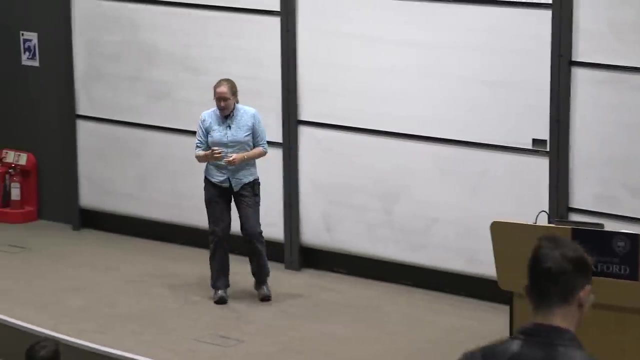 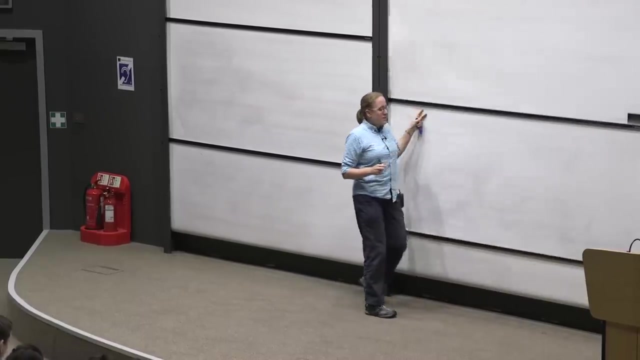 Good morning everyone. We're on complex numbers. So just at the end of the last lecture we were thinking about the argument of a complex number And I'd like to keep going from there a little bit. So sort of thinking about Cartesian coordinates, polar coordinates. 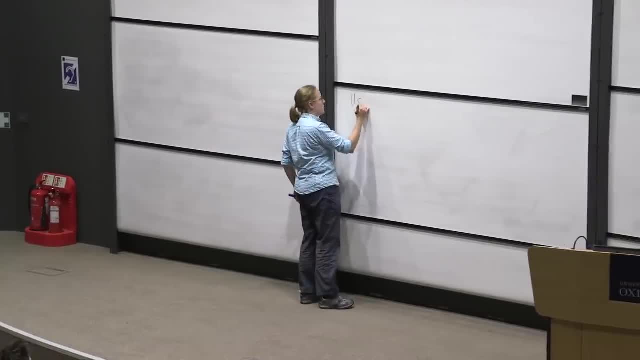 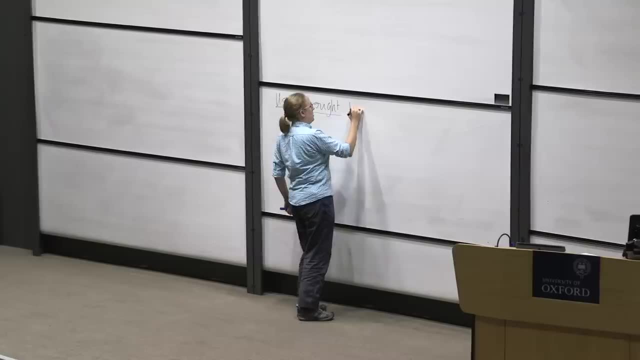 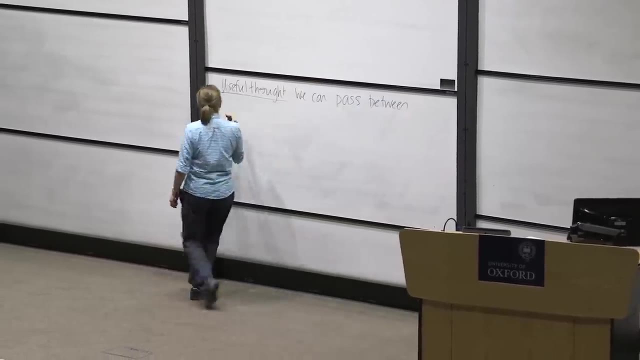 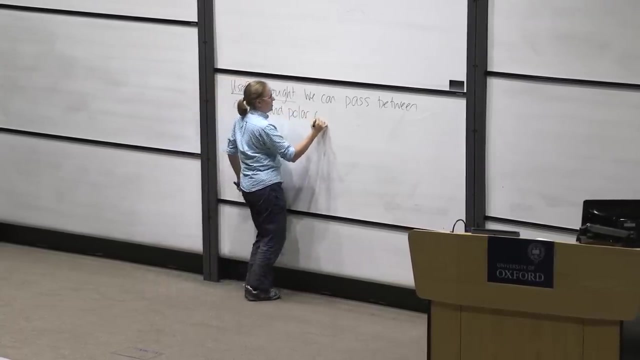 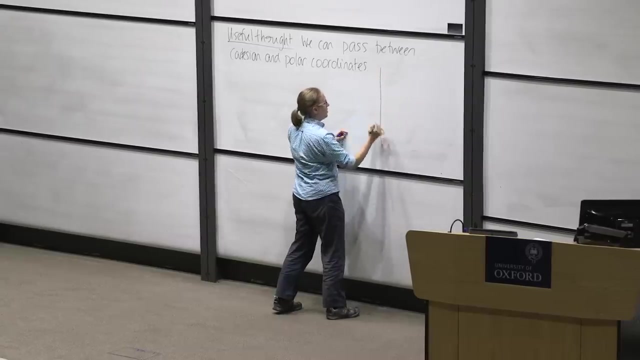 and it's really important that it's convenient to pass between the two of those. So here is a useful thought: So we can pass between Cartesian and polar coordinates. So here's my kind of picture of what I'm doing. So this is my. 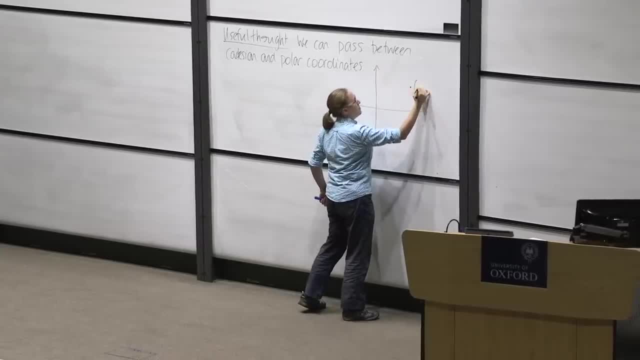 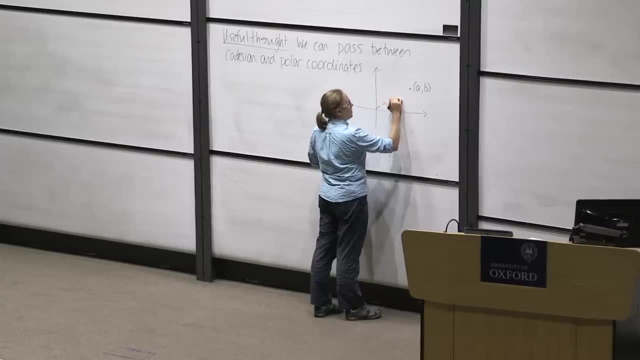 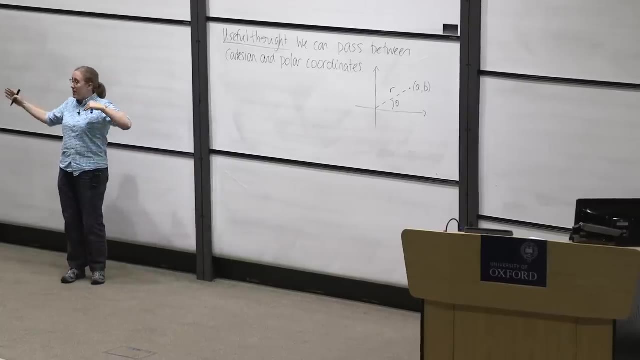 Argand diagram, my complex plane. Here is some little complex number which I might think of as having Cartesian coordinates or I might think of as having modulus r and argument theta, And I'd like to know, if I know a and b, can I find r and theta? 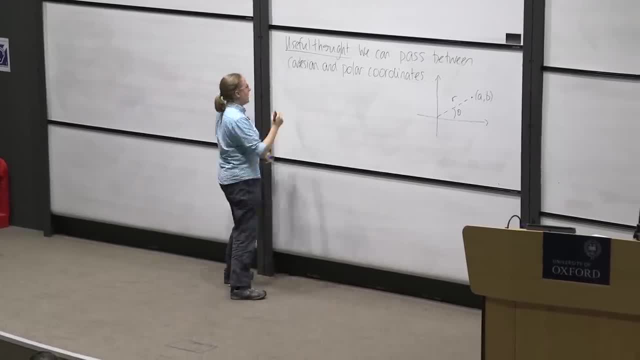 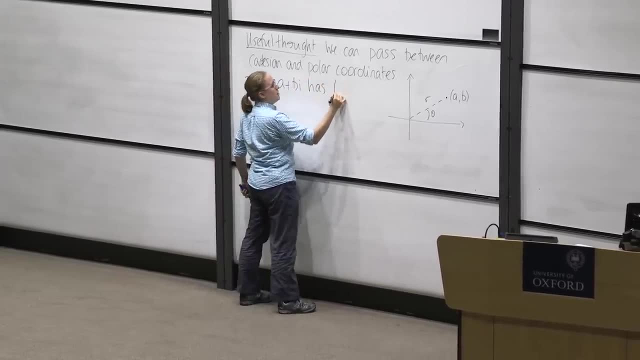 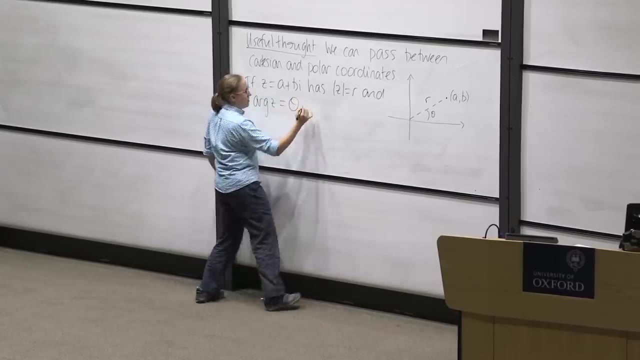 If I know r and theta, can I find a and b? That's the kind of point here. So if z, which is a plus b i, has modulus r and argument theta, then we can find a and b. So maybe I'll draw this on here in another colour for you. 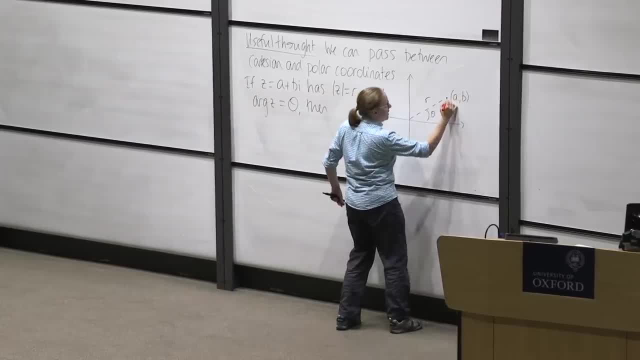 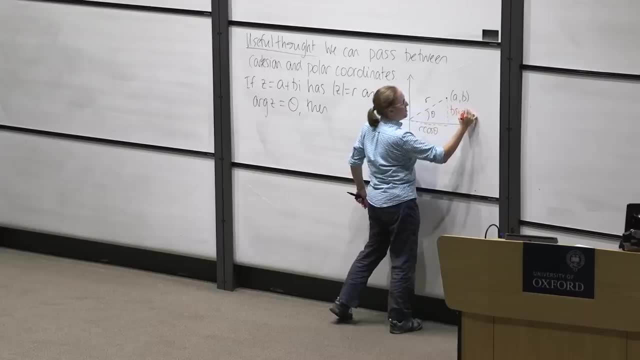 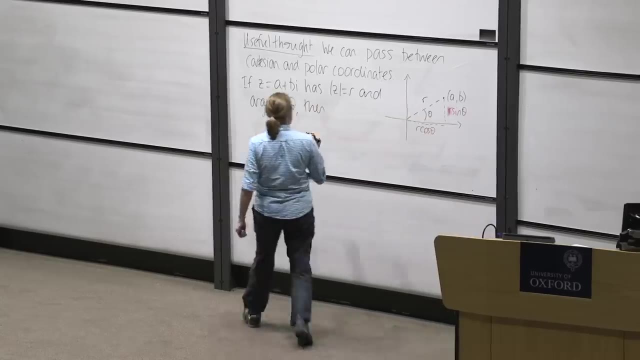 So this is just a little bit of trigonometry. So this bit is r cos theta, this is a, this is b sine theta. sorry r sine theta. Let's try that again. which is b. So a is r cos theta and. 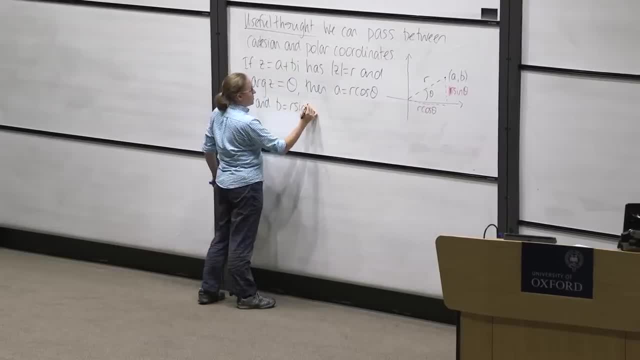 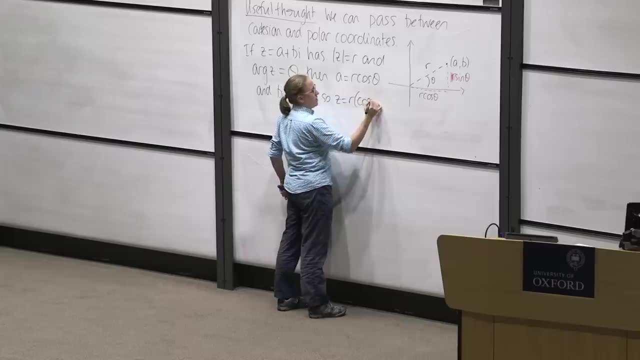 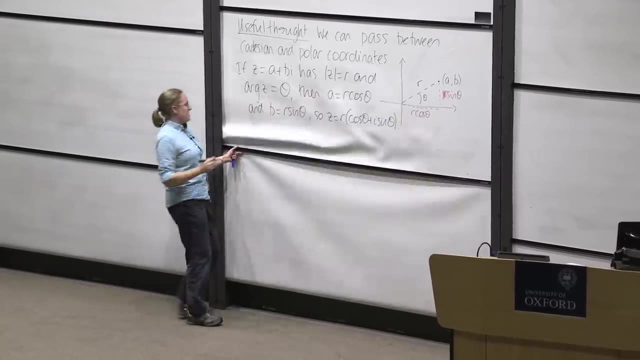 b is r sine theta. So one kind of way of thinking about z, then, is to think of it as being r times, cos theta plus i sine theta, which is a representation that we find coming up in various contexts. In the other direction, if z is a plus, 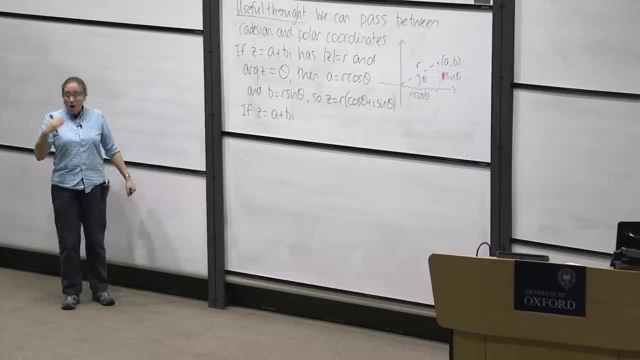 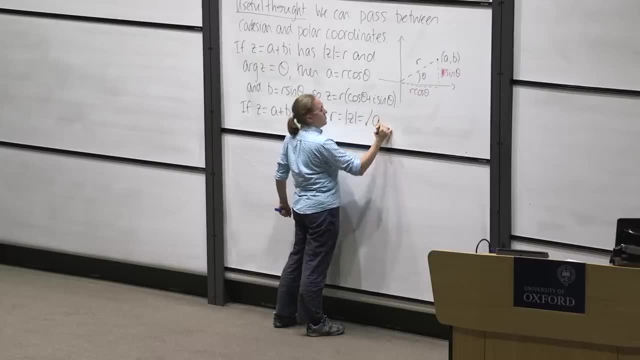 b, i and I want to find r and theta. well, we know how to find r just by the definition. So r is the modulus of z. It's just the square root of a squared plus b squared. That's how we defined it. 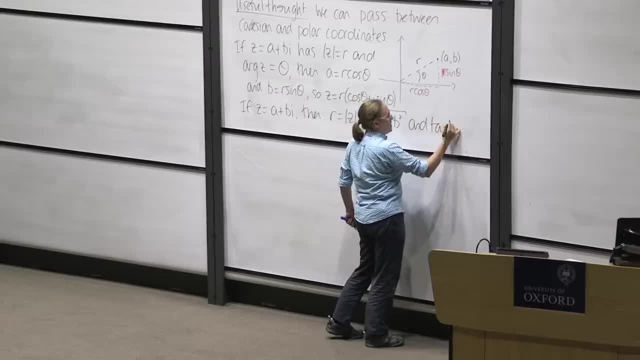 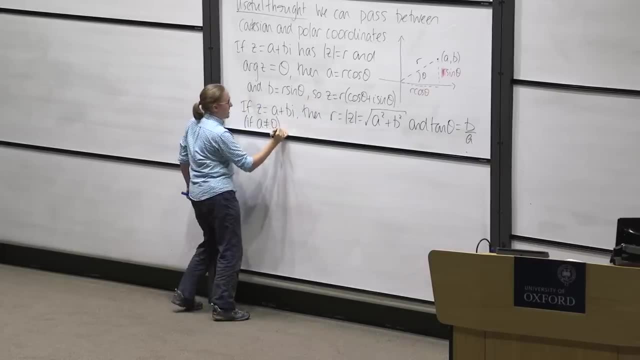 And also again looking at the diagram tan, theta is b over a, At least in the case when a is not zero. I'm very scared about the possibility of dividing by zero. I don't want to risk it, But as long as a is not zero, 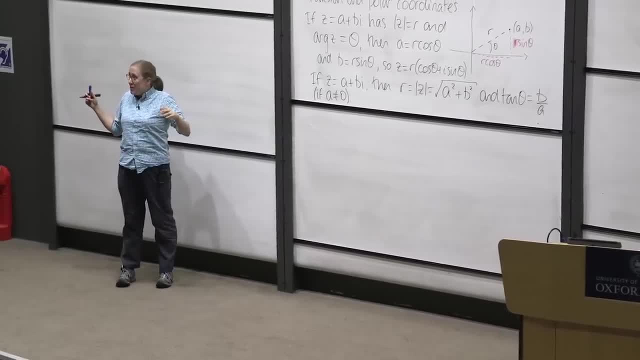 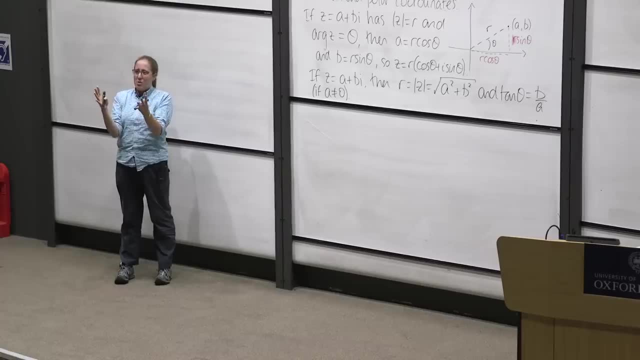 then b over a is going to give me tan theta And from that I can kind of recover theta. but as we know, there's this sort of ambiguity about what theta is, because if you have some argument, theta, well theta plus 2 pi or theta plus any integer multiple of 2. 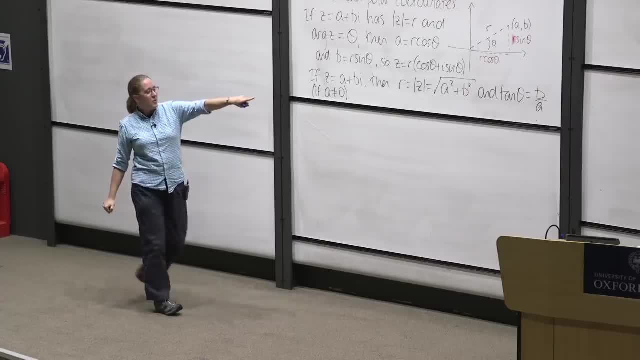 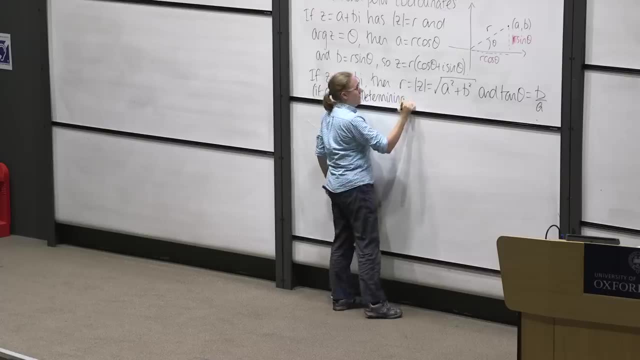 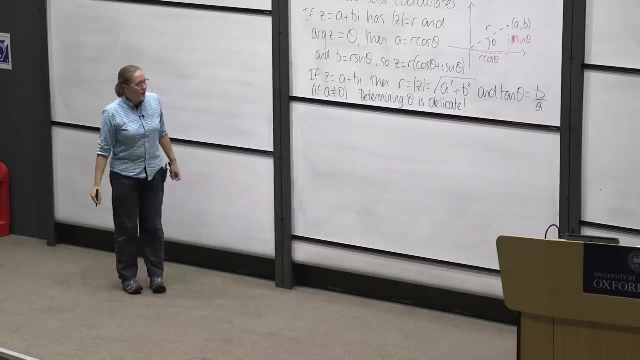 pi will also be a valid thing, And that's reflected in the fact that there's not a kind of unique inverse here. So I'll just put: determining theta is delicate, So in practice this is not a problem. you just need to have your wits about you a little bit. 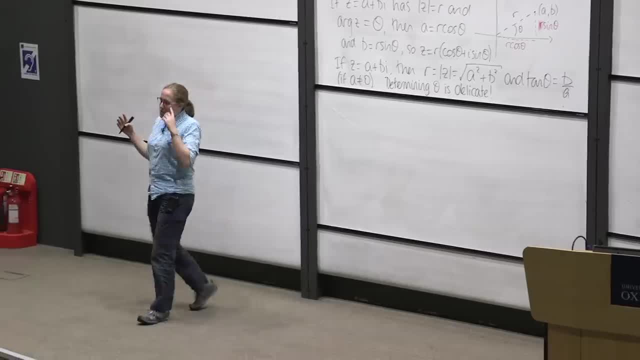 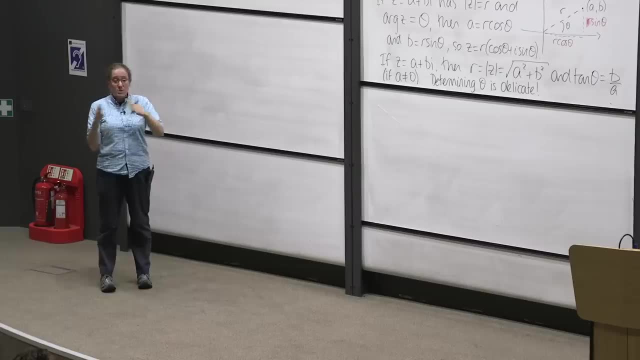 So I want to know what happens when we multiply. We saw that we could interpret addition of complex numbers geometrically with that kind of vector addition parallelogram diagram. What happens with multiplication? Well, we know what happens to the modulus when we multiply. That behaves nicely. 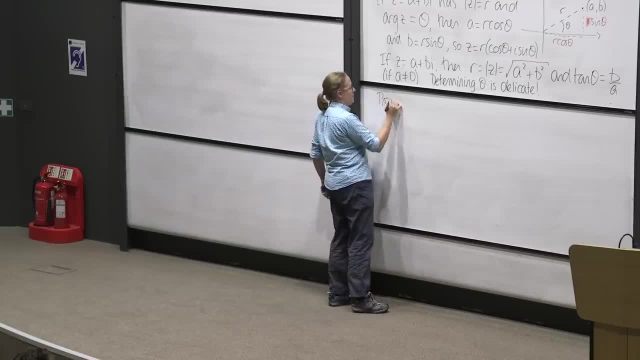 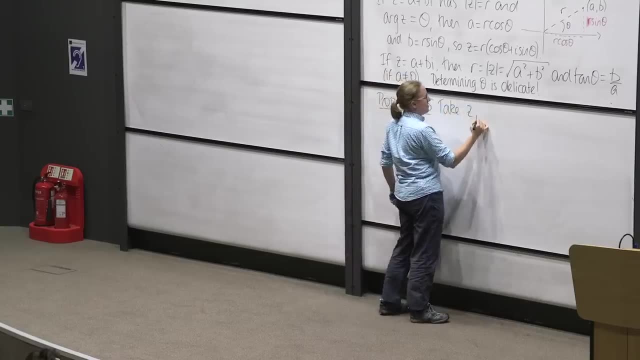 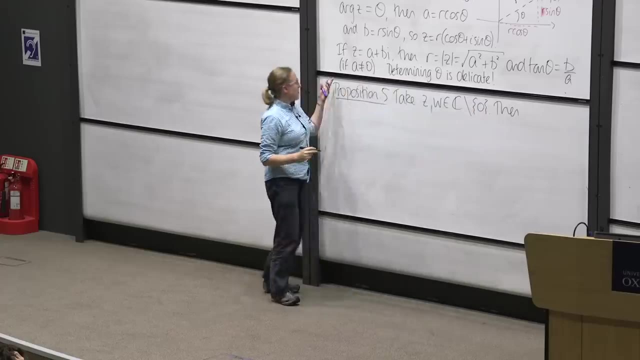 What happens with the argument? So this is proposition 5 and this says: take z and w in the complex numbers, but not zero then. so remember, the argument of zero isn't defined, so I want to ignore that. The argument of z times w is equal. 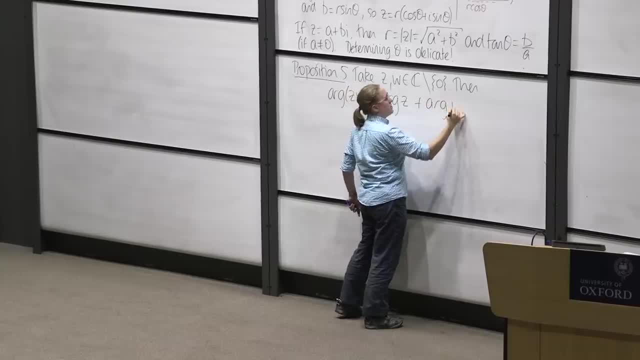 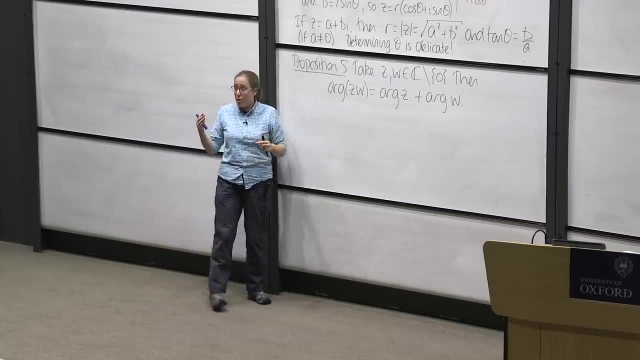 to the argument of z plus the argument of w. So a couple of little comments here. One is that here we're working with arguments modulo 2, pi, So this idea that these two are equal up to some multiple integer, multiple of 2. 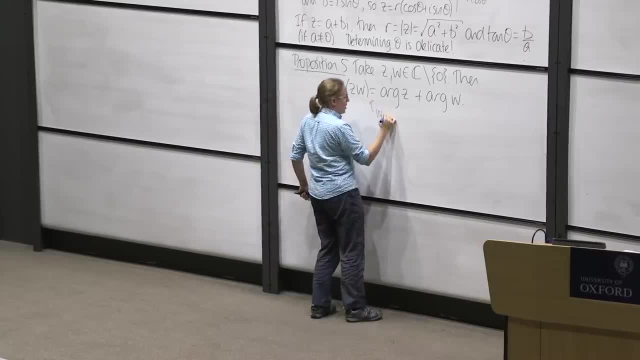 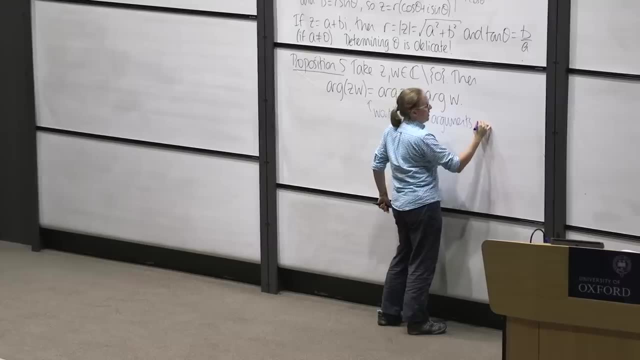 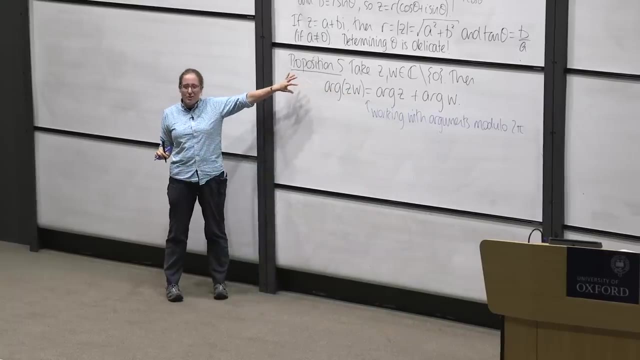 pi. So it's important that we remember that. So this is working with arguments modulo 2 pi. The other is that you've seen this kind of relationship before. This looks a bit like a logarithm. right, That's not a coincidence. There are no coincidences. 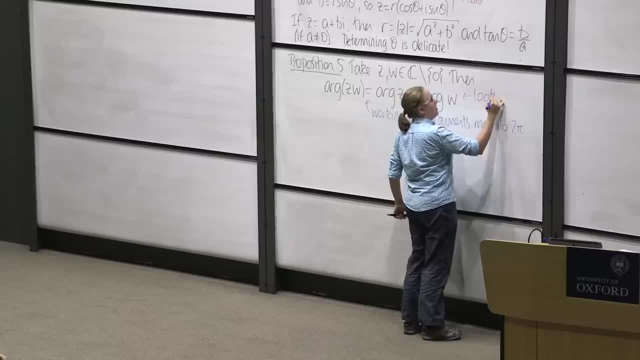 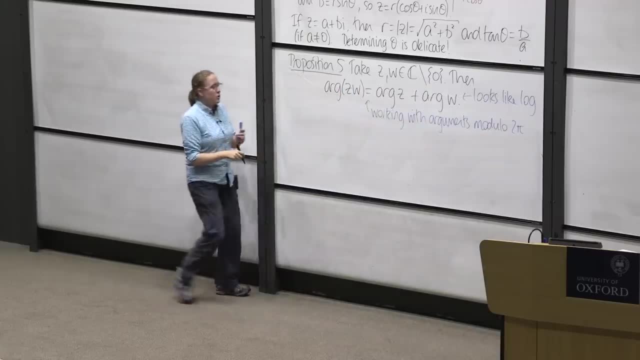 in mathematics. So maybe I'll just note here: this looks a bit like log. Looks like log That's very pleasingly alliterative, So let's think about how we're going to prove this. So this is not too bad actually, given this. 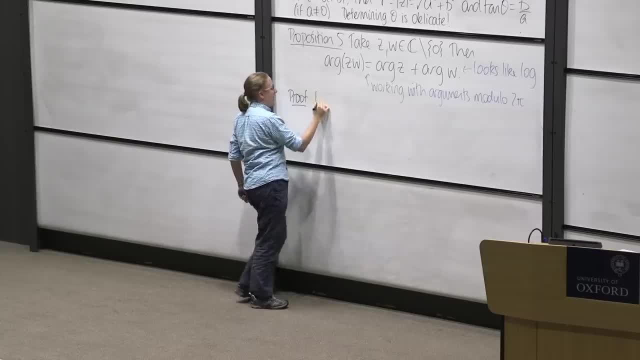 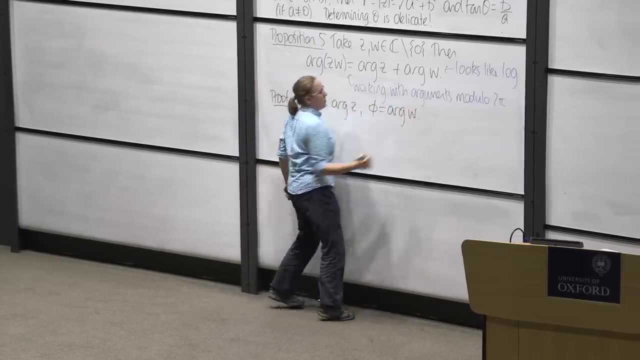 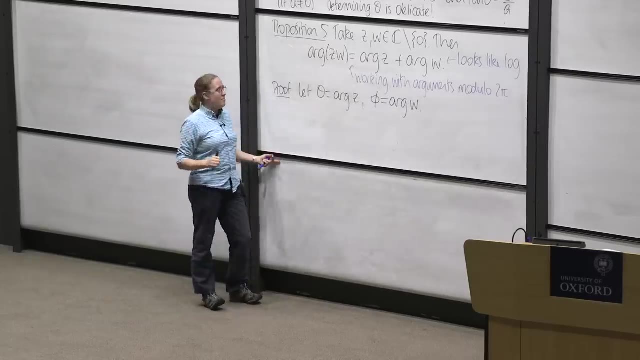 kind of thinking that we've been doing up here. So if I let theta be the argument of z and phi be the argument of w, I hope you're making good progress with learning the Greek alphabet. It's not fantastic with every Greek letter, but theta and phi are really good. 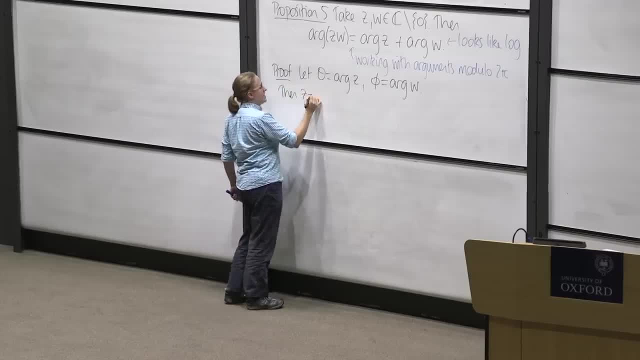 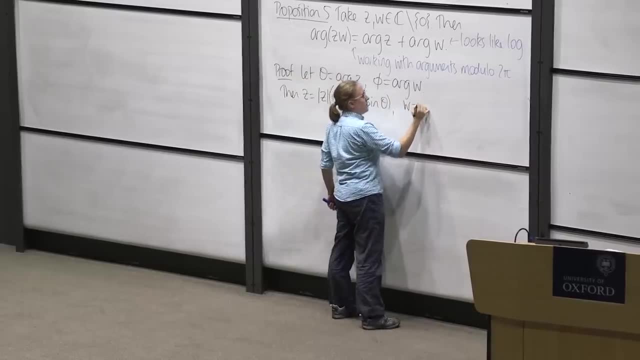 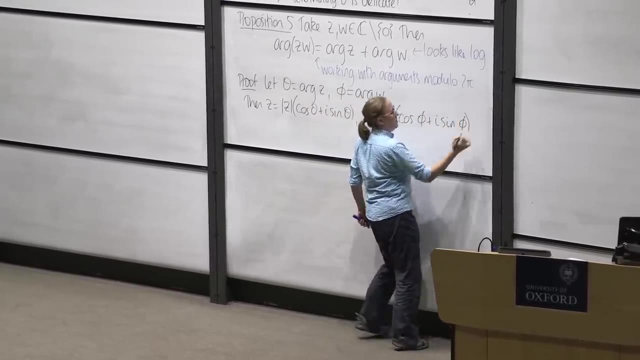 Greek letters to know. So then, what we've just said is that z is going to be the modulus of z times cos theta plus i sine theta, and w is going to be the modulus of w times cos phi plus i sine phi. So we can just multiply. 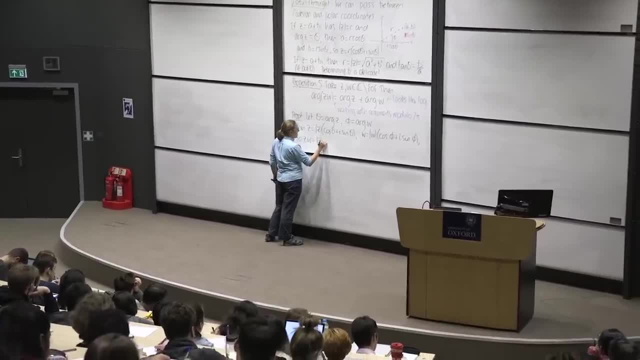 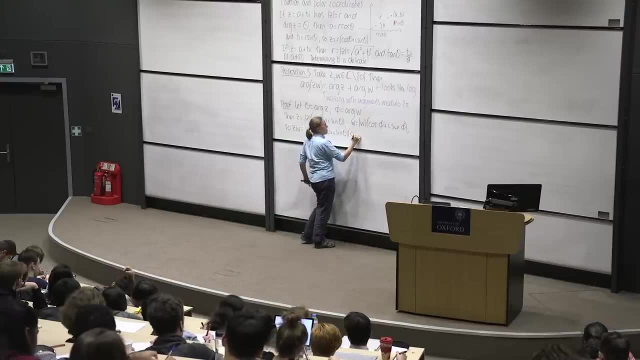 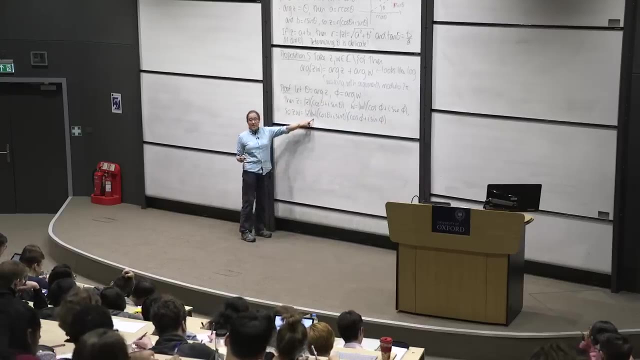 So z w is the modulus of z times, the modulus of w times cos theta plus i sine theta, times cos phi plus i sine phi, And I can do some tidying up here. So one thing is that I know what happens with this multiplication for the modulus. So that's the modulus. 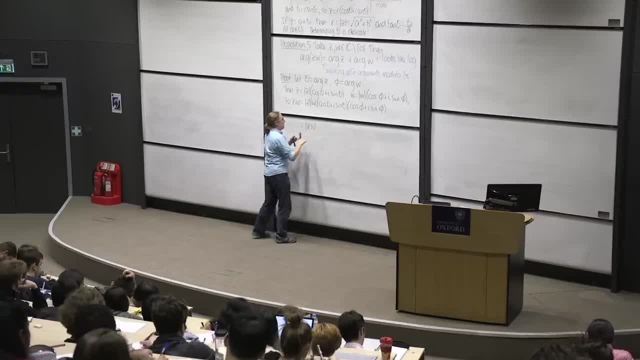 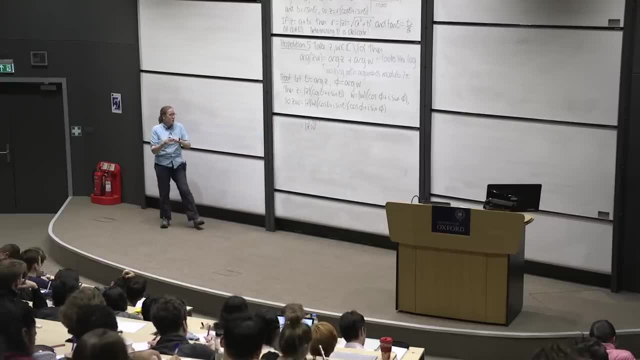 of z w. I'll write it that way round And I guess we're using proposition 3 here. I'm not going to record every time we use proposition 3 for the rest of all time, because it's just going to come up so much. But 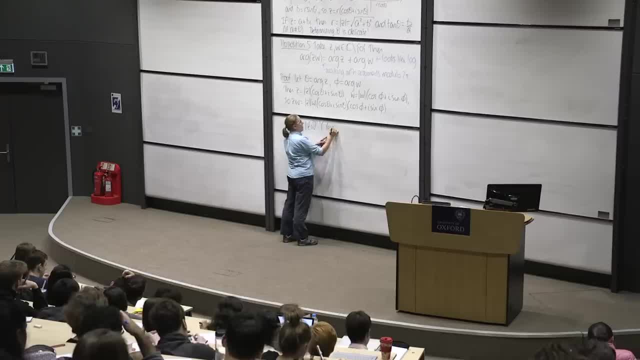 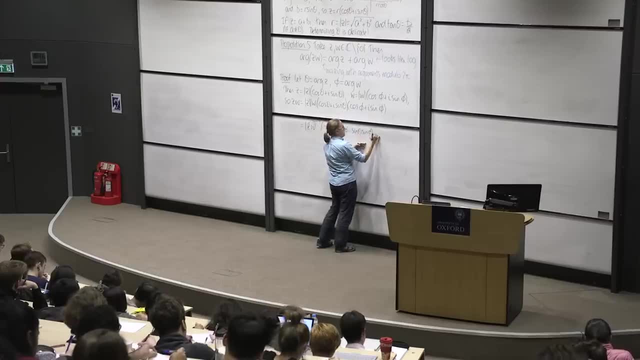 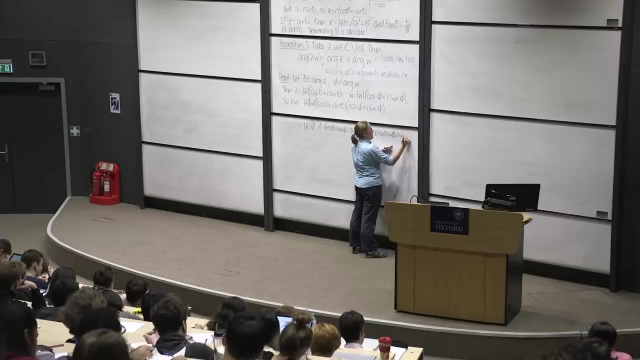 I'll just note it here to remind you, And if I multiply out here, I get cos theta cos phi, minus sine theta sine phi. that's coming from these terms plus i times cos theta sine phi, plus sine theta cos phi, And hopefully you might recognize these from your. 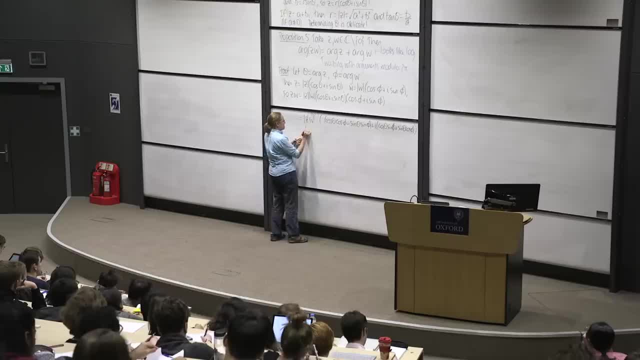 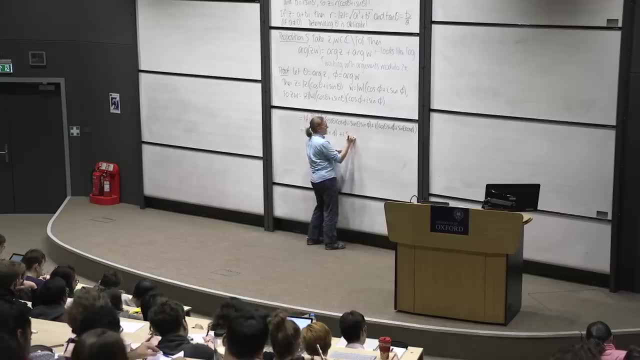 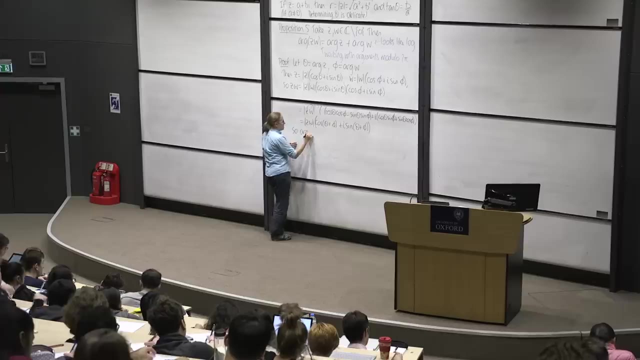 kind of compound angle formulae in trig. So this is the modulus of z w times cos of theta plus phi plus i times theta plus phi, And so we can read off immediately that the argument of z? w is theta plus phi, which is the argument of z. 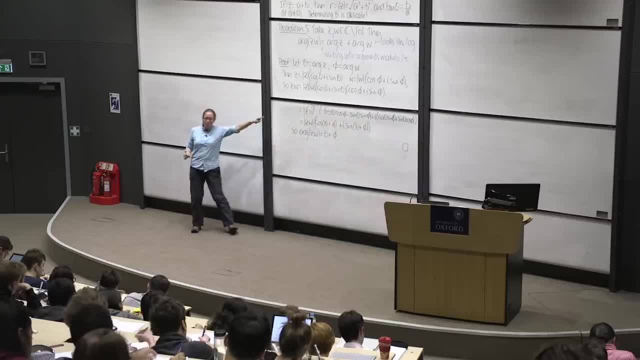 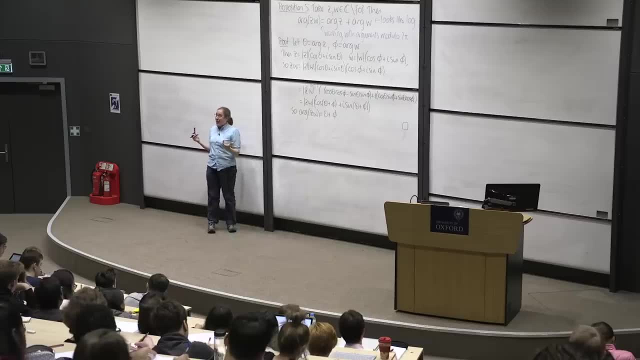 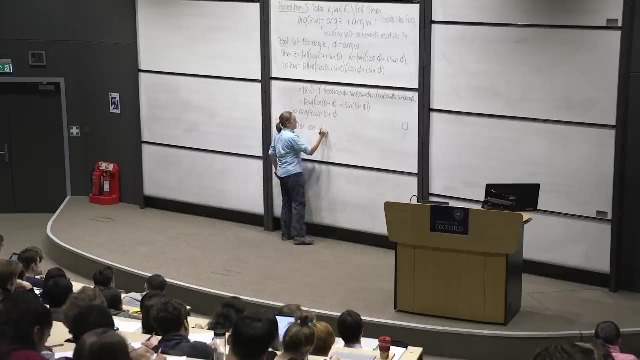 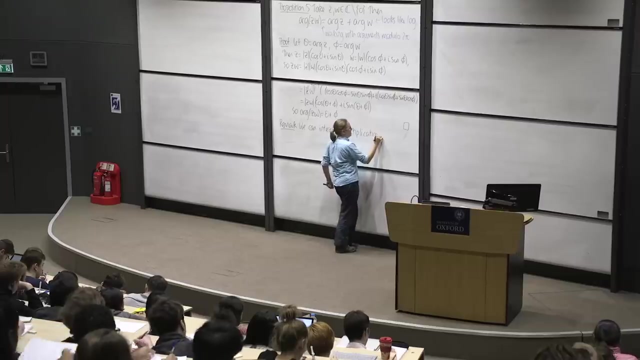 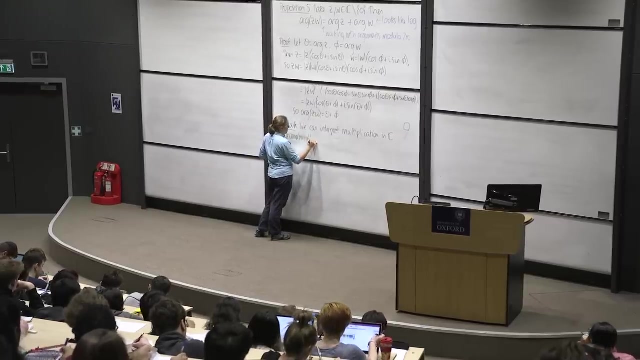 plus the argument of w. Of course, it's not a coincidence that the trick here works out nicely, right? So we can use this to make sense of multiplication in a geometric way. So, remark, we can interpret multiplication in c geometrically, So multiplying. 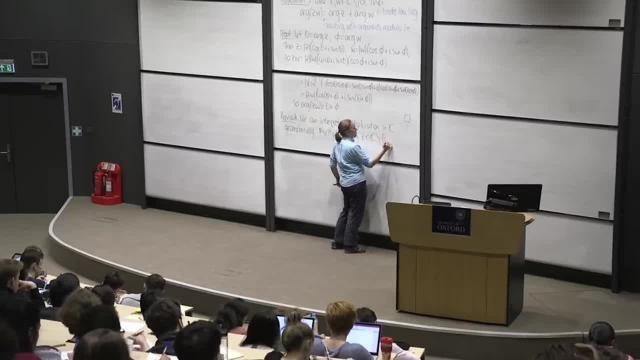 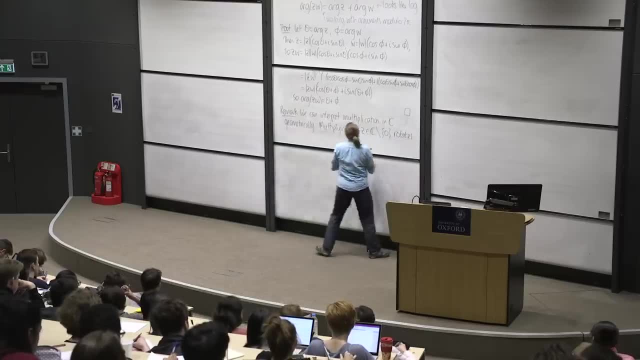 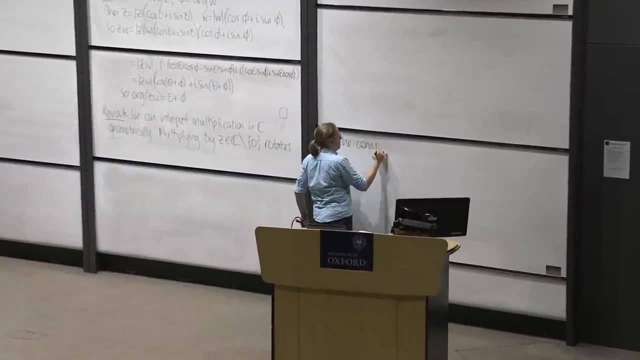 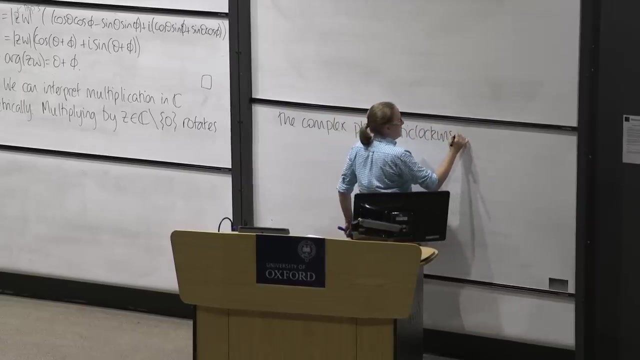 by a non-zero complex number, z. Multiplying by zero is not so exciting. Multiplying by some non-zero complex number, z. That rotates the complex plane. I'll move over here Anti-clockwise by the argument of z. This is a consequence of that proposition. 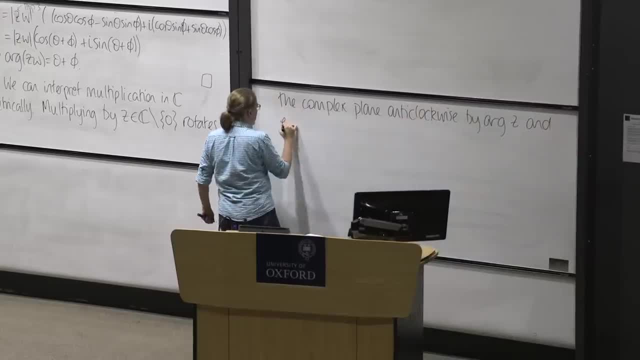 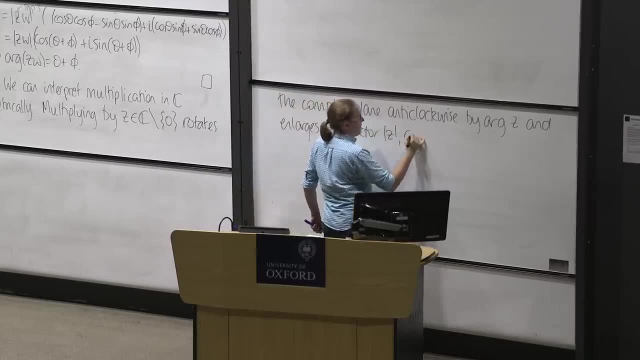 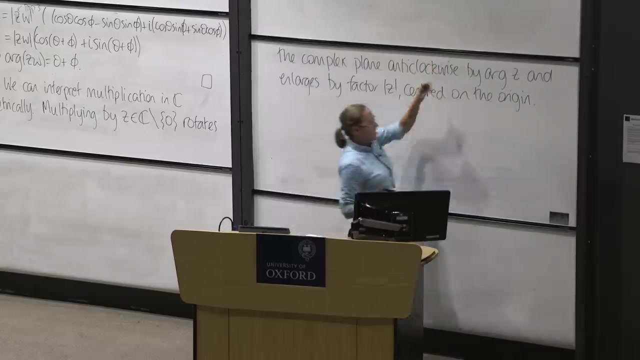 we just proved, And it enlarges by a factor, the modulus of z, And that's all centred on the origin. So there is a nice way to make sense of multiplication with our geometric view of complex numbers as well as algebraically. So we're going to find ourselves using this. 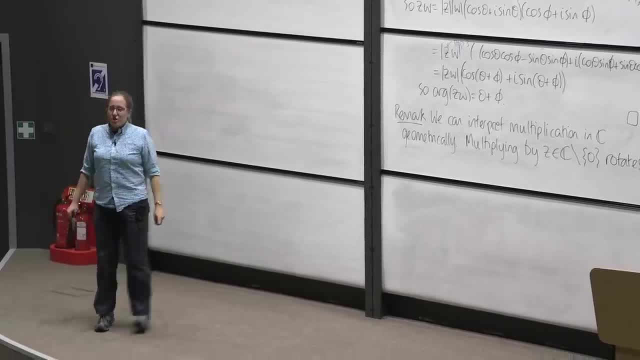 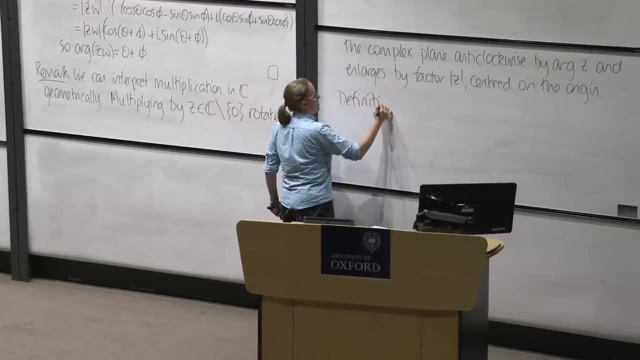 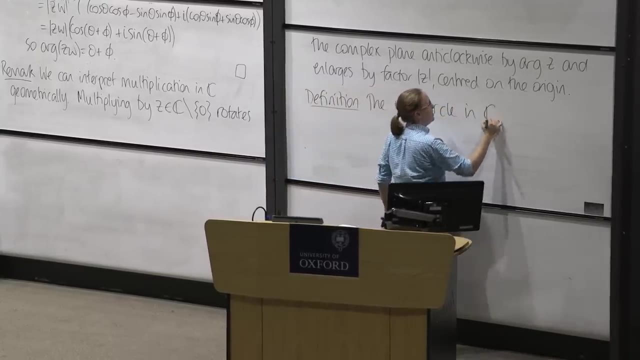 proposition lots. Okay, I want to introduce you to some particularly nice, complex numbers. They're called the unit circle. So definition: The unit circle. In c I'm defining unit circle. It's kind of what you'd expect. But I'm also telling you this because I want 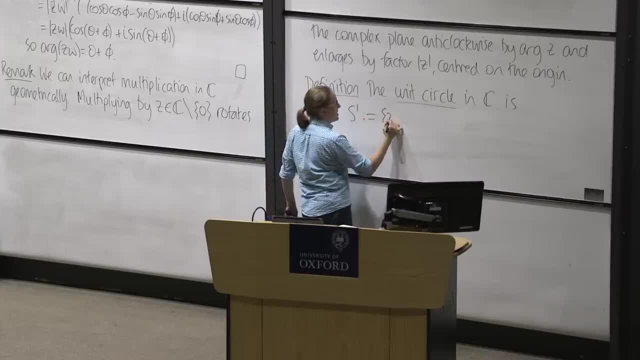 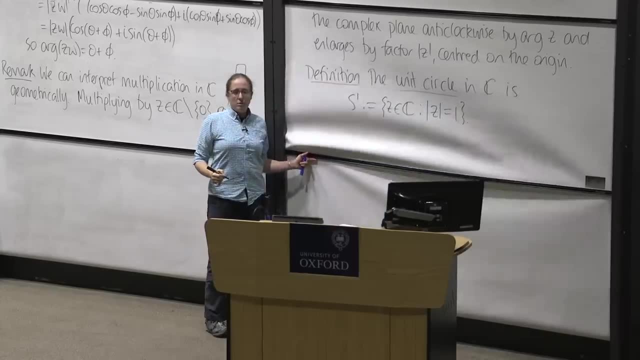 to tell you that it gets called s1. And s1 is defined to be the set of all z in c, such that the modulus of z is equal to one. So, geometrically, it's a circle of radius, one centred on the origin. 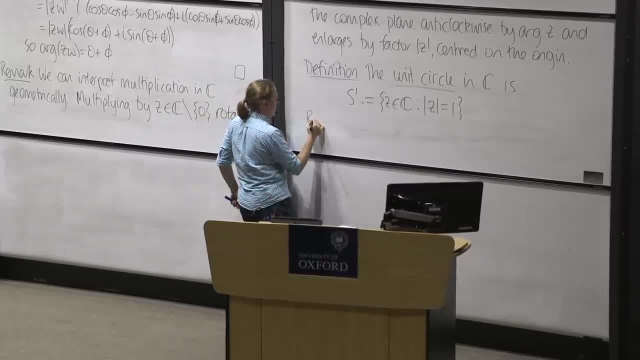 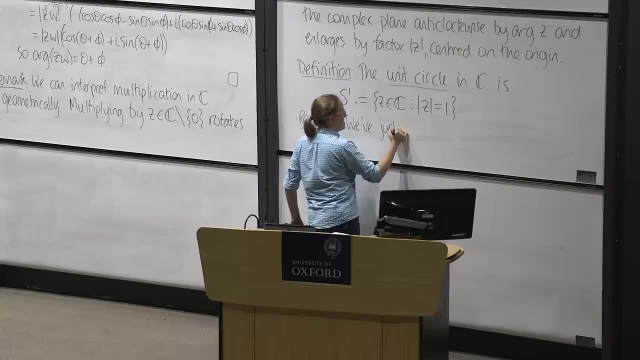 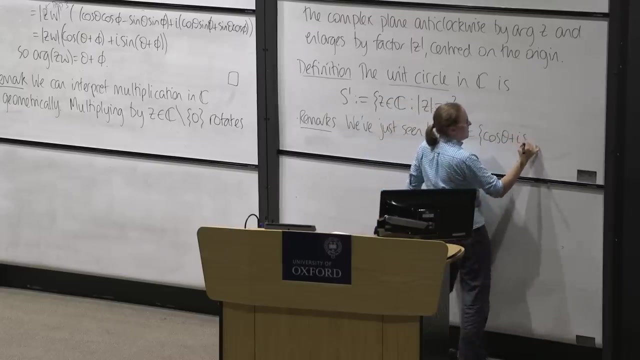 And what we've just noticed is that we can write that in another way. So here are a few little remarks about the unit circle. So we've just seen, essentially, that s1 is also the set of all cos theta plus i sine theta, where theta is real. 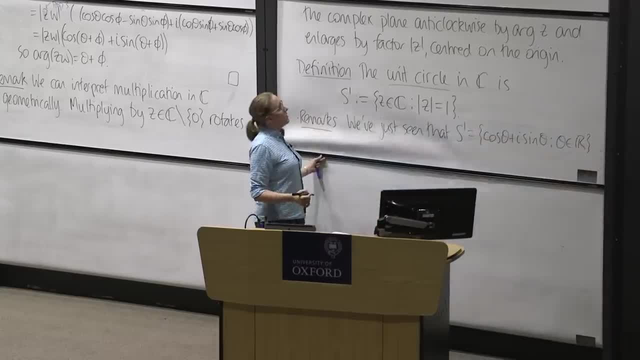 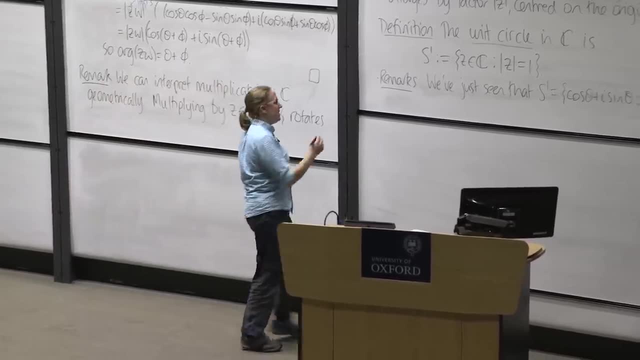 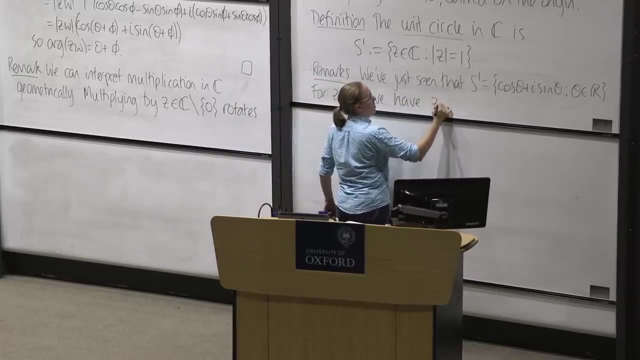 So that would be another way of thinking about it. Here is an amusing and really surprisingly useful fact about numbers in the unit circle. So if I take z in s1, what is the inverse of z? Well, we know that z times z bar is the modulus. 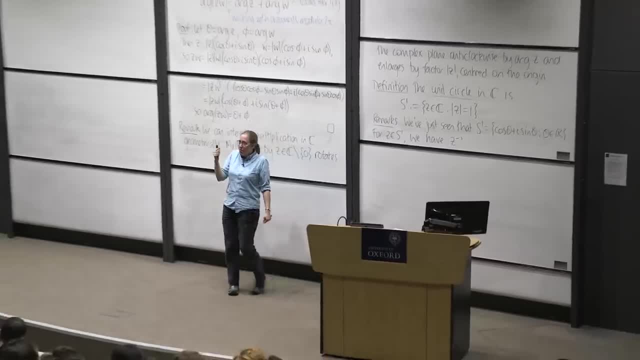 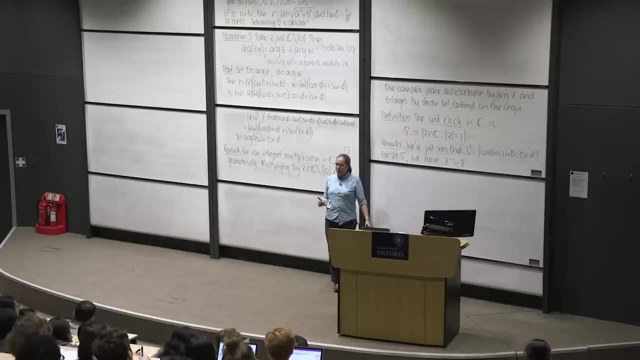 of z squared. If you're in the unit circle, the modulus of z squared is one, So z times z bar is one in this case, So the inverse of z is its complex conjugate Cute Also useful, And this is also going to. 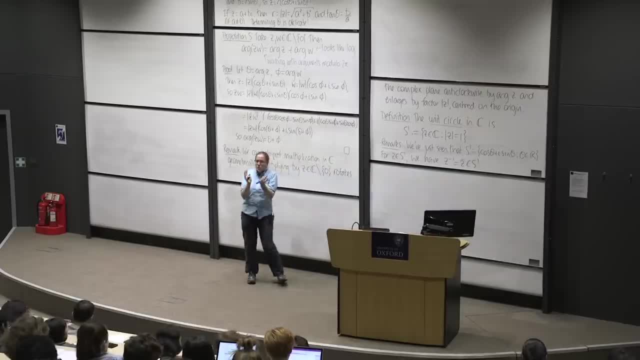 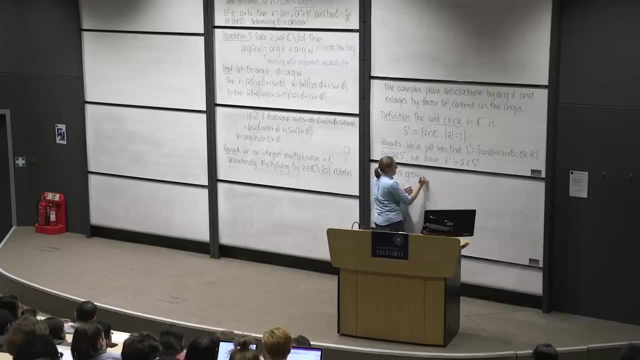 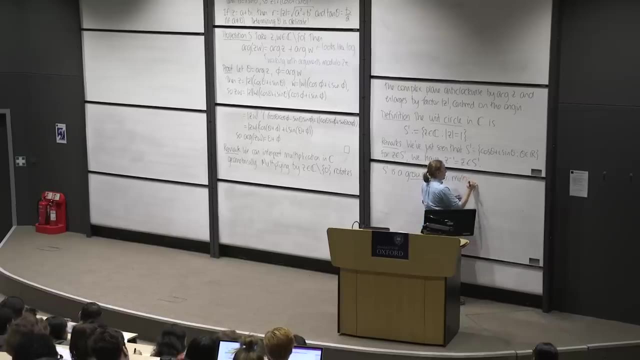 lie in the unit circle. So the unit circle has all sorts of nice structure within itself And in fact s1 is a group under multiplication. This is not the time to tell you what a group is. There's a course on that. It's called groups. 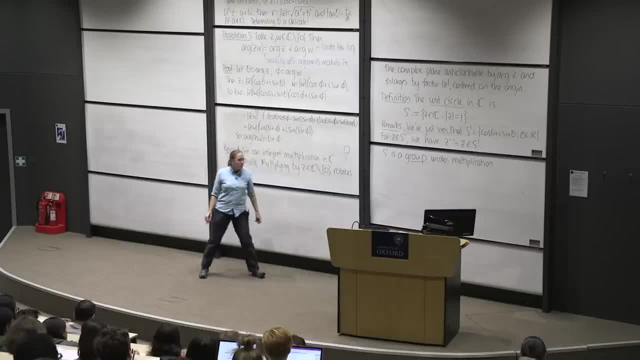 So in February some person will introduce you to groups in the course on groups and group actions and you'll meet at s1 as an example. So this thing about the inverse is relevant. There are some other things that go into that. The thing to remember here is: 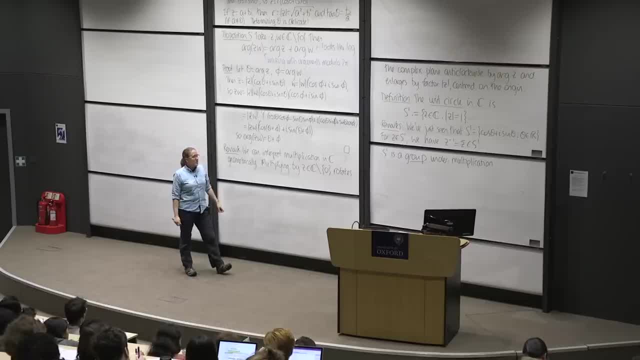 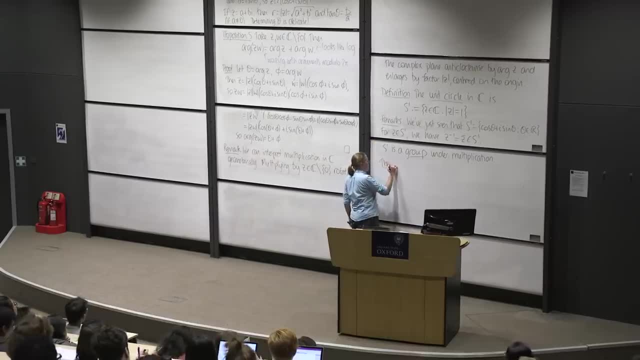 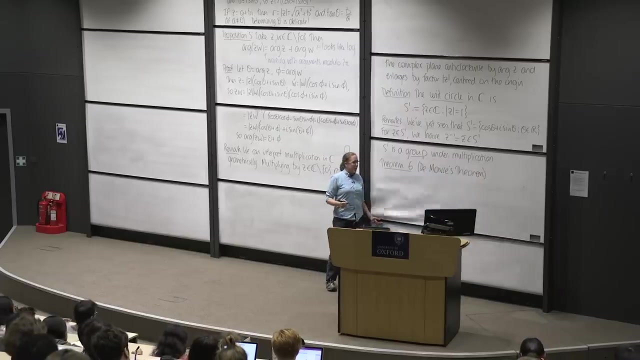 the unit circle is a kind of important and interesting object. It has kind of structure. So here is a really super exciting result about numbers in the unit circle. This is a theorem and it's called de Moivre's theorem And this is going to be, I imagine, familiar to. 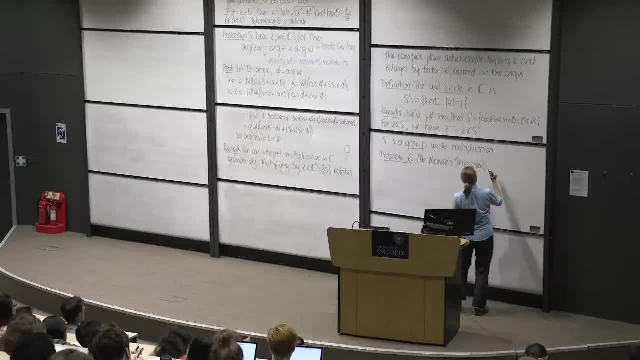 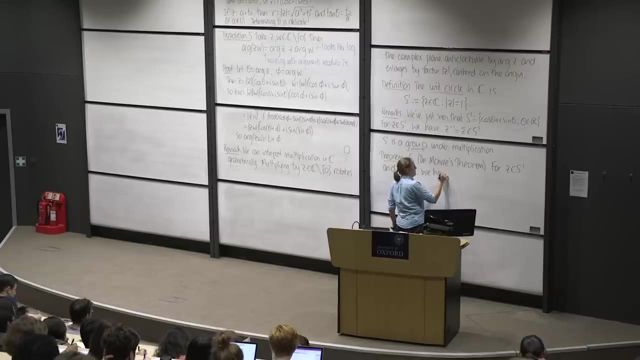 quite a few of you, But I might not be phrasing it necessarily in the way that you're used to. So for z in the unit circle and any integer n, remember this- just means n is any integer. we have that, the argument of z to the n. 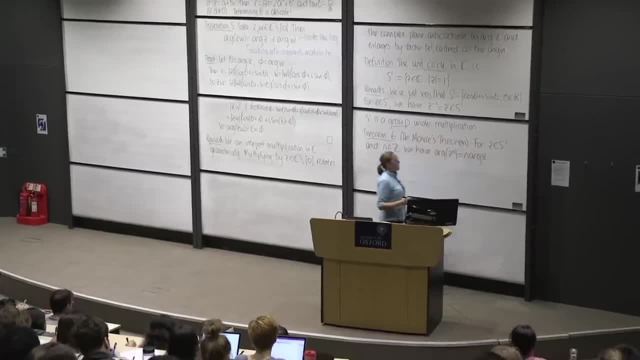 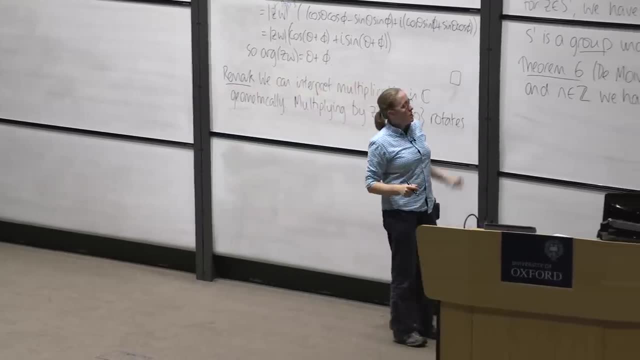 is n times the argument of z. So this proposition is a very special kind of. it's kind of related to this. We're going to be using this proposition to feed into it, But this is kind of helpful So you might be more familiar with the equivalent. 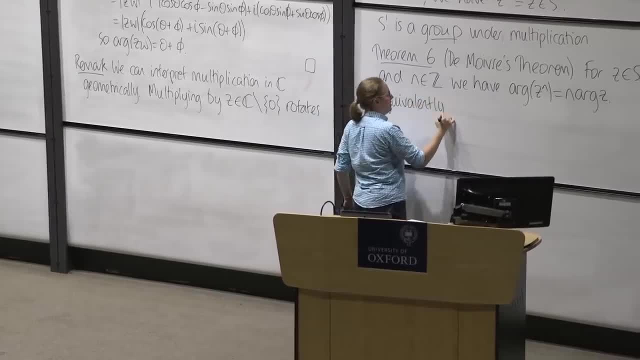 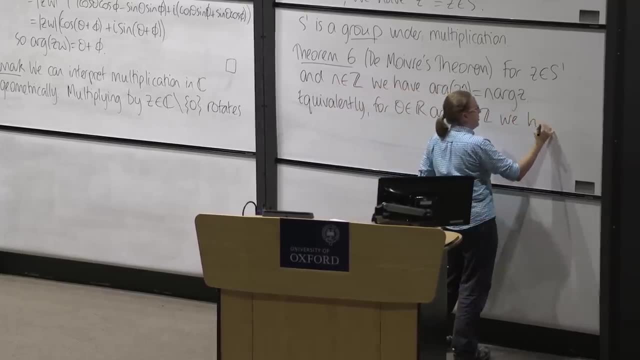 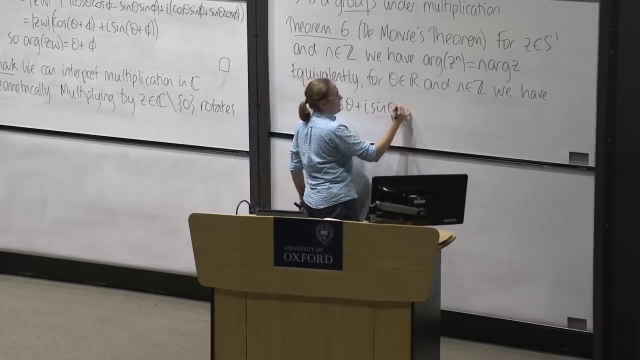 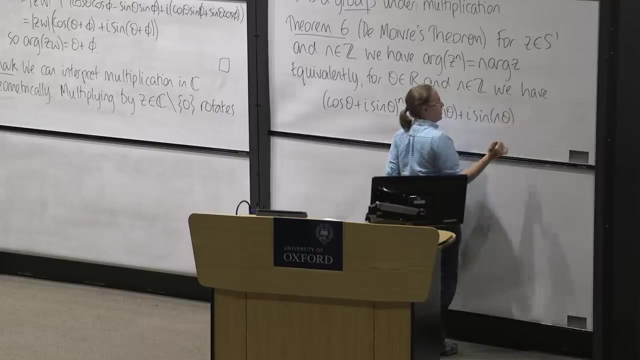 formulation: Equivalently for theta in r and n in z, we have that cos theta plus i sine theta to the power n is cos of n theta plus i sine of n theta. So definitely, when I first learnt about de Moivre's theorem, I learnt about it in this form. 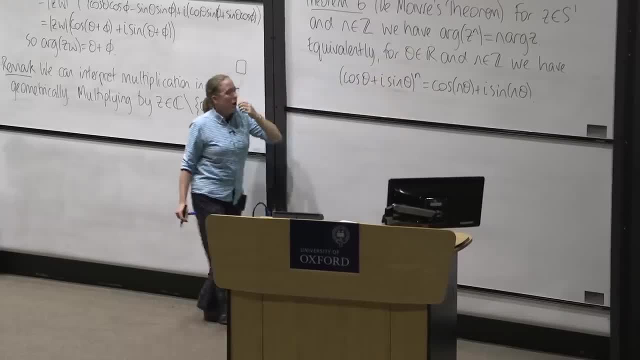 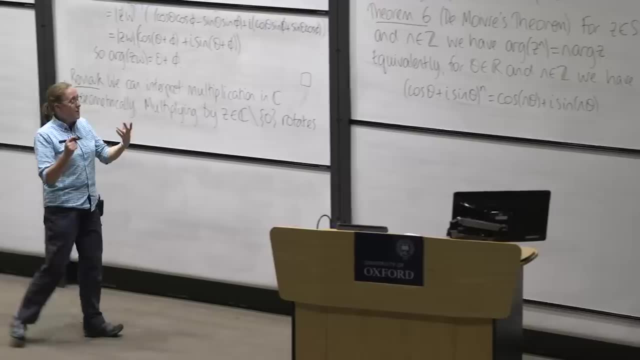 But this form is a really helpful way of thinking about it. So I encourage you to think about why these are saying the same thing, Because if you understand why they're saying the same thing, that's a really good way, kind of sign that you are understanding. 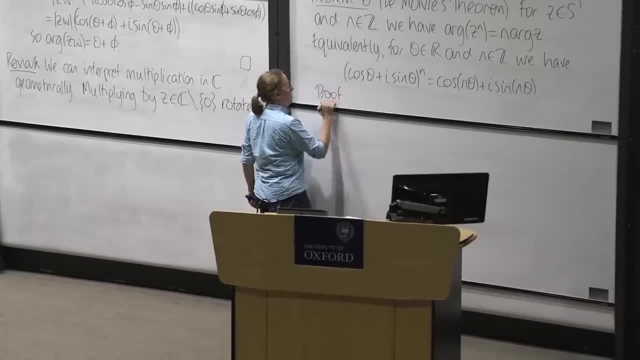 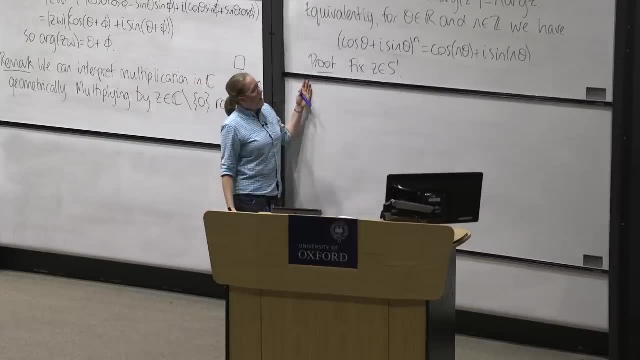 the theorem. So let's prove this. So I'm going to fix some z in s1 and show that the theorem applies to this z And for n greater than or equal to 0, so for non-negative n I'm going to use induction on n. 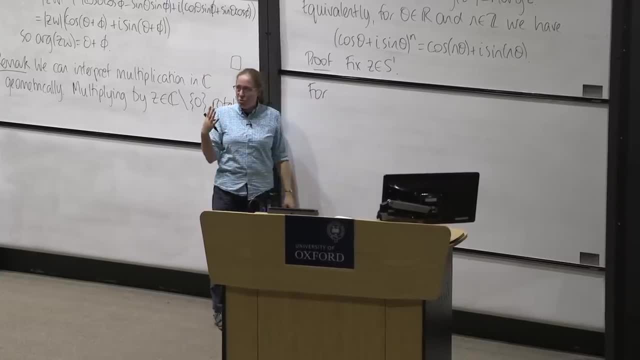 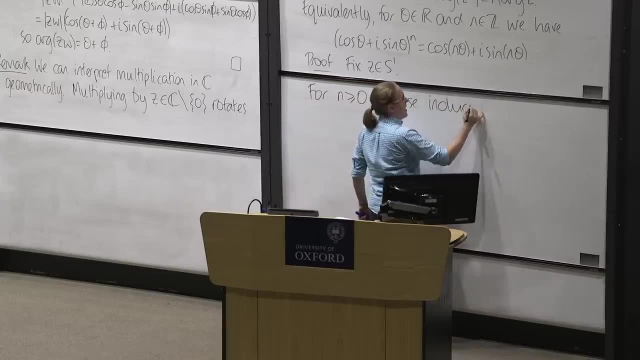 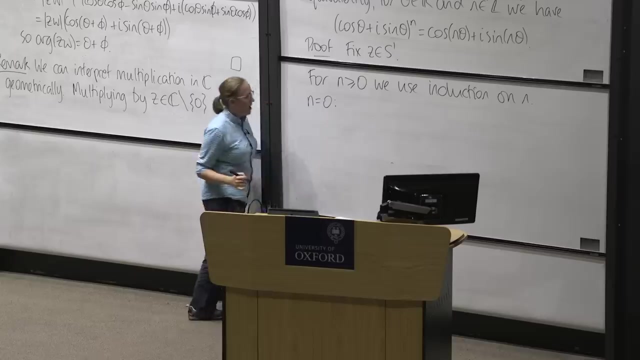 And I'm going to write that down because it helps the reader to know that we're going to use induction. So for n greater than or equal to 0, we use induction on n. So my base case is n is 0 and that's. 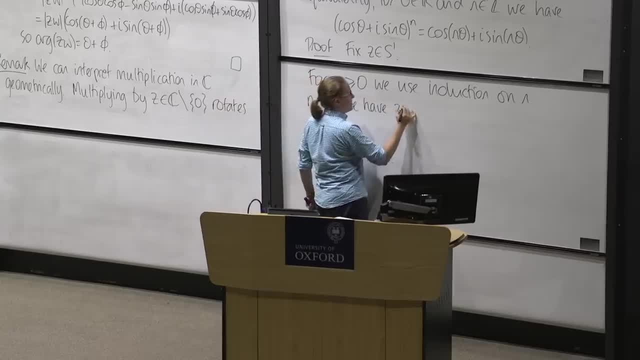 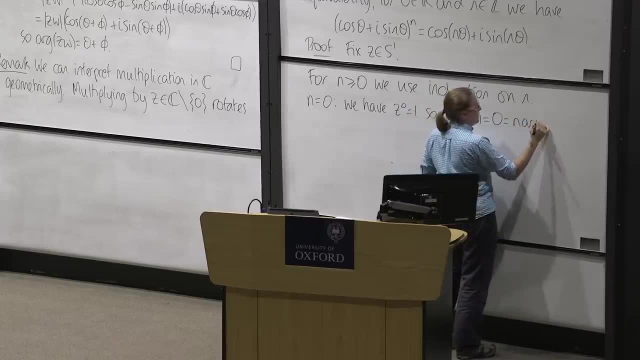 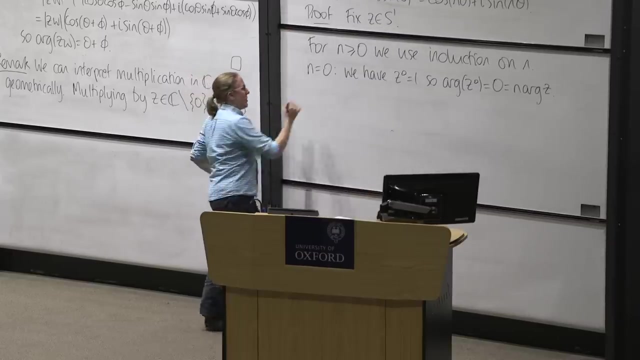 just a quick check. So z to the 0 is equal to 1.. So the argument of z to the 0 is 0 is n times the argument of z in this case. So that was important, although not super exciting. More interestingly, let's think about the inductive 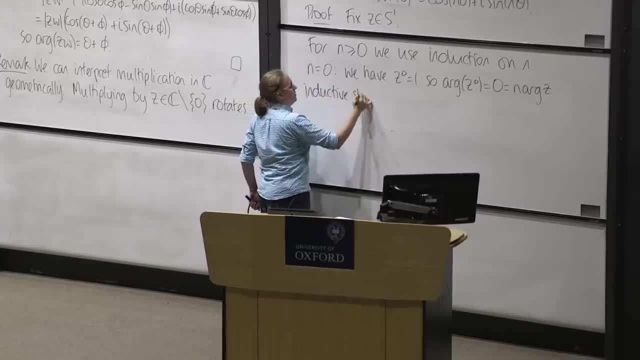 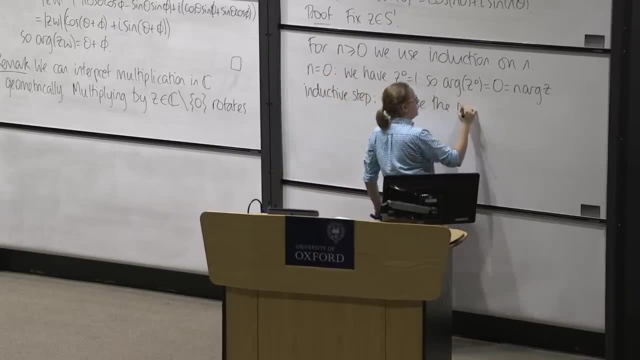 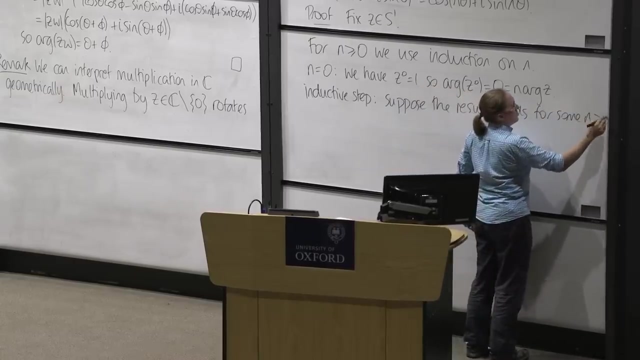 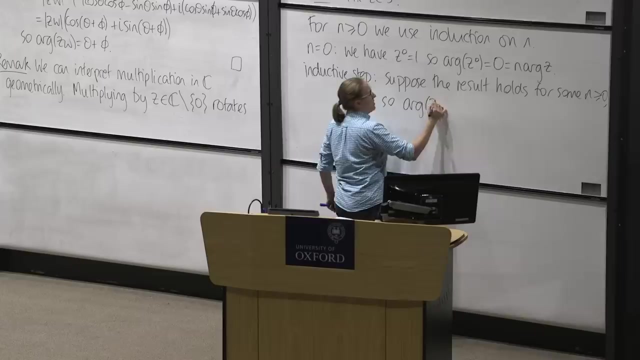 step. So let's suppose the result holds for some n greater than or equal to 0.. So we've got some fixed value of n where we're supposing it holds. So we're saying that the argument of z to the n is equal to n times the 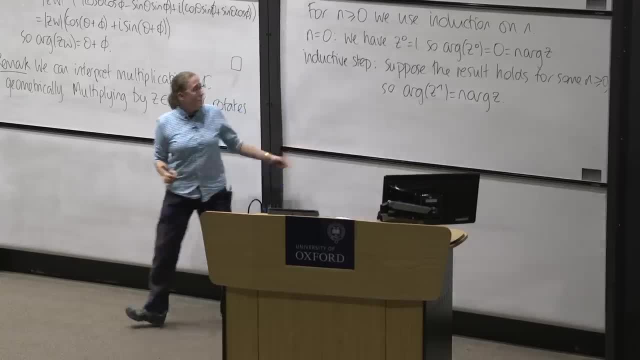 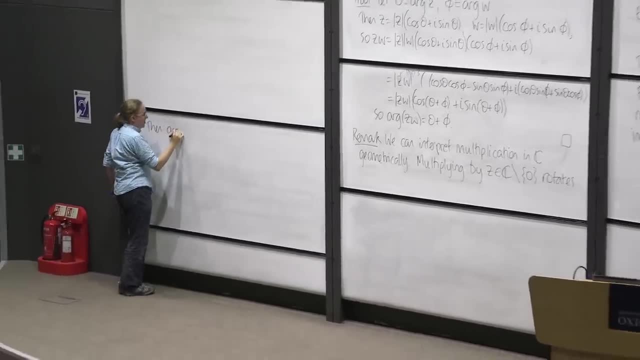 argument of z. And now we want to think about the argument of z to the n plus 1.. So let's do that over here. So then, the argument of z to the n plus 1.. I want to relate to the argument of z, but I can. 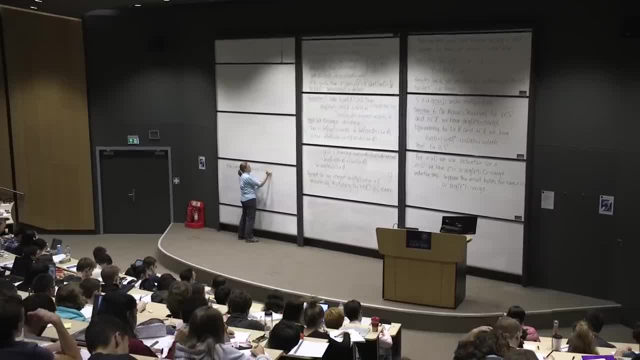 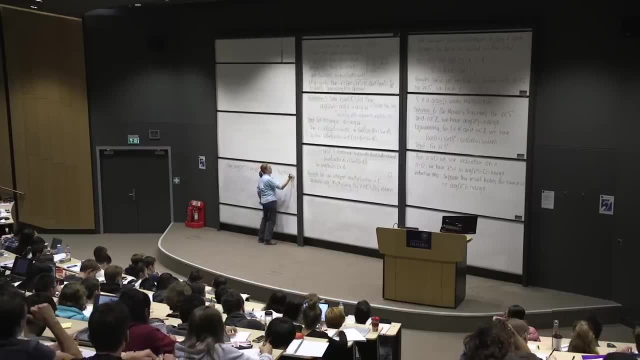 do that using proposition 5, which tells us that that's the argument of z to the n plus the argument of z. So I'll write down that's by proposition 5.. And then we know about the argument of z to the n, because that was our. 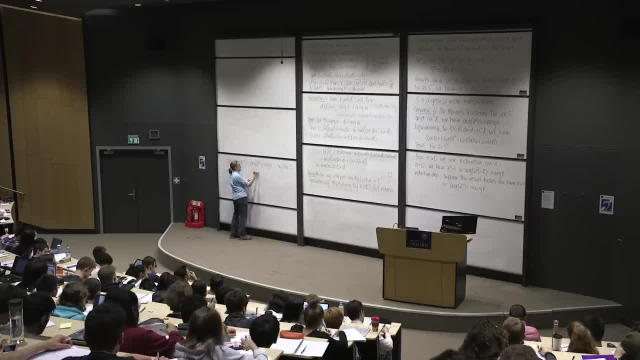 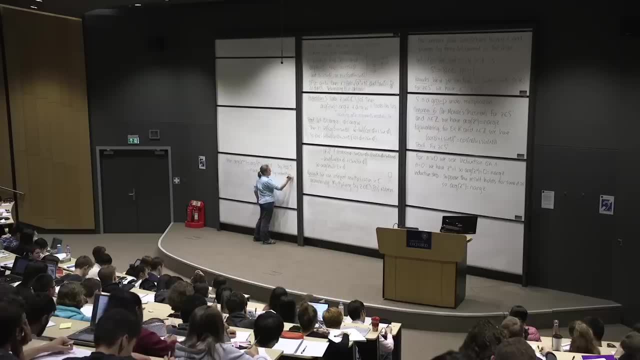 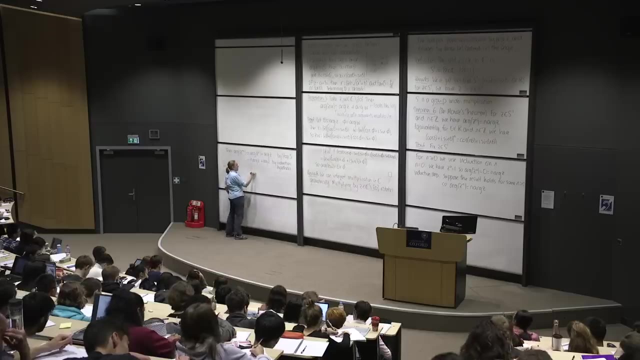 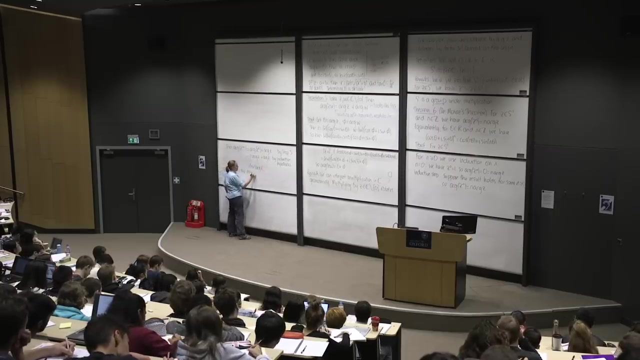 induction hypothesis. So this is n times the argument of z plus the argument of z by the induction hypothesis, And that's equal to, of course, n plus 1 times the argument of z. So we've shown that the result holds for n. 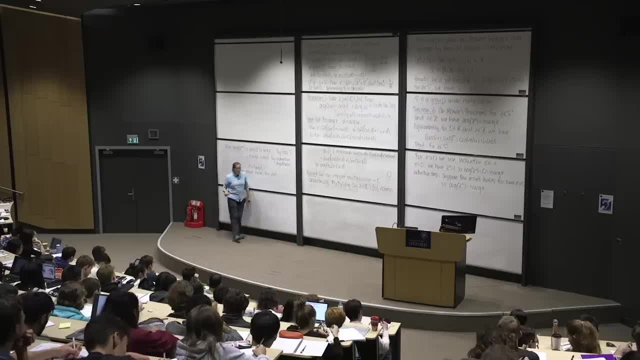 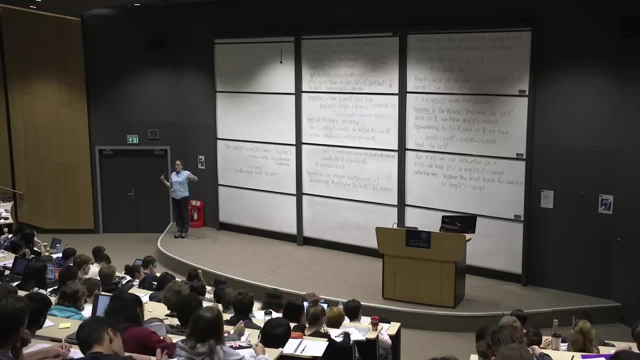 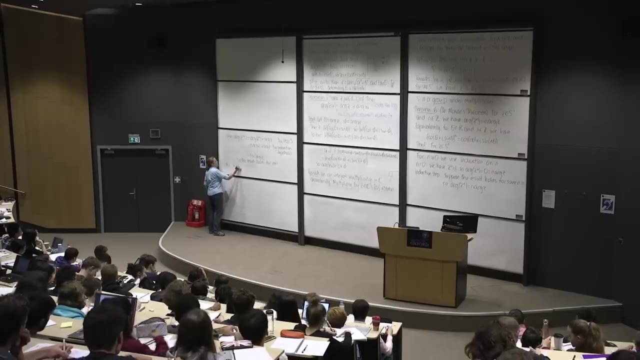 plus 1.. So that's an inductive proof that shows us that this relationship works for n greater than or equal to 0.. Now I want to think about negative n, And one possibility would try to be to do a kind of induction downwards. That could be a useful 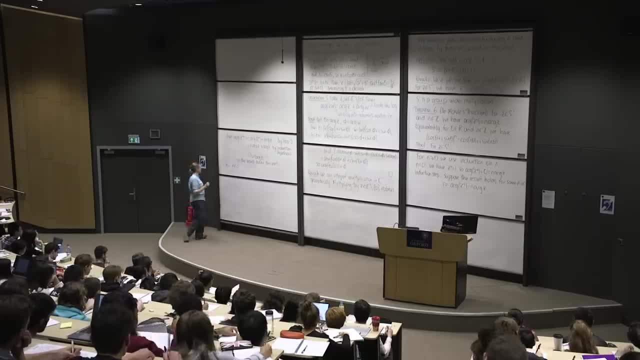 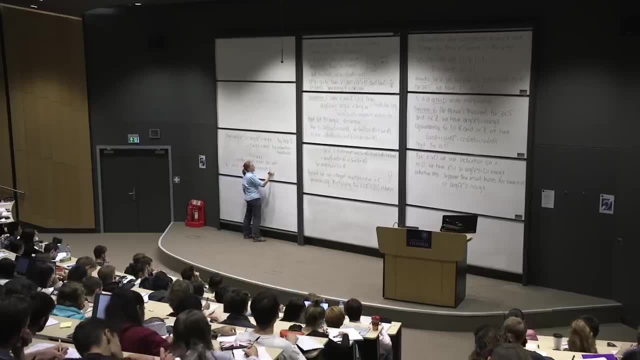 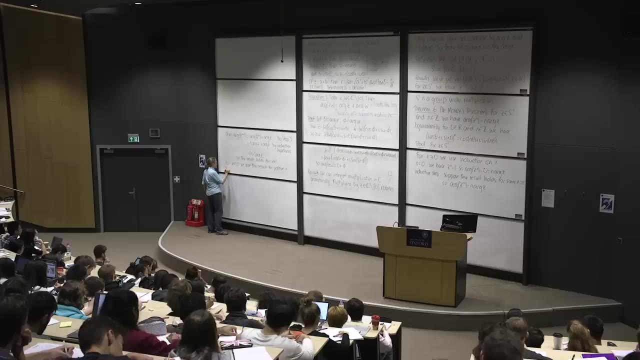 strategy. But actually I think we can just use the result for positive values. So for n less than 0 we use the result for positive n. So this can be a nice strategy to use work you've already done to save yourself a bit of effort. So if I fix, 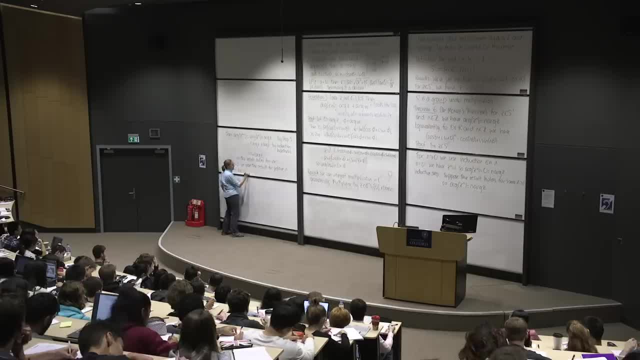 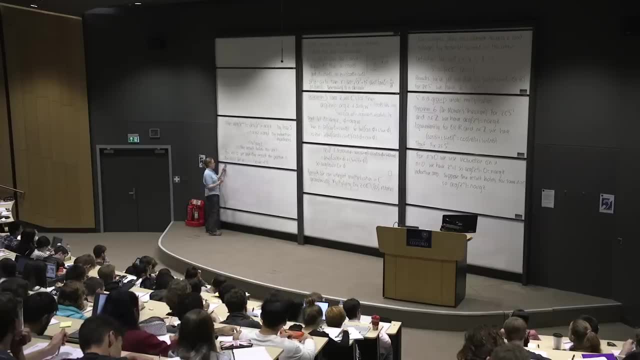 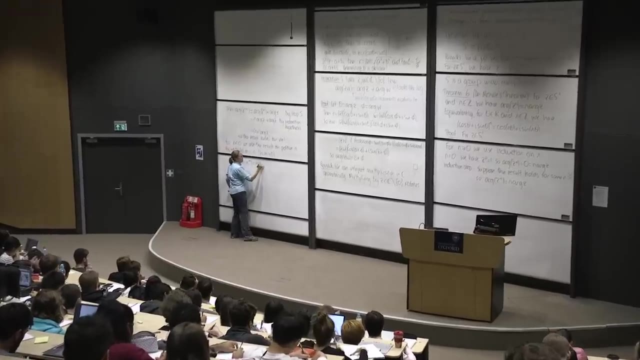 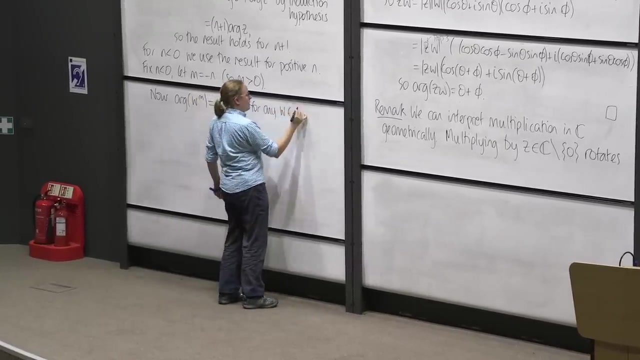 some negative n. I'm going to let m be minus n, So of course m is then positive. So by our previous result, so we know that the argument of w to the m is m times the argument of w for any w in s1.. 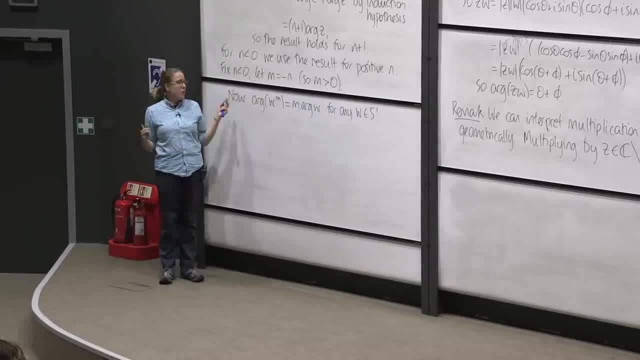 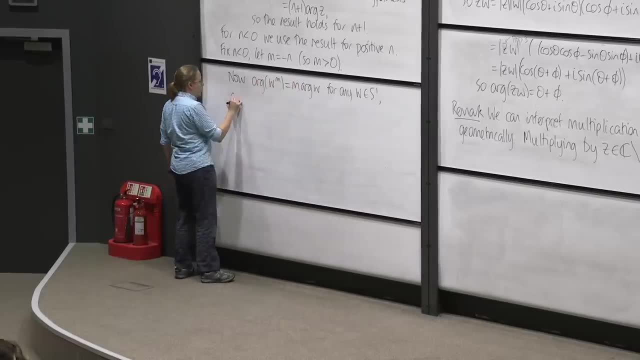 That's using the result for m, which is a positive value. So that follows from our previous part. So we just need to think about how we're going to apply this. Well, let's think about z to the n. z to the n is: 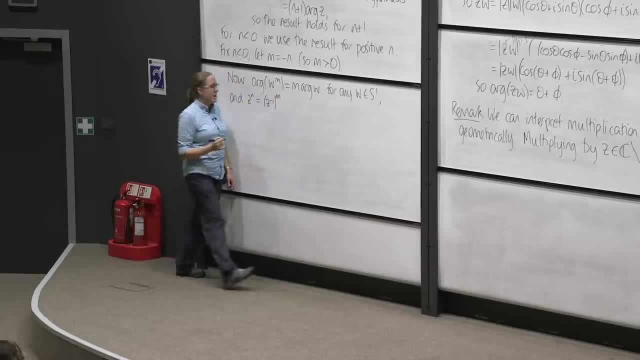 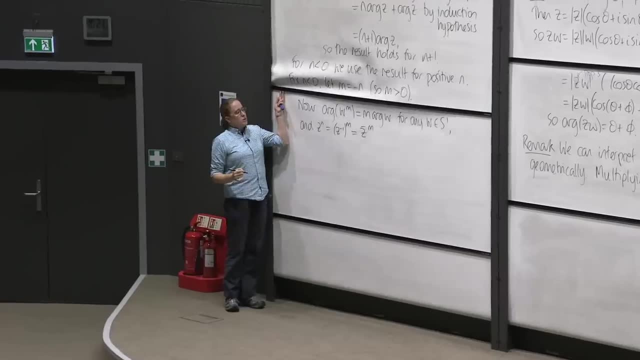 z inverse to the power m. That would be another way of rewriting it And z inverse. I noticed in my kind of fun facts over there was the complex conjugate of z, So we're going to be able to apply this result with w being the complex conjugate of z. 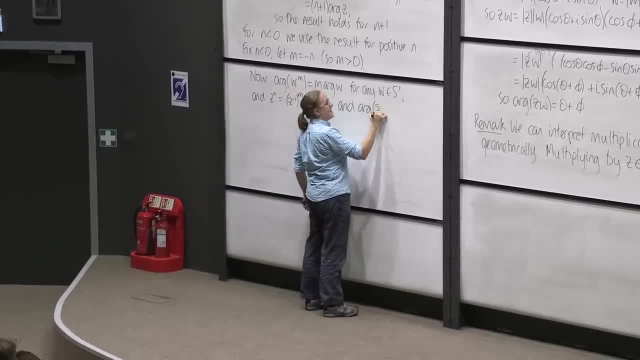 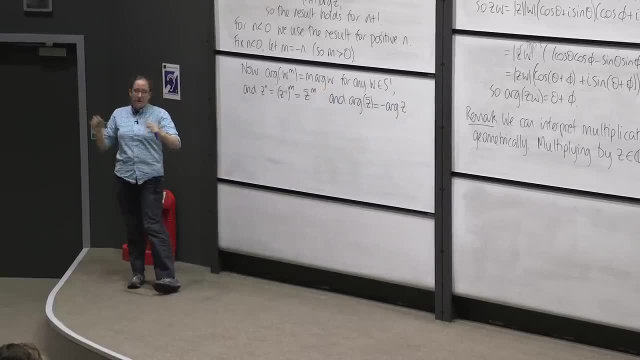 I'd quite like to know what the argument of the complex conjugate of z is. But if you ponder that for a moment, you'll see that it's minus the argument of z. Again, everything is modulo 2 pi here. So the argument of z to the. 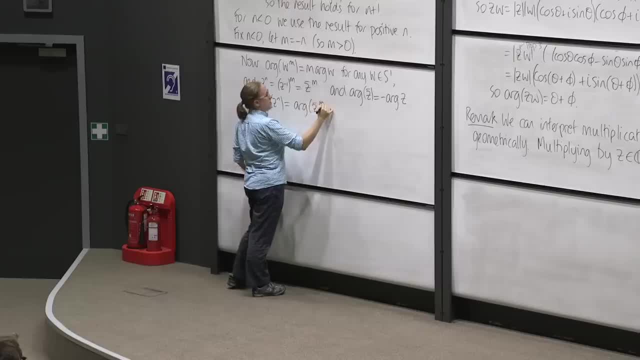 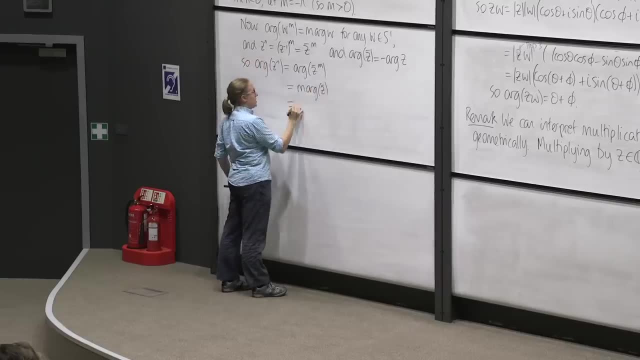 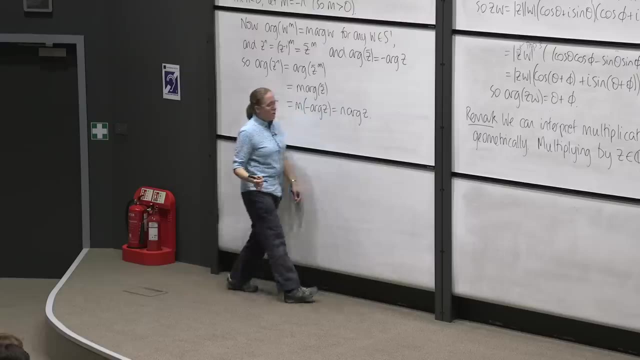 n is the argument of z bar to the m, which is m times the argument of z bar, which is m times minus the argument of z, which is n times the argument of z. So that proves the result for negative values, using the result for positive values. 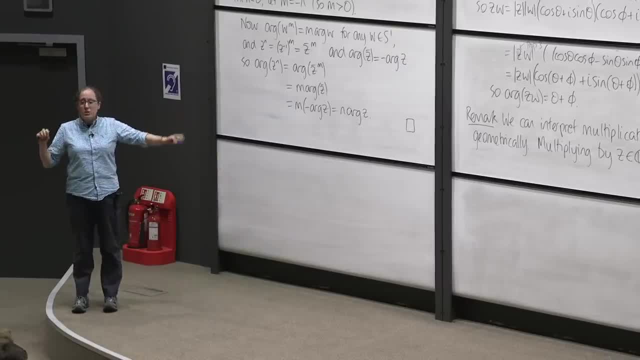 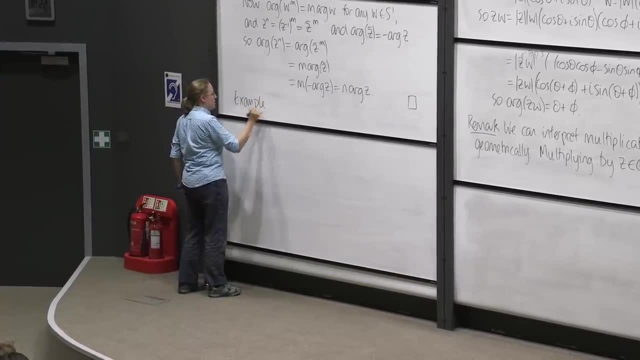 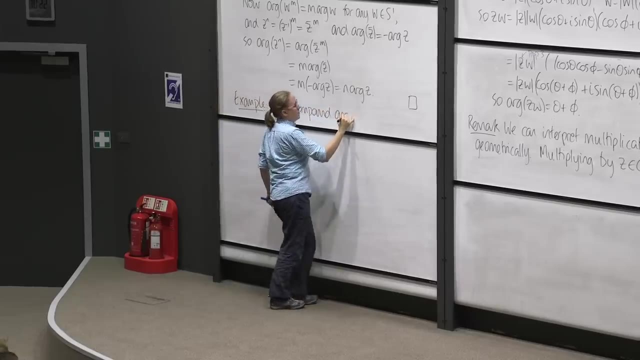 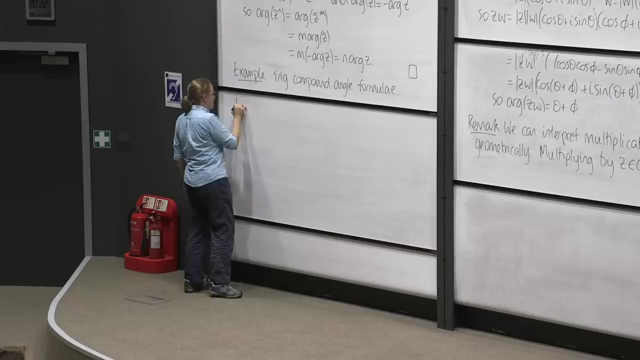 So De Moivre's theorem is just kind of somehow utterly fundamental and it gets used lots. Here is a specific example of a kind of classic way in which it gets used, Namely trig compound angle formulae. So by De Moivre for any theta. 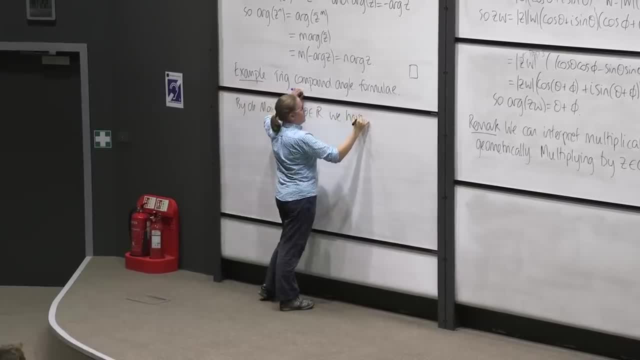 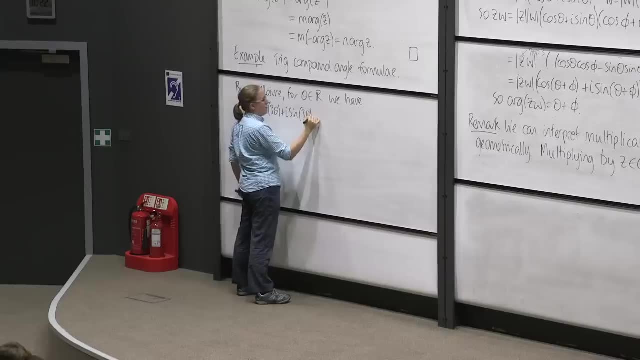 in R. we know that cos of 3 theta plus i sine of 3 theta is cos theta plus i sine theta cubed, That's from that kind of equivalent formulation. My goal here is to find some nice formula for cos of 3 theta. 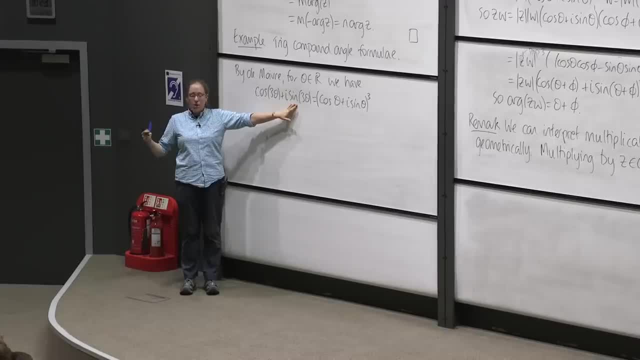 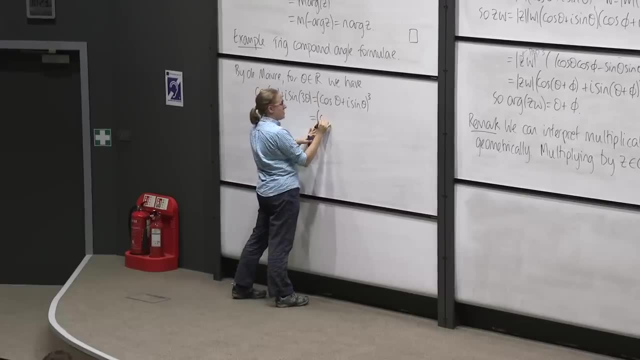 in terms of cos theta for sine, of 3 theta in terms of sine theta. So I'm going to expand this out. So this is a binomial theorem and kind of tidying up, and I think I'm going to get cos cubed theta. 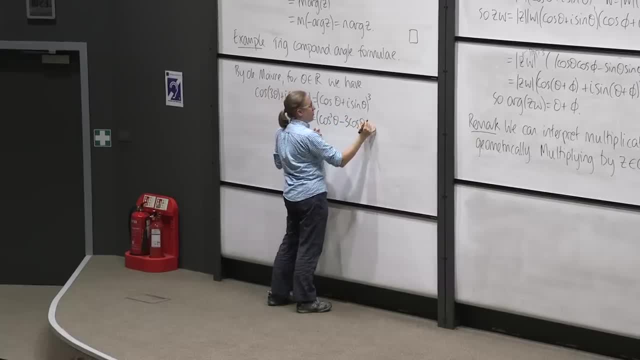 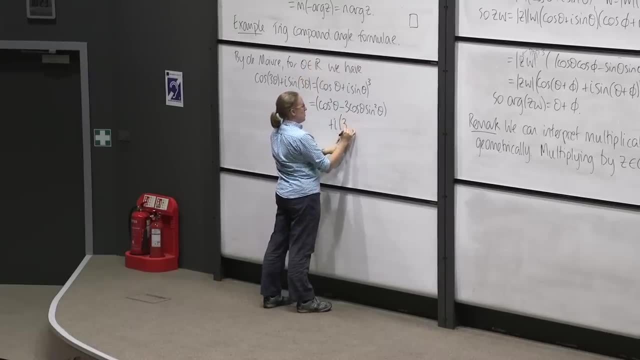 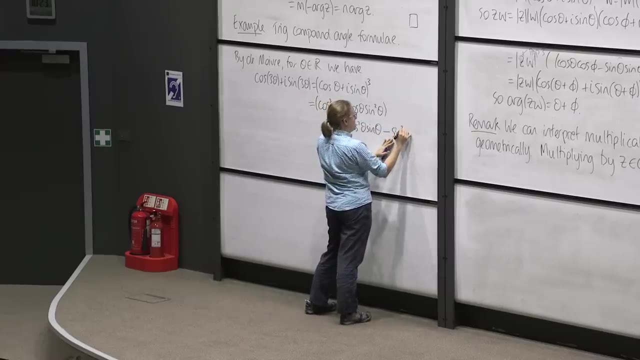 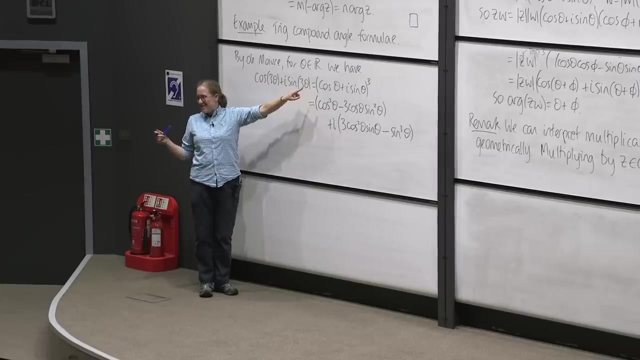 minus 3 cos theta sine squared theta plus i times 3 cos squared theta sine. theta minus sine cubed theta. So that's just by multiplying out. I've had quite a lot of practice at multiplying out cubes and I'm just trying to tidy up the 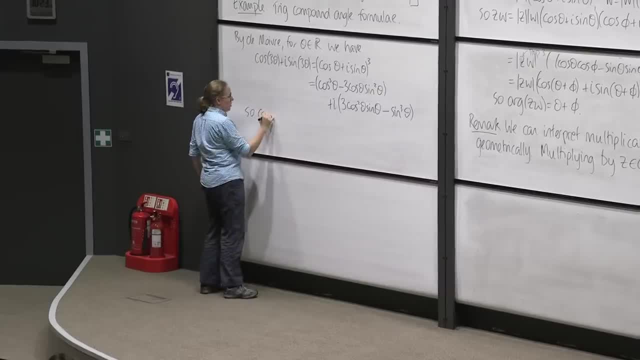 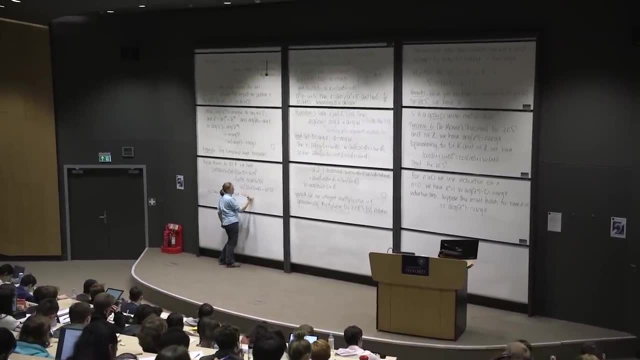 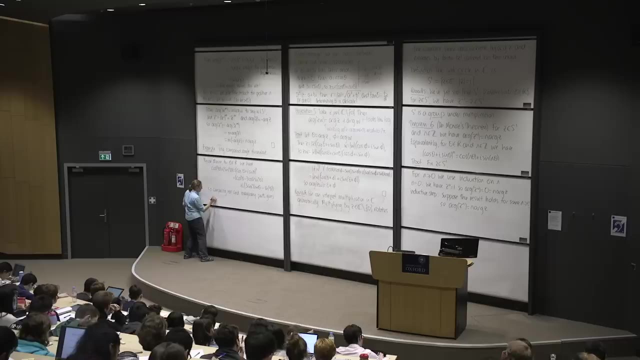 real and imaginary parts as I go along. So comparing real and imaginary parts gives that cos of 3 theta is cos cubed theta minus 3, cos theta sine squared theta. and then I got a formula for sine squared theta in terms of cos theta, right. So I could kind of keep going. 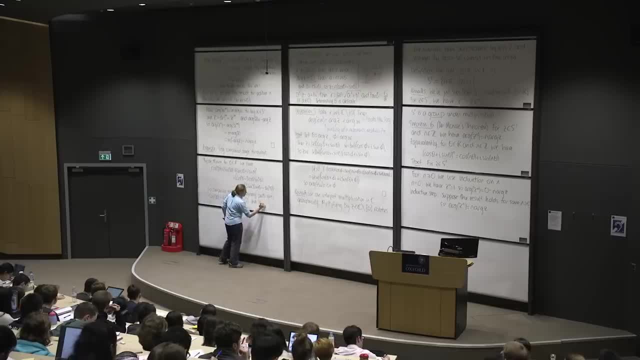 and tidy up, and I could write out some kind of corresponding formula for sine 3 theta and again tidy that up. So I'm going to let you do that tidying up while we have a short pause. I also have one other thing for you to do in this. 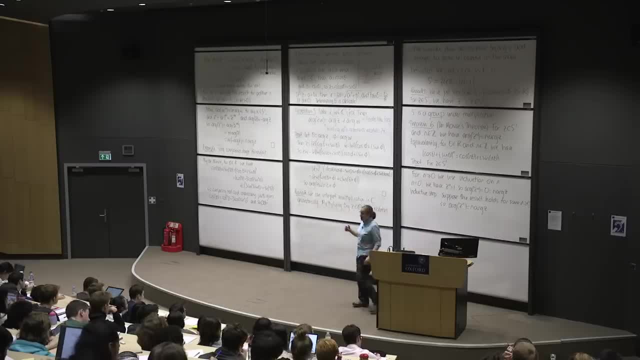 short pause At the end of each of your lecture courses. this year, we'll give you a paper questionnaire towards the end of the course so that you can give some feedback on how you found the course, how you found the lectures and so on, so that we can then, as a department, 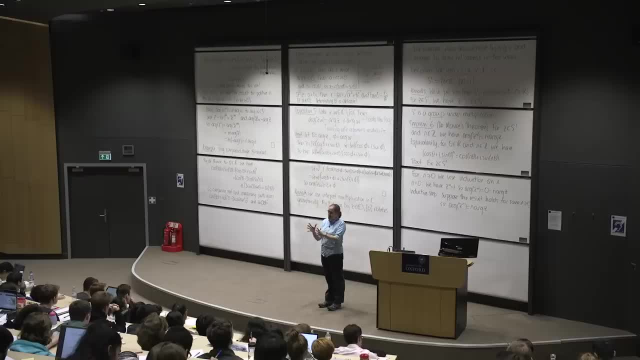 use that to improve teaching for next year, Even though it's only Thursday of week one, this is, in fact, the last lecture of this course officially, which means it's questionnaire time, So I'm going to put some piles of these in strategic places. 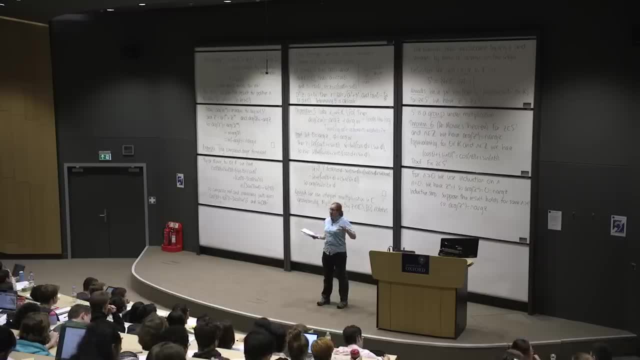 If you could pass them along so everybody gets a questionnaire, that would be great. If you want to fill it in during the lecture, you can, and if you just leave two piles, one at the top there and one at the top there, I'll collect them at the end, If you prefer. 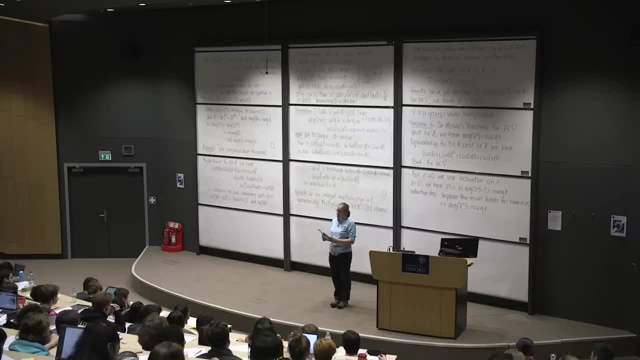 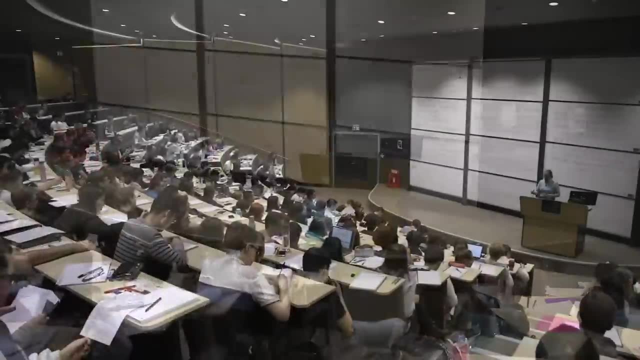 to fill it in later. you can also return it directly to the academic admin team, who are the people who process them. So this is your opportunity to give some feedback on the very short, complex numbers course. Okay, the questionnaires are making their way round, so, if you can, 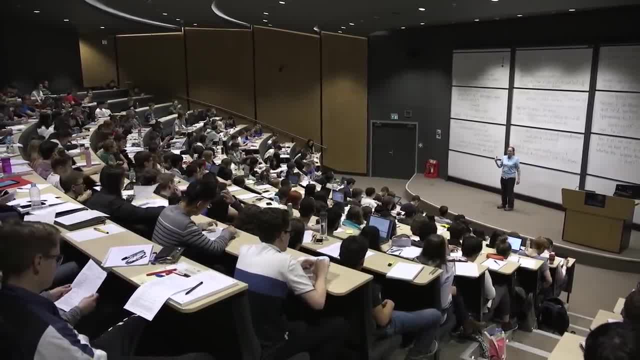 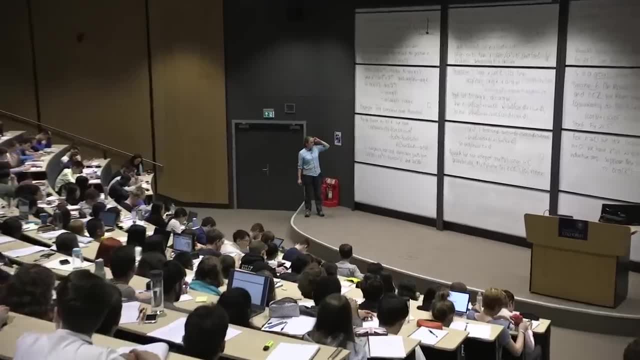 concentrate on keeping the momentum going, passing those round. that would be great, so that everybody gets them. I will try to remember in a couple of minutes to check that everybody's got them. But hopefully that's given you a little bit of a chance to think about these trig formulas especially. 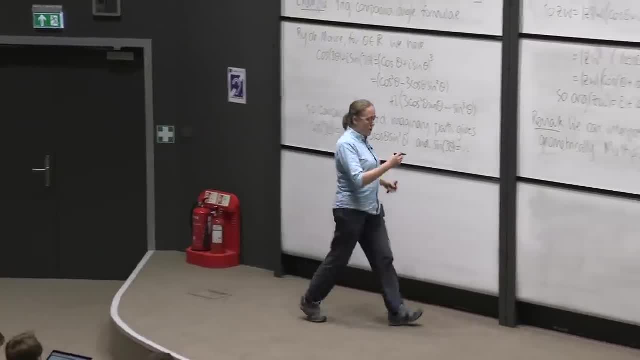 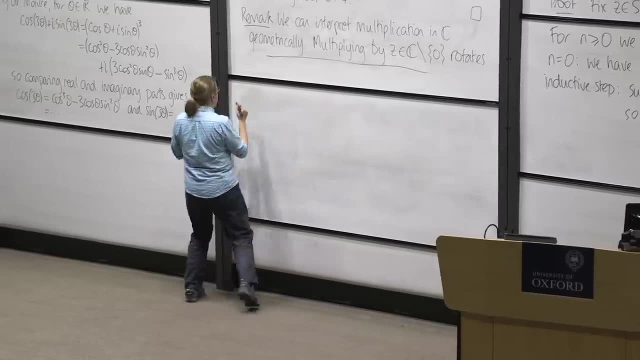 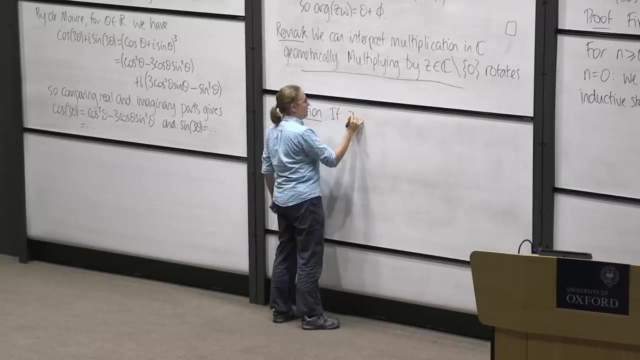 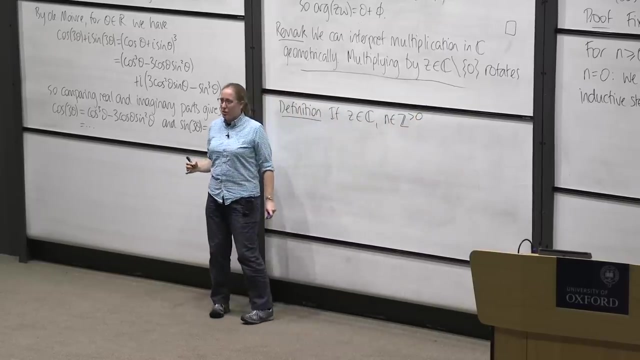 if this isn't something that you've thought about before, Let's keep going over here Because, excitingly, it's time for nth roots of unity. So here's a definition. So, if z is a complex number, n is a strictly positive integer, which you might call a natural number. 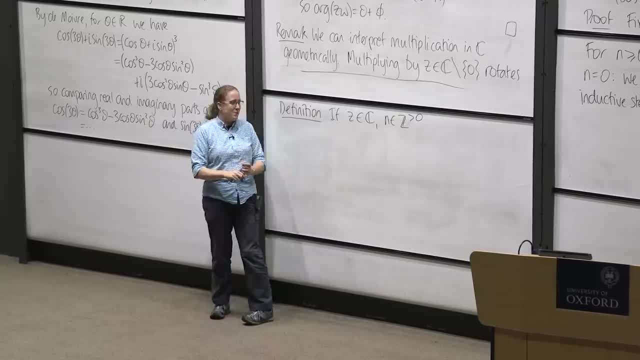 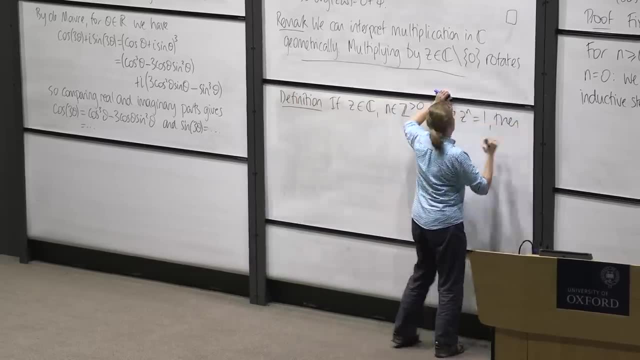 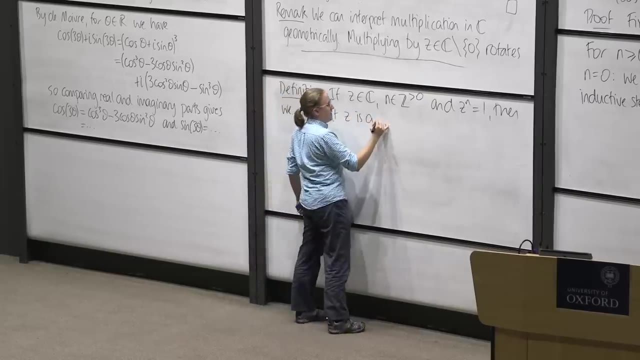 but somehow we can't decide whether or not zero is a natural number, and I don't have an argument about it. so I'm just trying to be unambiguous. and z to the n is equal to one, then we say that z is a root of unity. 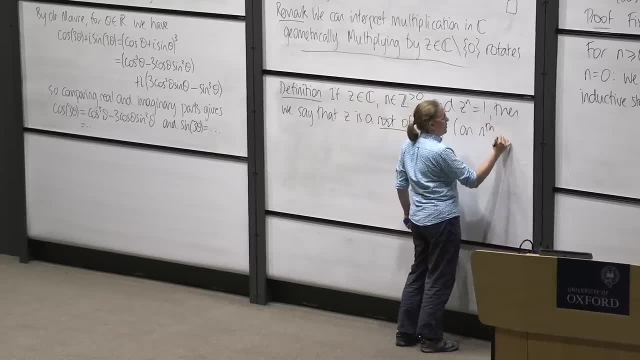 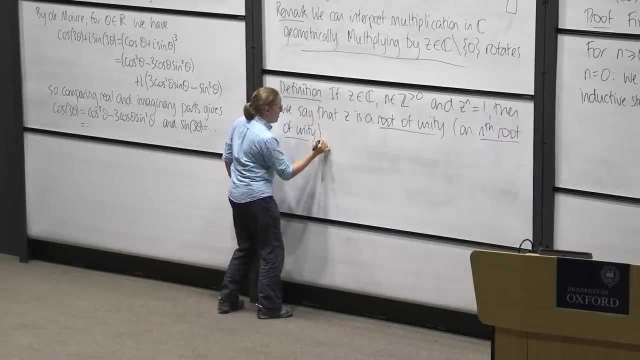 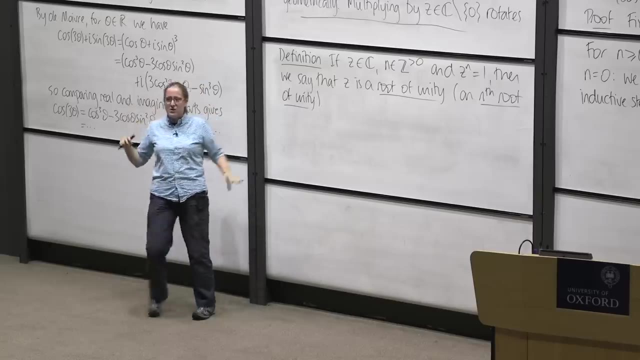 or more precisely, an nth root of unity. When I learnt about this stuff, I think I remember kind of thinking, oh, roots of unity, that sounds really cool. and then unity turned out to be one and it's sort of slightly less dramatic than I expected, But roots of one. 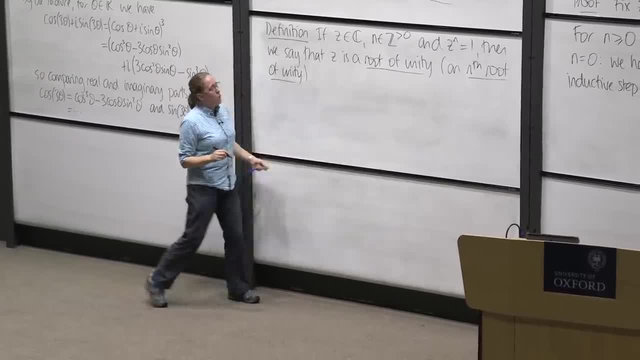 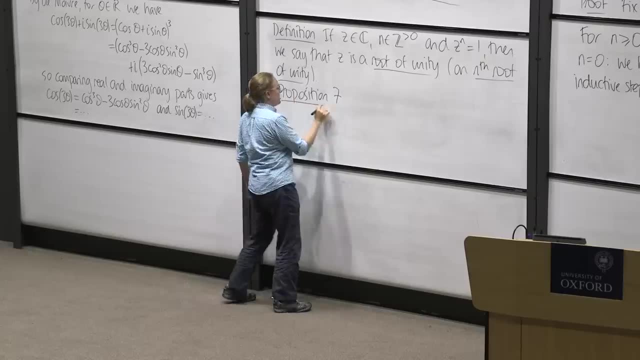 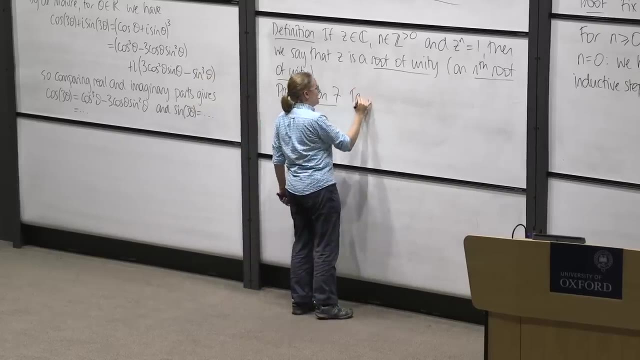 are still pretty good. There are lots of interesting things to explore. For example, proposition seven tells us which numbers are in fact roots of unity. So we can pinpoint where these things are without too much difficulty. So let's take z in c, then z is. 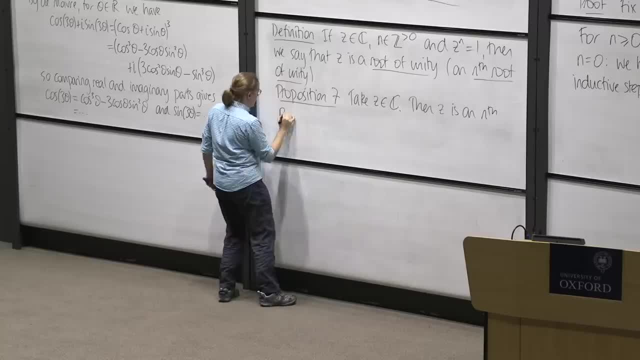 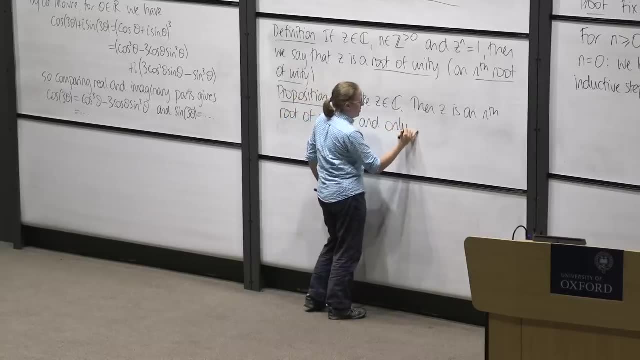 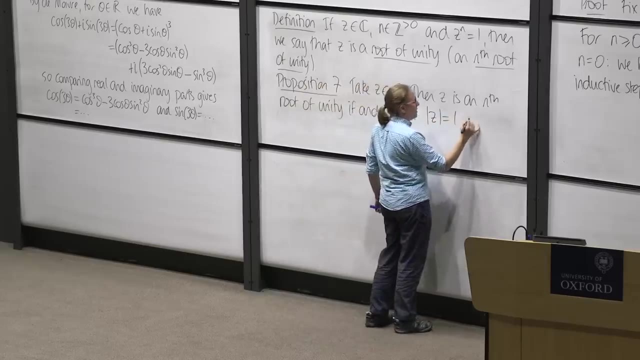 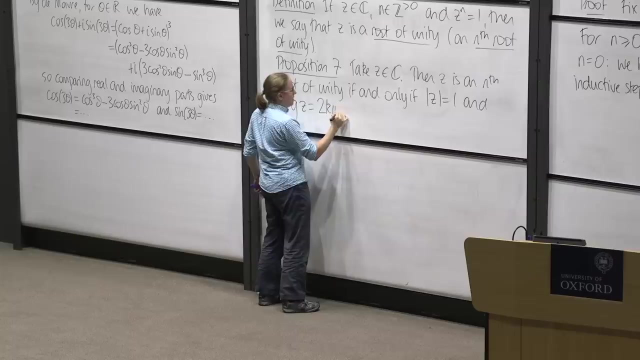 an nth root of unity, if and only if. and I've got two conditions here, One on the modulus of z and one on the arguments of z. So I need the modulus of z to be one and the argument of z to be two. k pi over n. 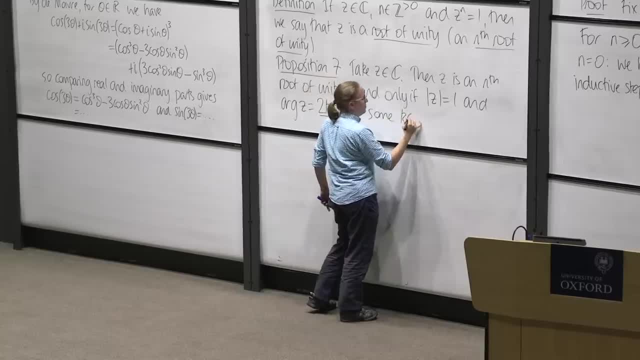 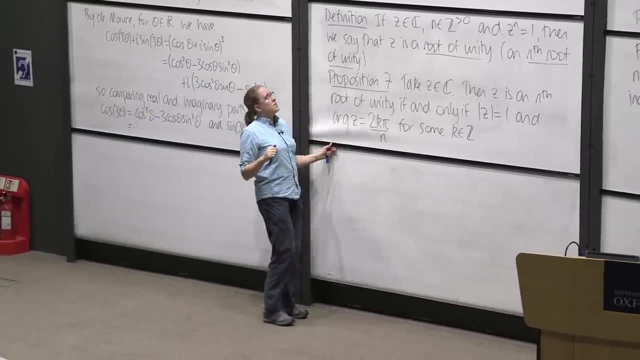 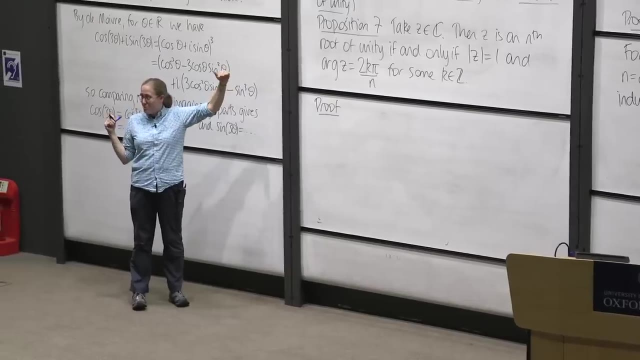 for some integer k. So this precisely describes what the nth roots of unity look like. So let's prove proposition seven, and you'll notice that proposition seven is an if, and only if statement. so it's really two statements packaged as one. Let's prove the two separately. 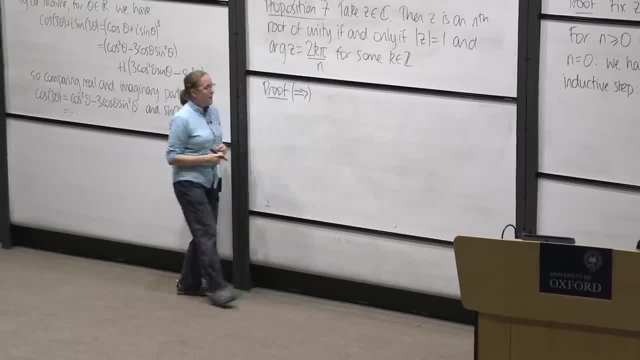 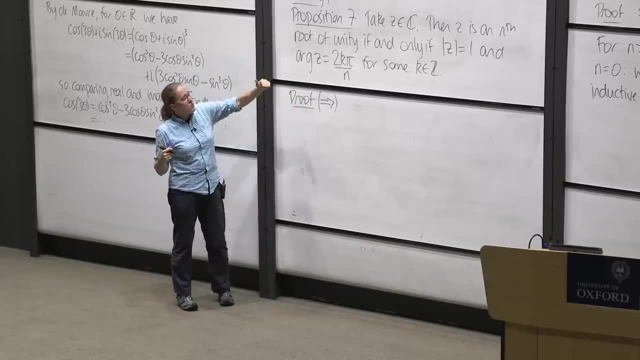 and try to help you see which one we're doing. I find it helpful to write these little kind of implication arrows and brackets When I'm doing this for my own benefit. I do this, not just for you. So we're going to do the left to right first. 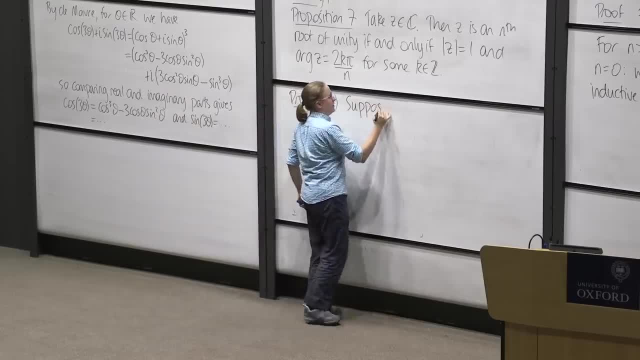 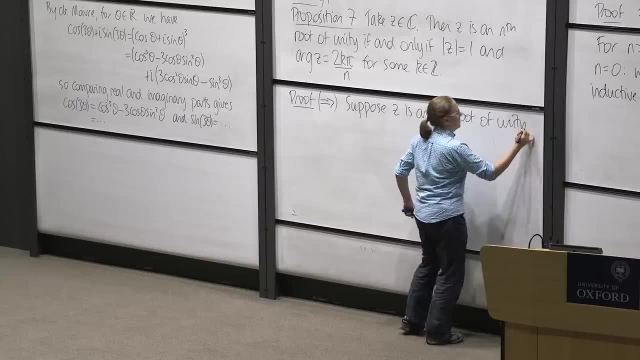 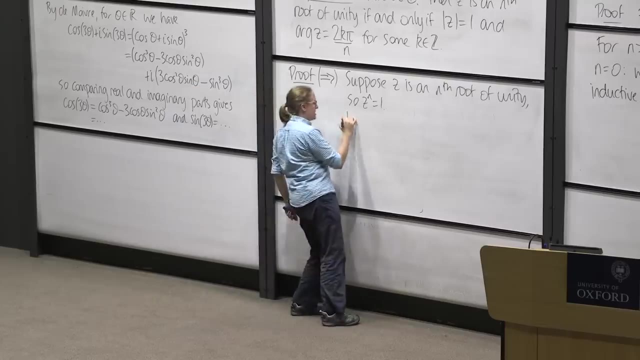 So we're going to suppose z is an nth root of unity, so we're supposing that z to the n is equal to one, and then we want to deduce kind of interesting things. Well, we can say something about the modulus straight away, The modulus of z. 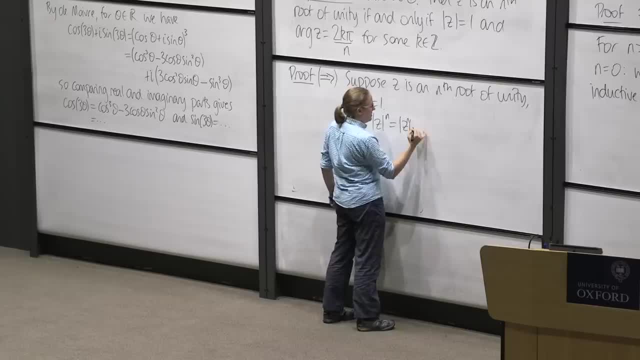 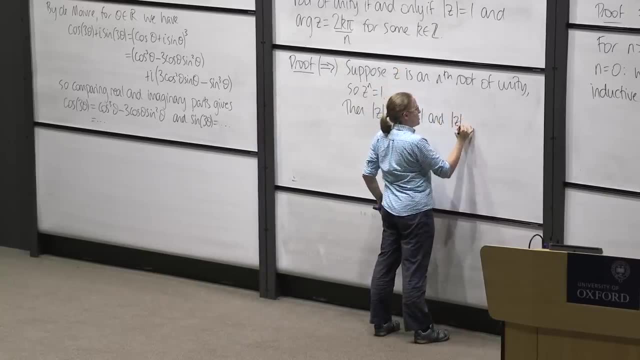 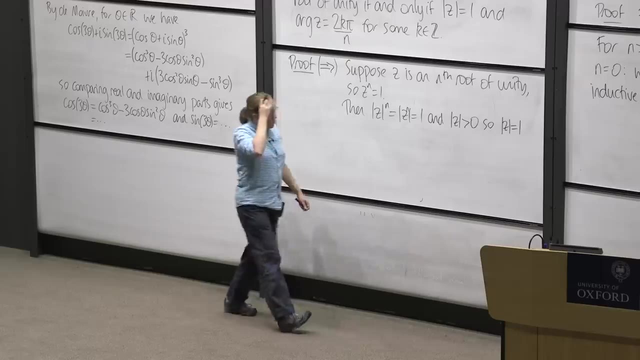 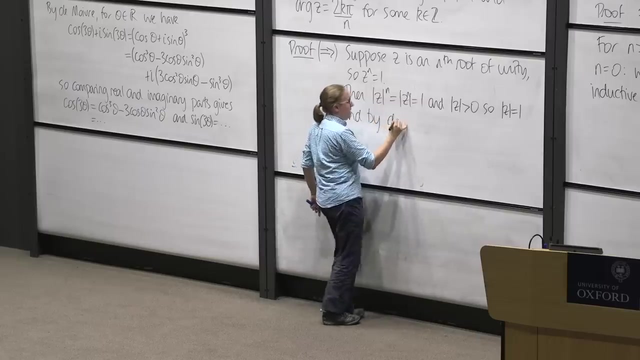 to the power n is. the modulus of z to the n is one and the modulus of z is strictly positive. so the modulus of z better be equal to one. So modulus of z is just a real number here, and by de Moivre, which conveniently we've just proved, 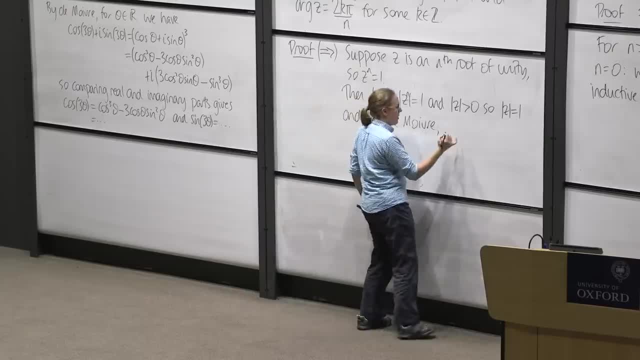 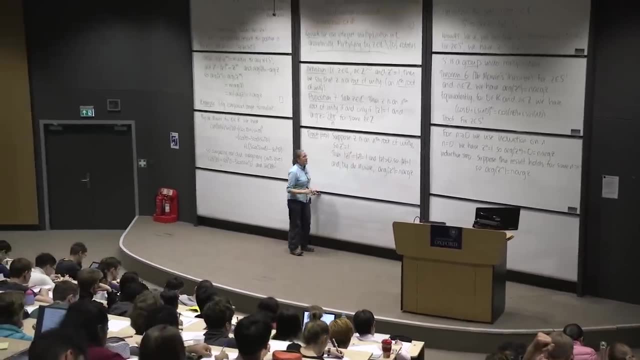 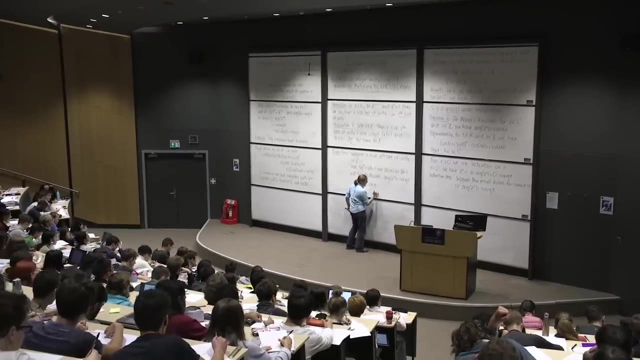 and comma by de Moivre. comma. the argument of z to the n is n times the argument of z, but we know that z to the n is equal to one, so the argument of z is the argument of one over n. and now we have to concentrate because there's a little. 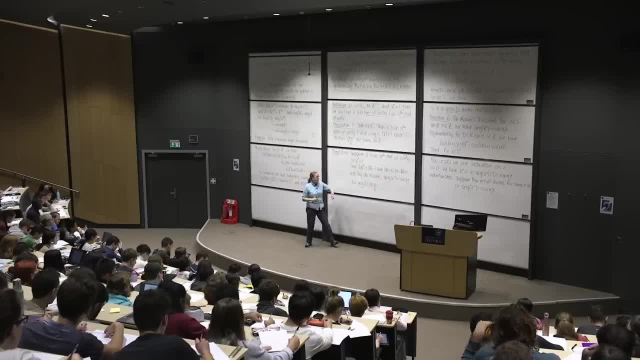 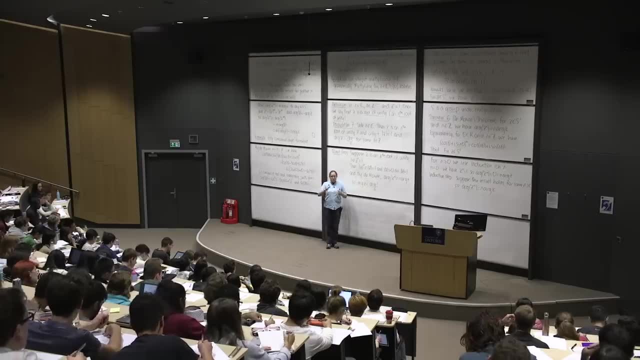 subtlety here, because we're working with arguments modulo two pi. So it'd be tempting to say the argument of one is zero, therefore this is zero, and that wouldn't be correct. all we know is that the argument is zero plus an integer multiple of two pi. 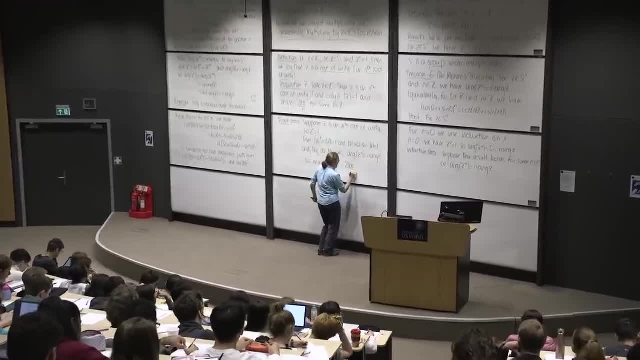 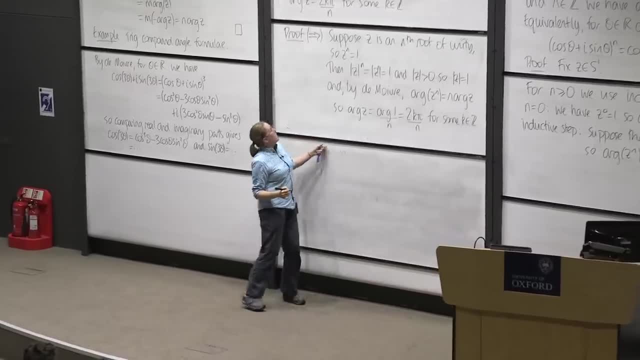 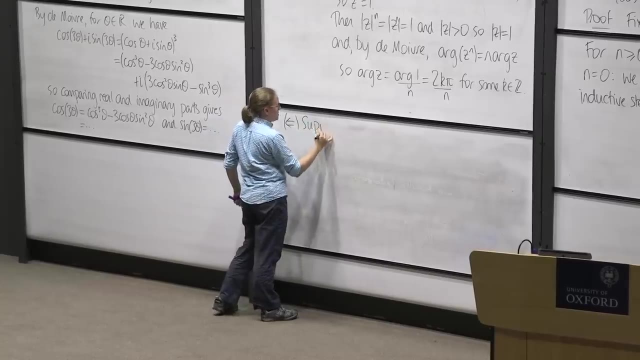 so what we know is that this is two k pi over n for some integer k, and that gives us what we were looking for. the other direction. let's get rid of these smudges for you, the other direction. so now we're going to suppose that the modulus of z is equal. 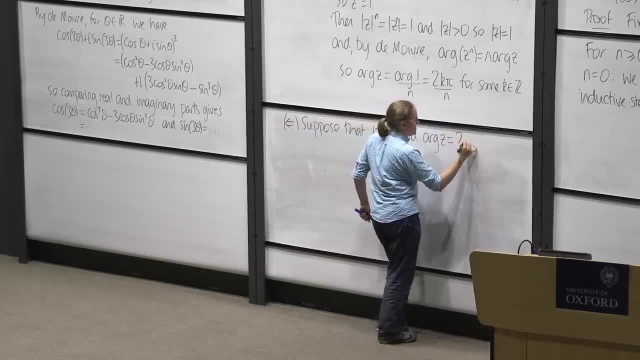 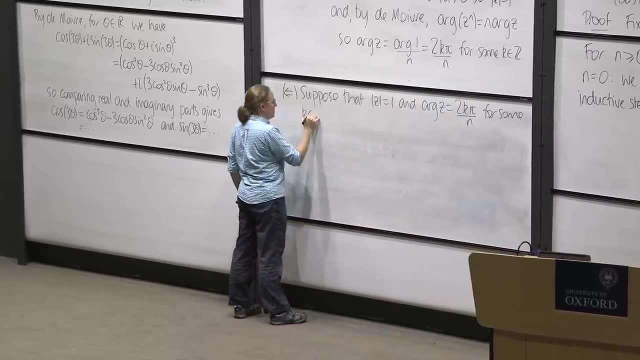 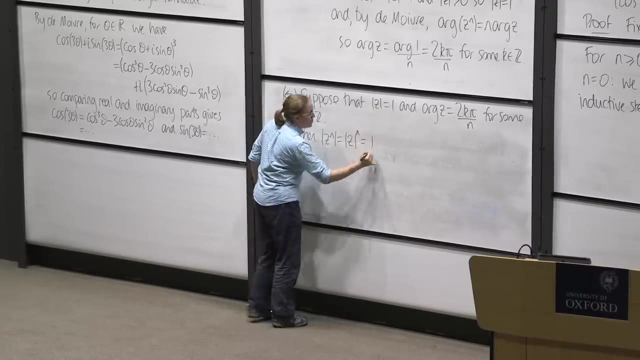 to one and the argument of z is two k pi over n for some integer k. so then what can we say about the modulus of z to the n? Well, that's, the modulus of z to the n is one we like modulus works out really nicely. 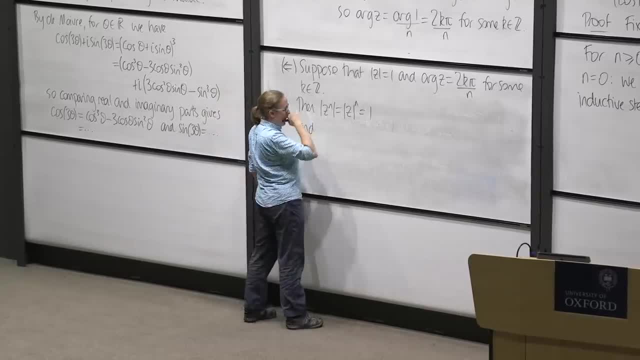 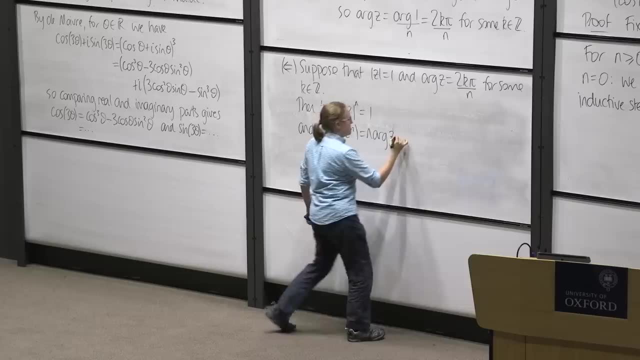 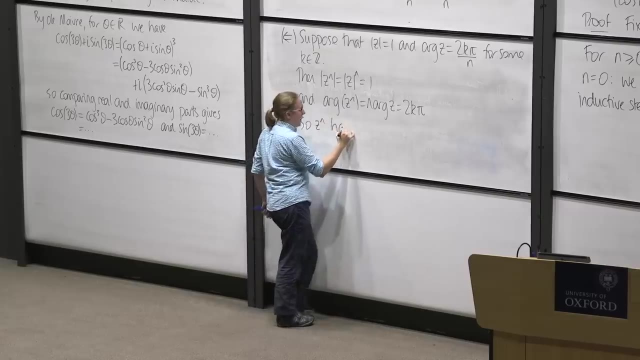 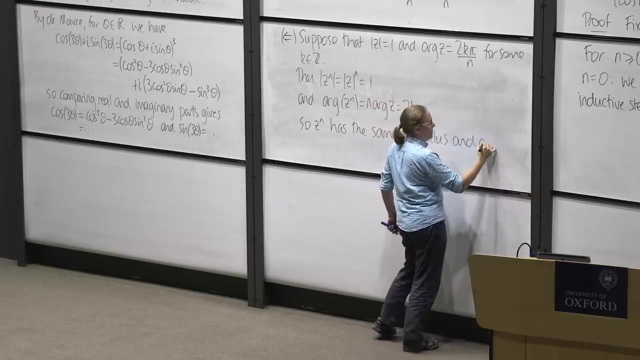 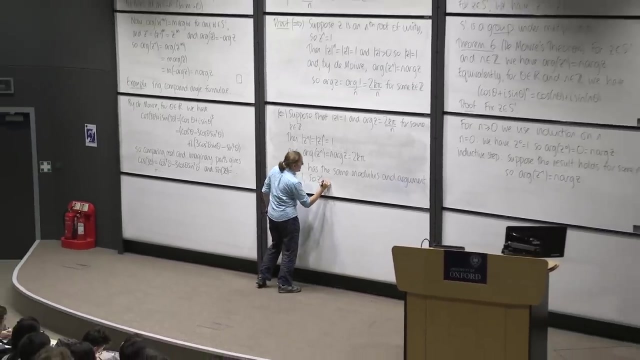 and also the argument of z to the n is n times the argument of z is two k pi. so what's that telling us? It's telling us that z to the n has the same modulus and argument as one. so in fact, z to the n is equal to one. 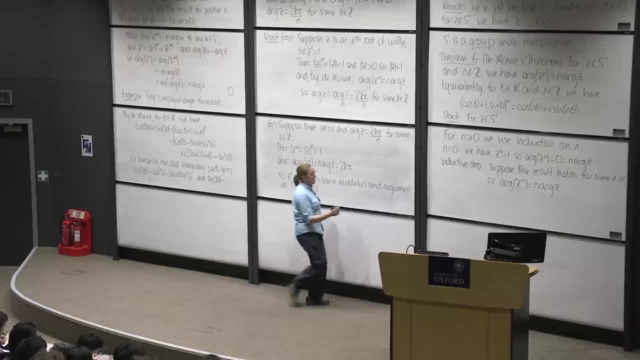 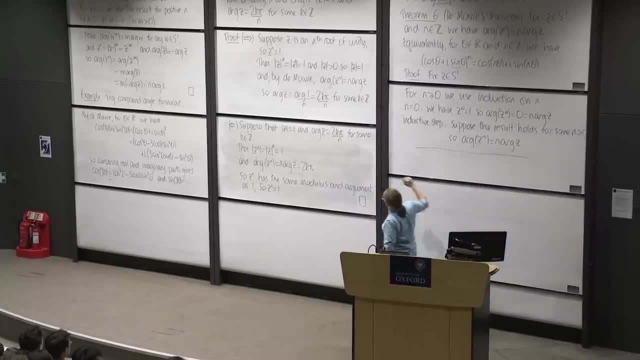 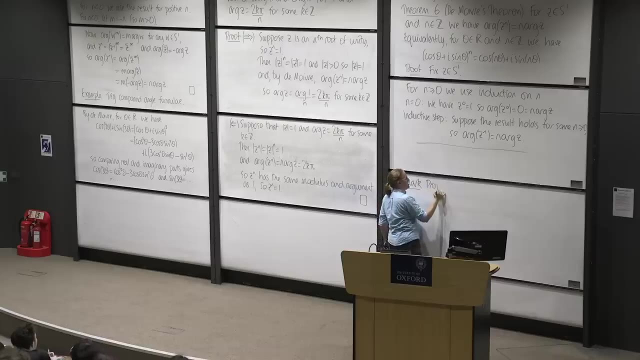 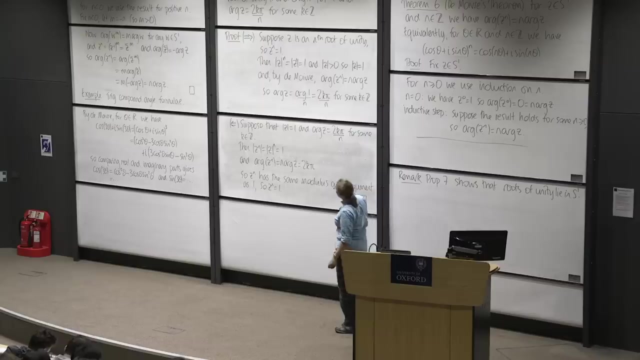 so z is an n-th root of unity, and that finishes our proof. so if I carry on over here, so one small observation from proposition seven. so remark. proposition seven shows that roots of unity are lie in s1, they lie in the unit circle, and that's a kind of handy thing to be. 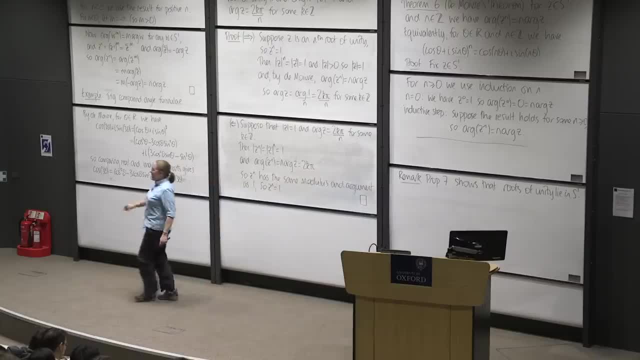 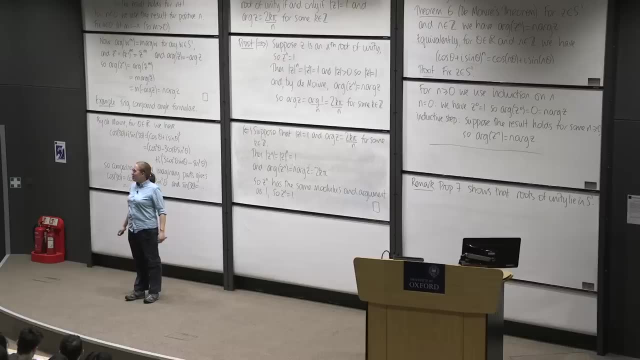 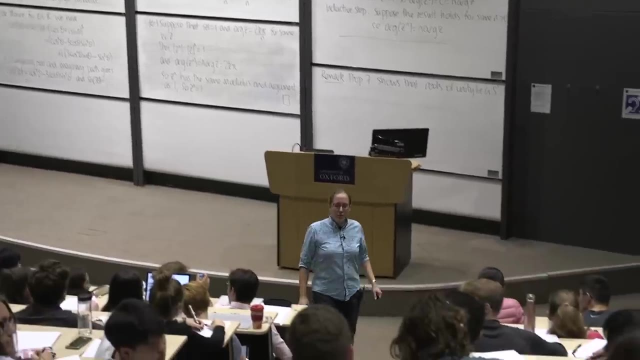 aware of occasionally. right, how are we doing on questionnaires? could you please put your hand up? if you do not have a questionnaire interesting, could you please put your hand up if you have some spare questionnaires. okay, so the people who didn't have questionnaires: 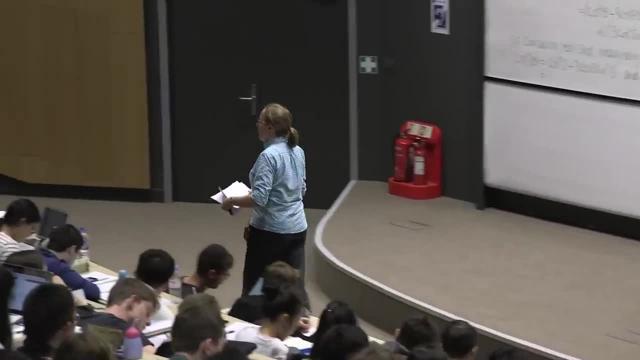 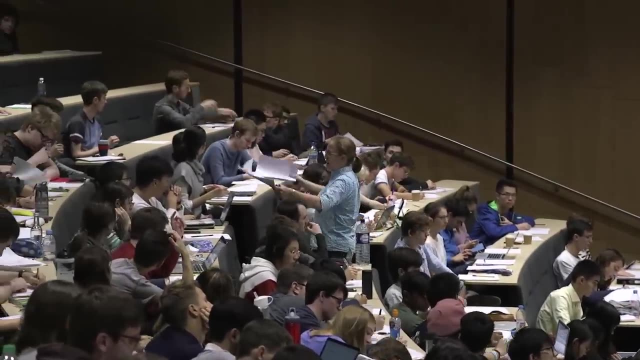 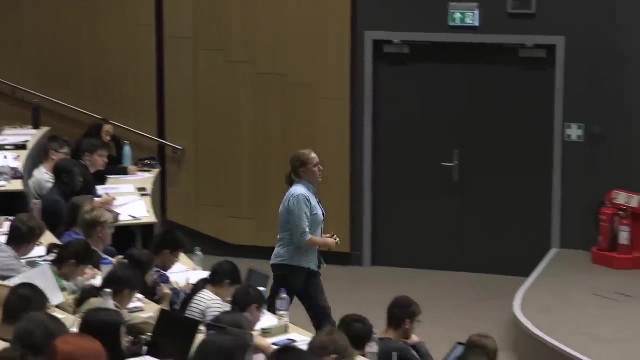 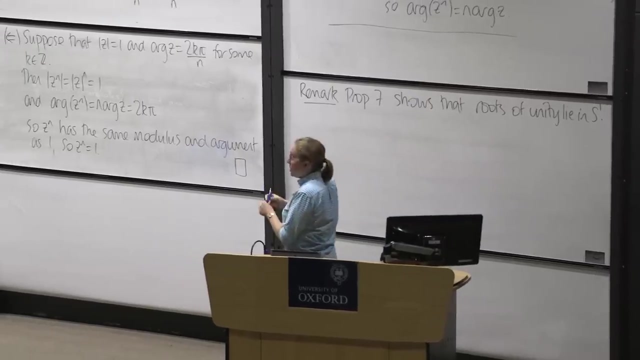 were over here somewhere. oh, thank you. more questionnaires wave, if you need a questionnaire, okay, so I'm going to send some this way and some this way, and it would be great if you could sort them out amongst yourselves, and hopefully they're enough so cute. consequence of 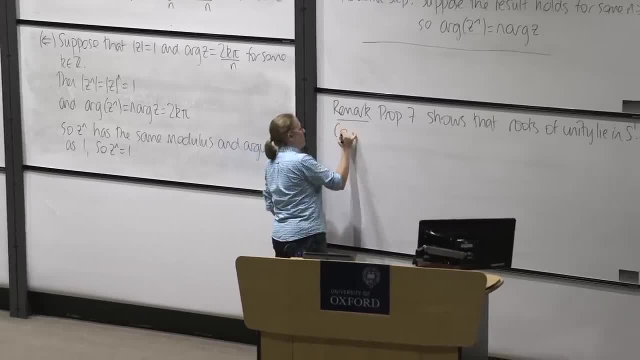 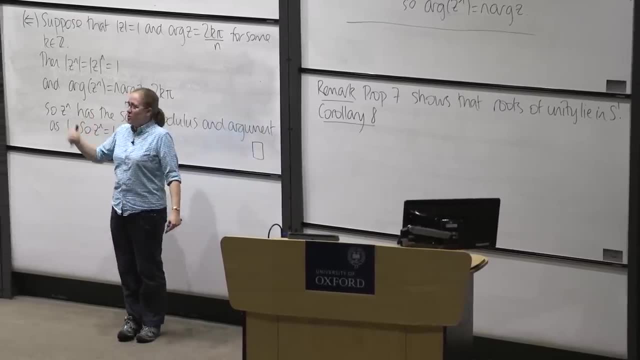 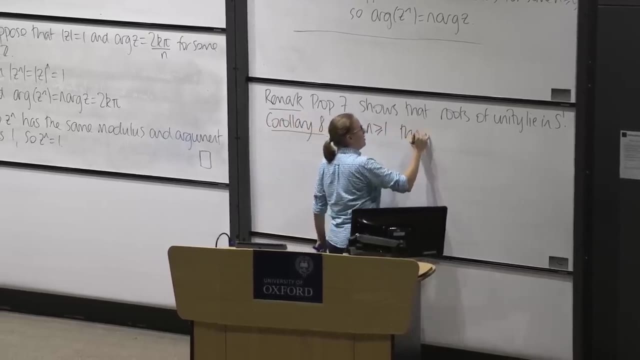 proposition seven is that we can count n-th roots of unity. so I think maybe I said on Monday, corollary is a quick consequence of something you've already proved. so corollary eight says for n greater than or equal to one, there are exactly n. 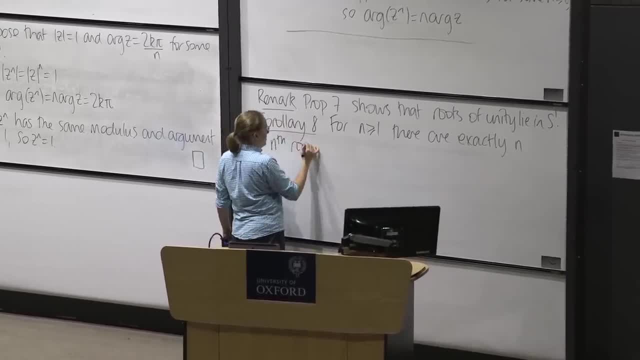 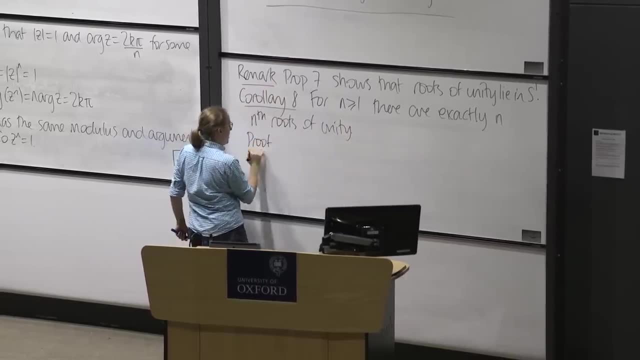 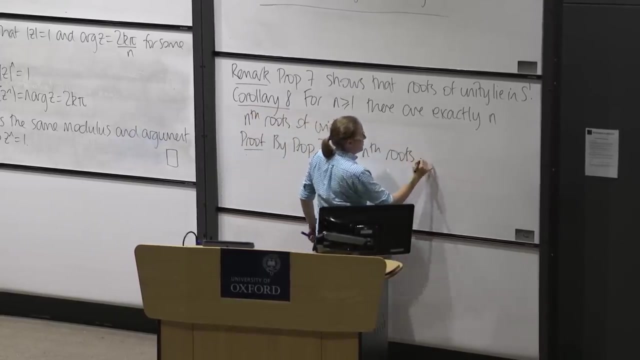 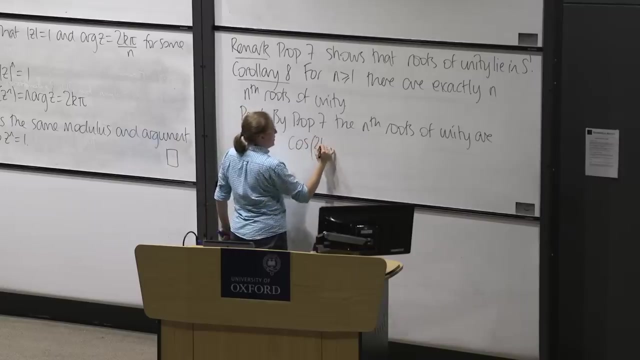 n-th roots of unity. and that's quick to prove from proposition seven, because we know what the n-th roots of unity are. so by proposition seven the n-th roots of unity are. so one way of writing them would be: is cos of 2k pi. 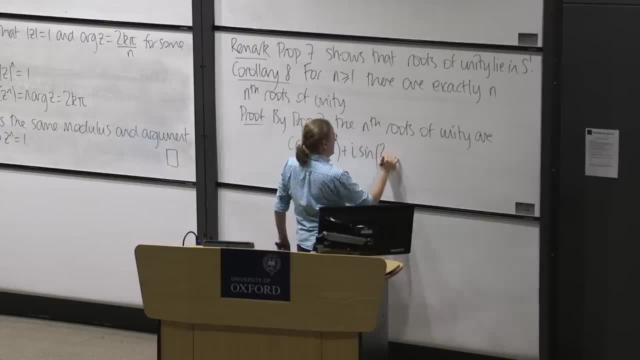 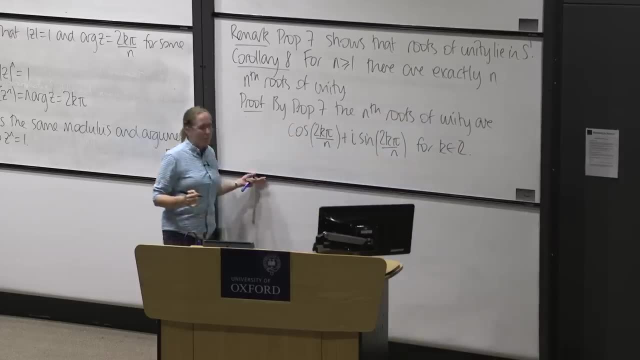 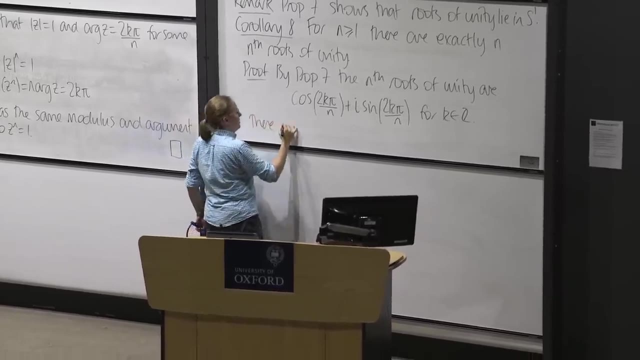 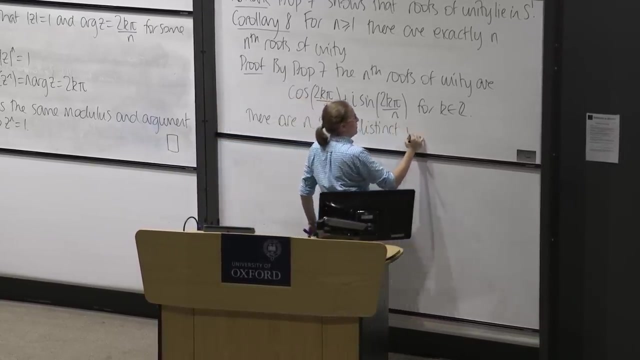 over n plus i sine of 2k pi over n for any k in the integers. that makes it look like there are lots of them, but of course there's lots of duplication here. so there are are n such distinct values eg we could choose. 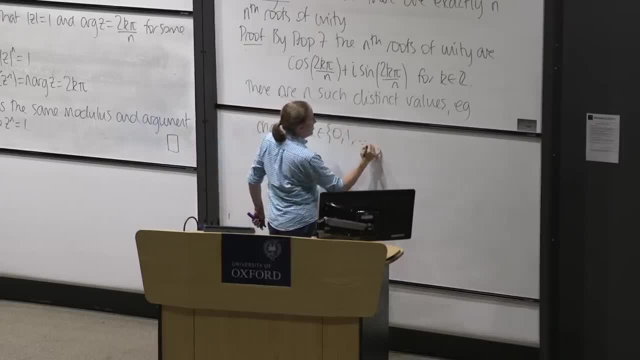 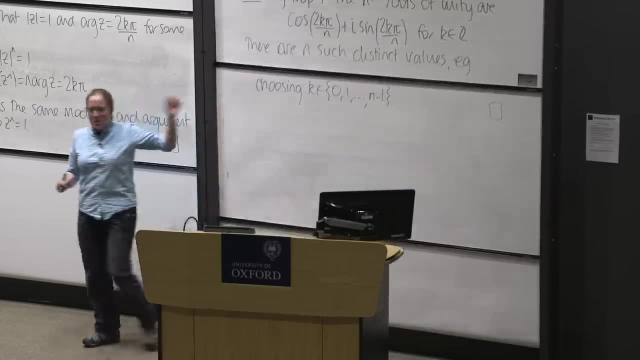 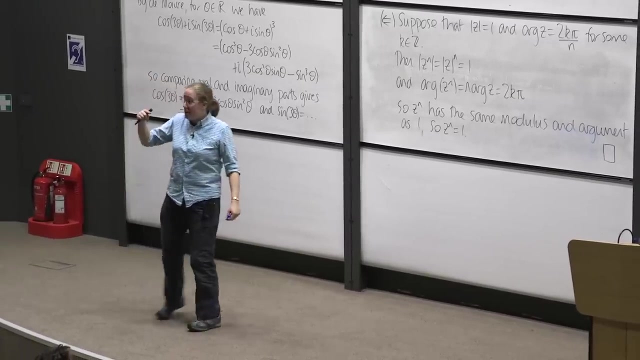 k to come from zero one to n minus one, so that was a handy consequence. it's good to know not only where the n-th roots of unity are, but that we've got n n-th roots of unity. that's a good thing to know. there are some n-th roots of unity. 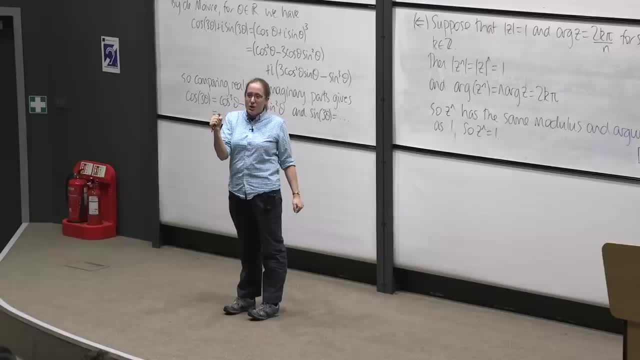 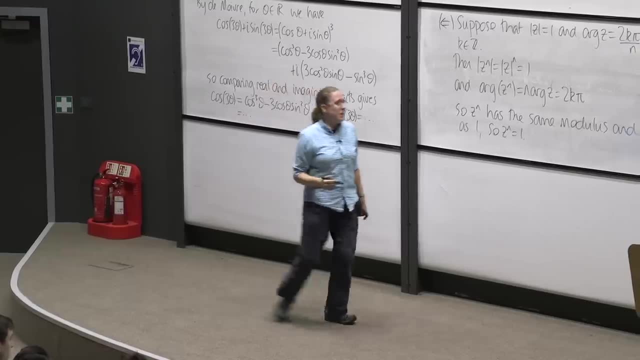 that are even more exciting than others. there are some n-th roots of unity that are n-th roots of unity but aren't smaller roots of unity, aren't n-th roots of unity for smaller m? and they're particularly important, so they get a special name. so this is a definition. 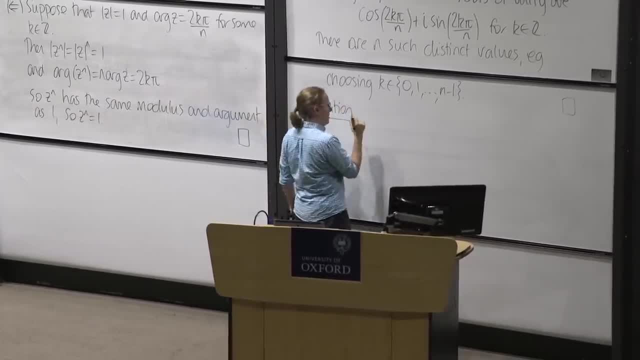 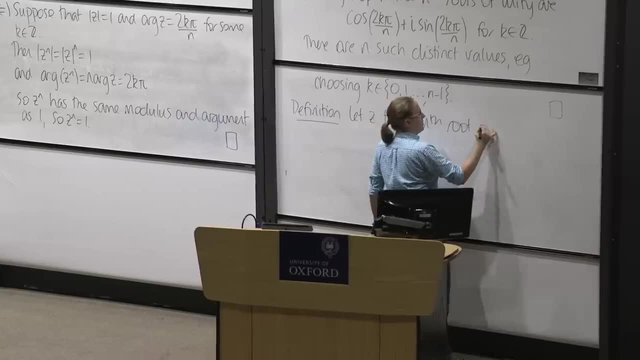 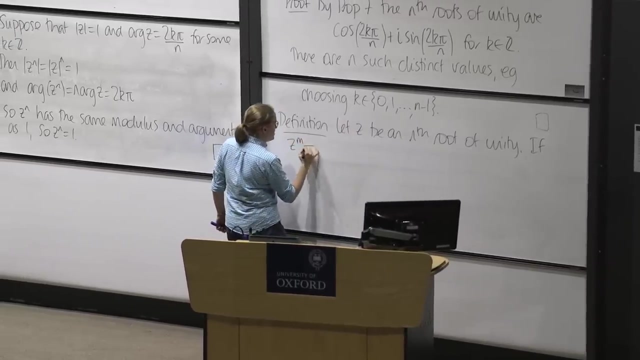 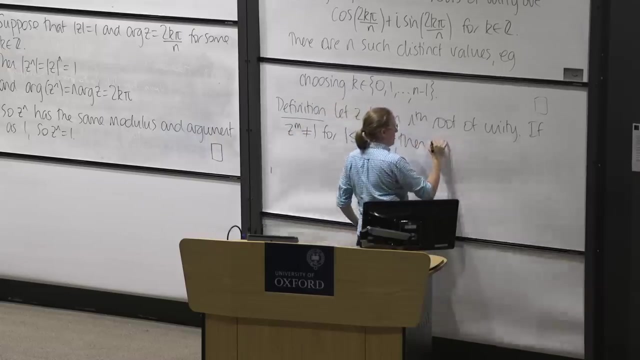 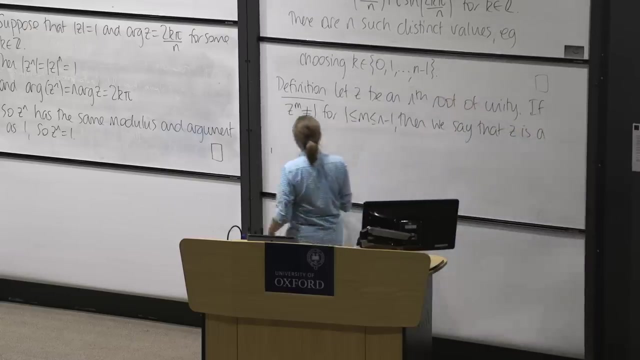 of n-th roots of unity. so let z be an n-th root of unity. if z to the m is not equal to one, for one less than, or equal to m less than or equal to n minus one, then we say that z is a primitive n-th root of unity. 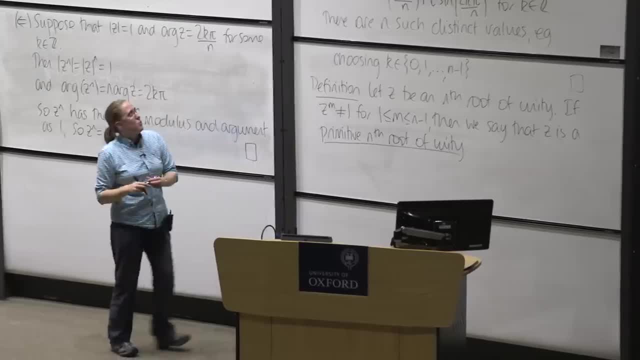 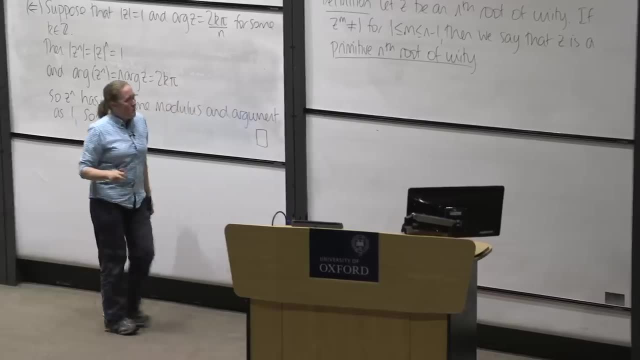 and these kind of have connections with things from group theory and other things that you will see- that was a very strange noise- other things that you will see this year. so a primitive n-th root of unity is like: n is the first power of z where you get. 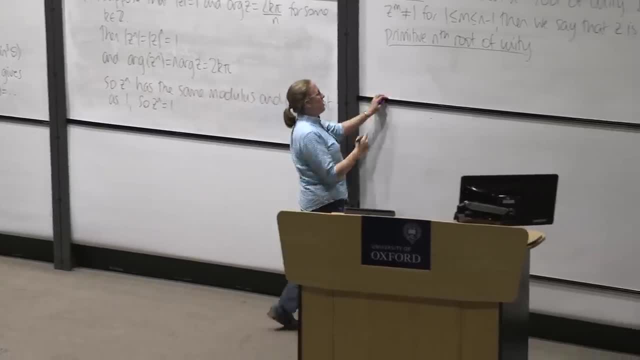 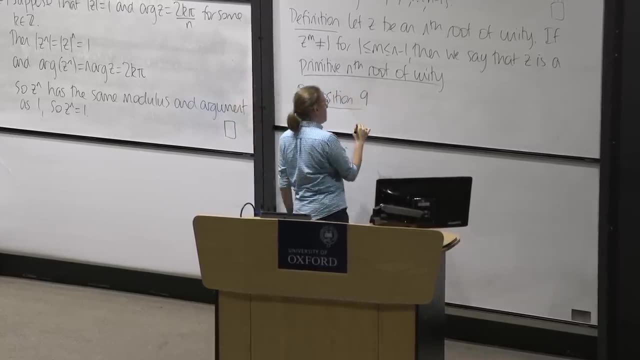 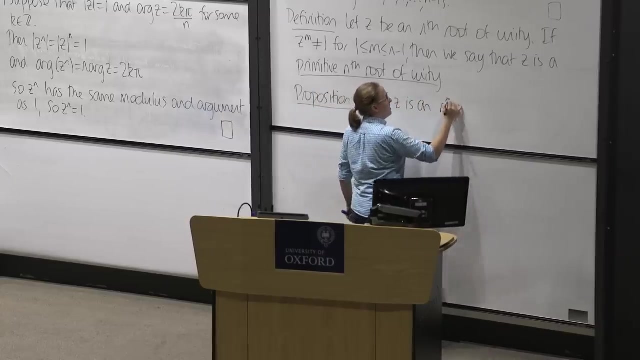 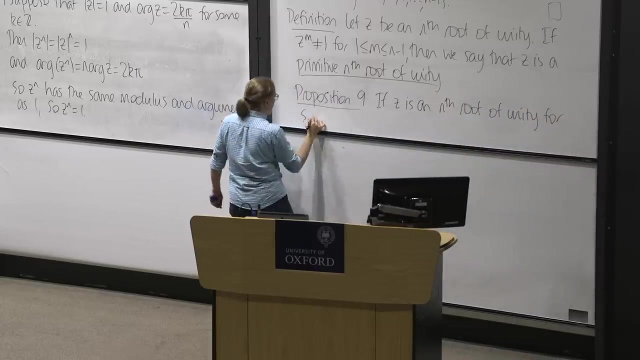 one. so here is a proposition that is useful and certainly applies to primitive roots of unity, although it applies a little bit more generally than that as well. so if z is an n-th root of unity, for some n greater than or equal to two and z is not equal to one, 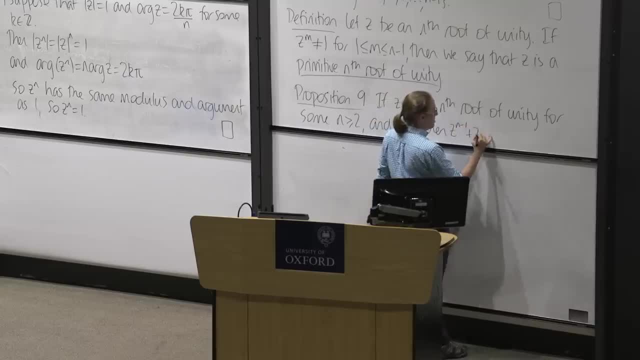 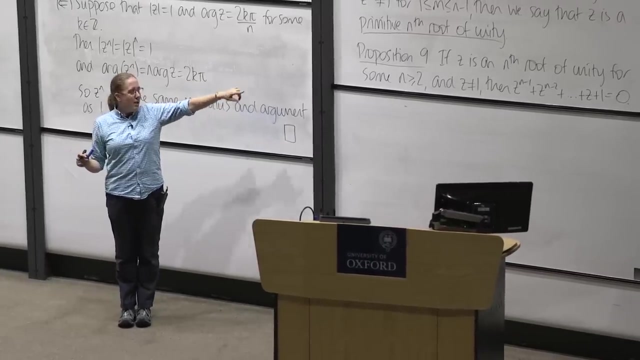 then z to the power n minus one plus z to the power n minus two plus dot dot dot plus z plus one is equal to zero. this is the kind of thing where, if I were working on these lecture notes this afternoon, thinking about them, I'd be thinking: oh, why has Vicky? 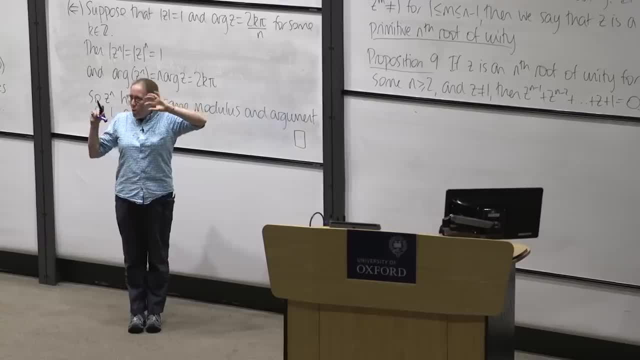 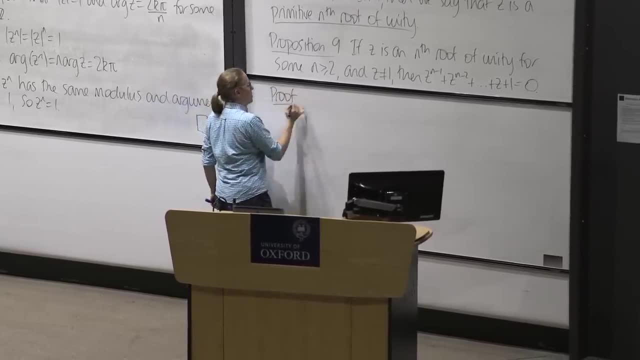 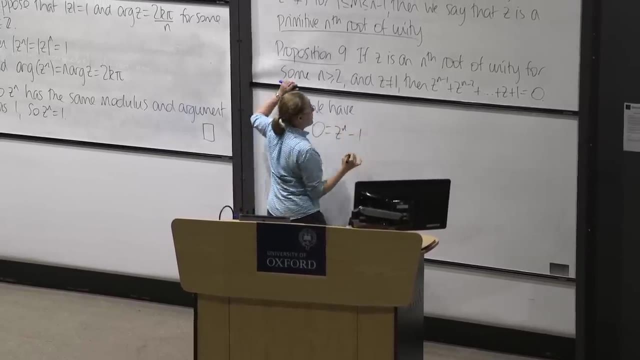 excluded the case when n equals one. what was special about that? that kind of why are the hypotheses there? that's the sort of question that you could be asking yourselves. so this is not too tricky to prove, because we know that zero is z to the n minus one. 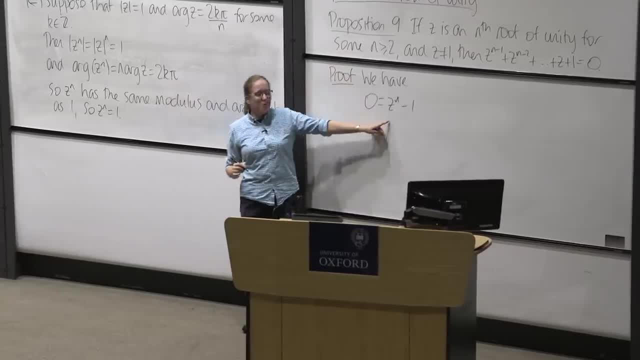 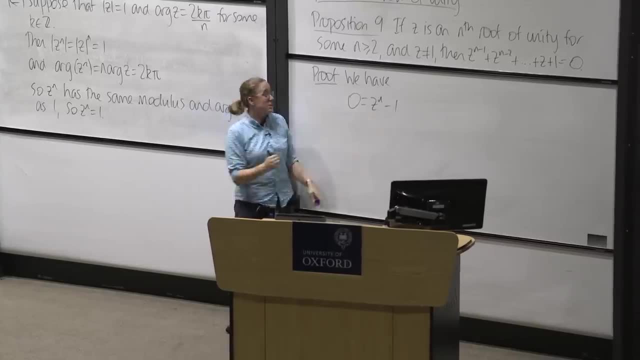 we're assuming that z is an n-th root of unity and we can factorise z to the n minus one. if this factorisation is not second nature to you, I invite you to think about it, because it's a really useful factorisation. it kind of generalises. 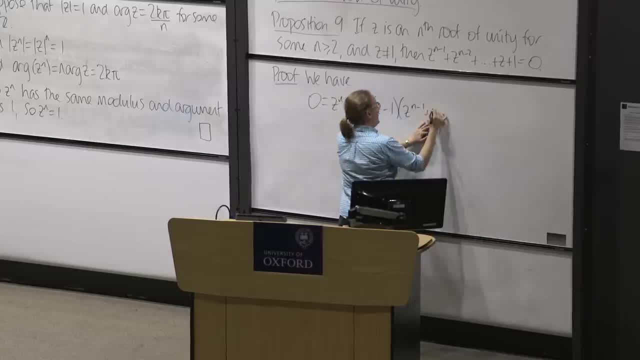 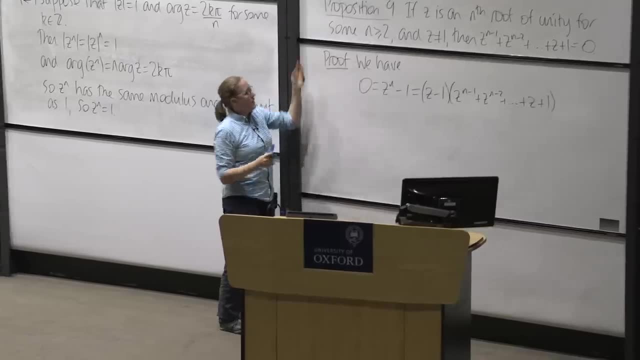 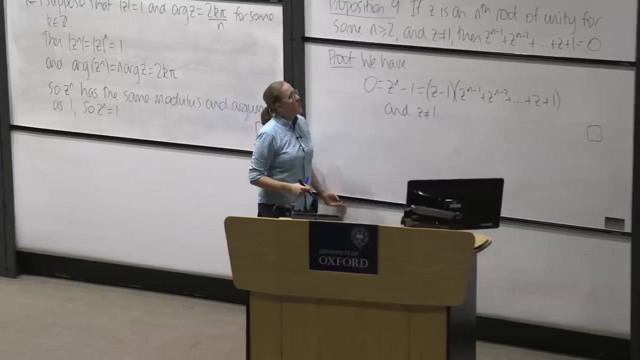 difference of two squares, and in fact it's this: and z is not equal to one, and that's the end of the proof. so this is not super difficult, but it's kind of useful. it's a nice result. so this starts to have some nice consequences geometrically. 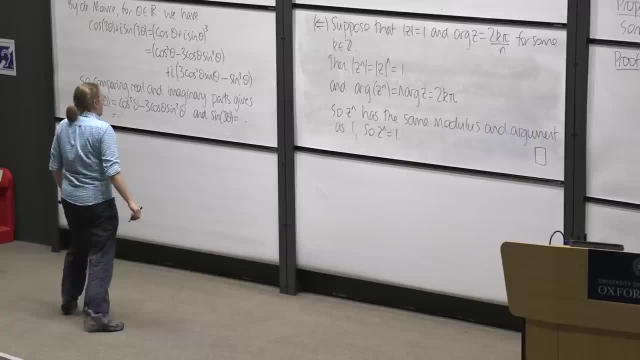 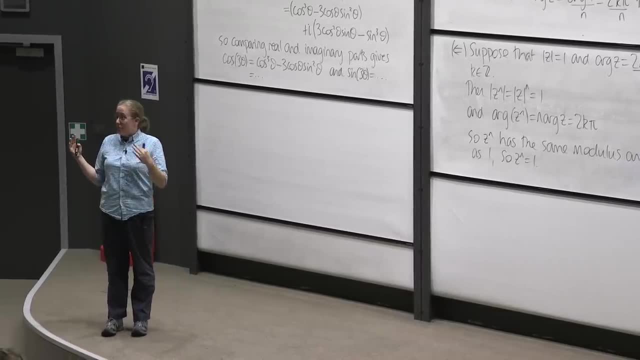 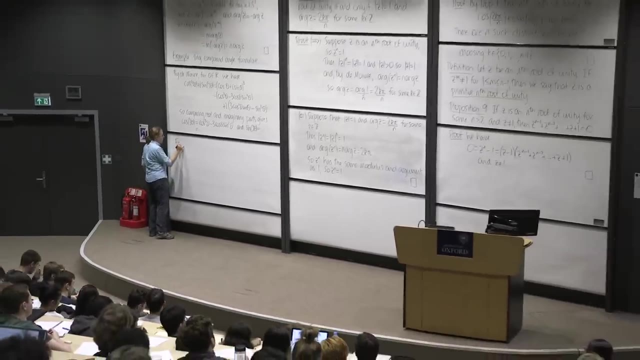 for example, when you're thinking about roots of unity. okay, I want to think about another way to represent complex numbers. we've sort of thought about modulus argument and we've thought about this Cartesian coordinates kind of way. there's another very useful way of writing them, which comes from the following: 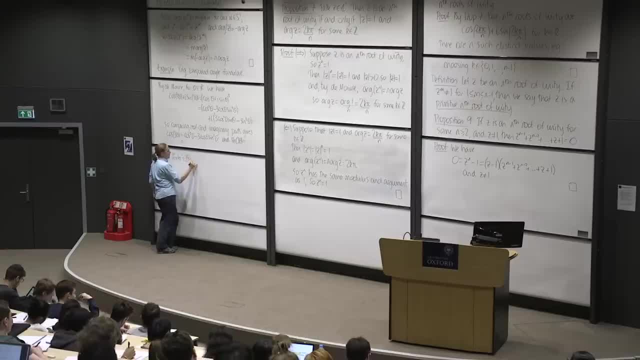 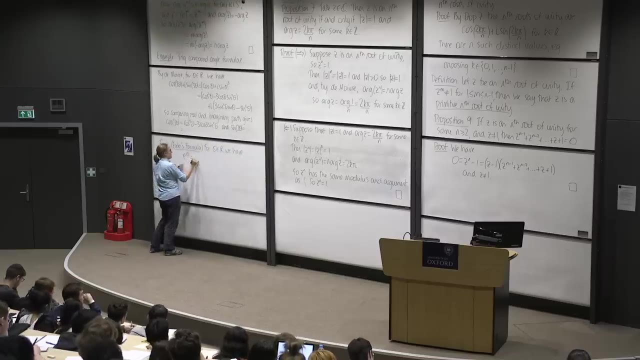 fact which gets called Euler's formula, at least sometimes. and this says for theta: in R we have e to the i, theta is equal to cos theta plus i sine theta. while you take ten seconds to just absorb how lovely that is, how are we doing with questionnaires? 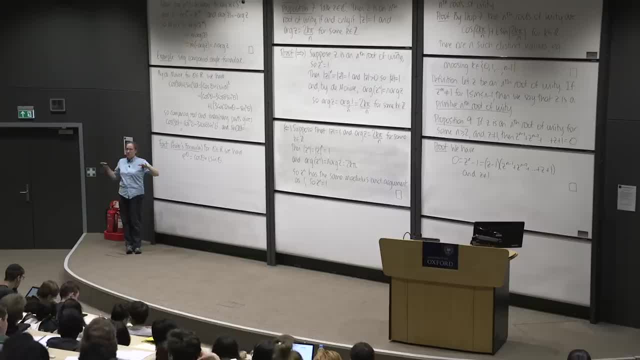 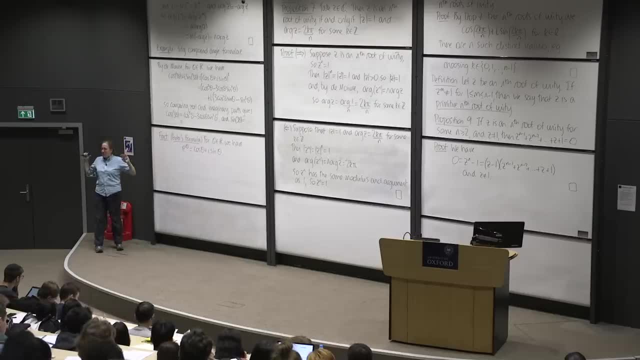 put your hand up if you do not have a questionnaire result. very good. now you will notice that I have labelled this as fact rather than theorem or any of those kinds of things. this looks a lot like a thing that needs proving right, and it does need proving. 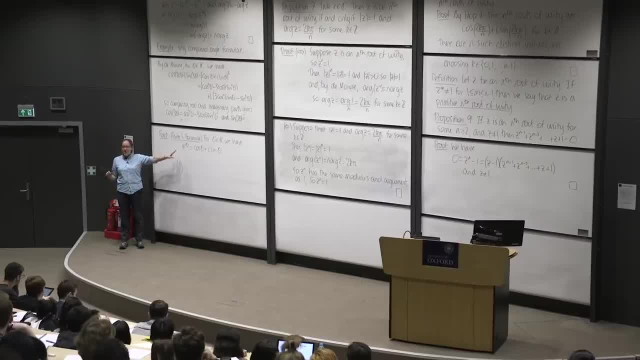 but in order to prove it, we first need to have defined the exponential and the cosine and the sine, and since we haven't done any of those things, we're not in a very good place to prove this. defining the exponential is something you will do in analysis. 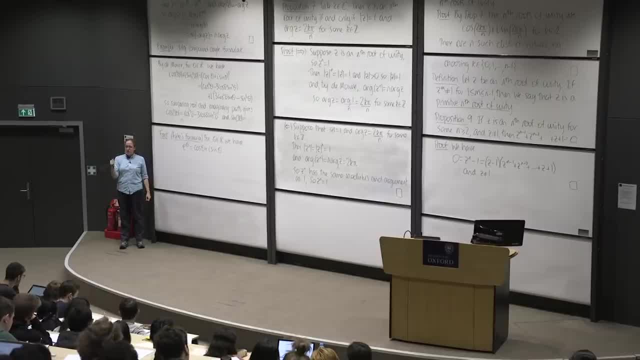 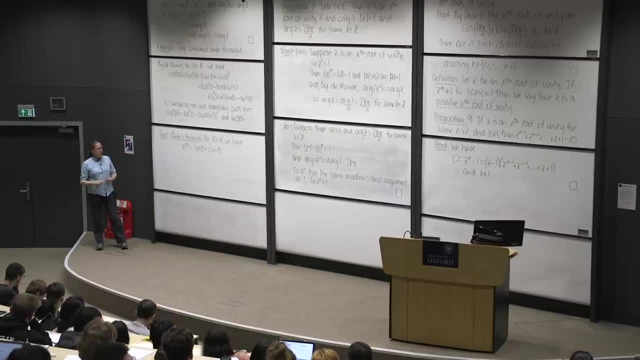 this year, and also cosine and sine. once you've learnt how to add up infinitely many things in a safe, controlled manner, it's very important to be careful when adding up infinitely many things. once you have got your licence that you are safe to do that, you can think about the exponential. 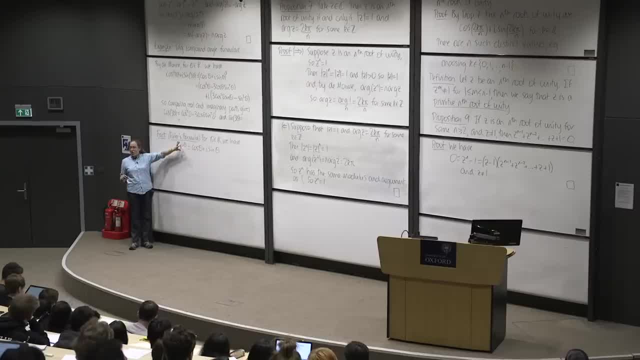 and then you'll be able to think about why this is true. so I just put a little bit more in the online notes. so if you want to read a little bit more about that, have a look at the online notes, but we're just going to accept this as a fact. 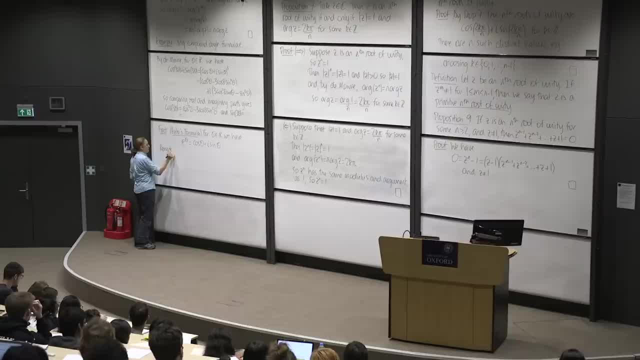 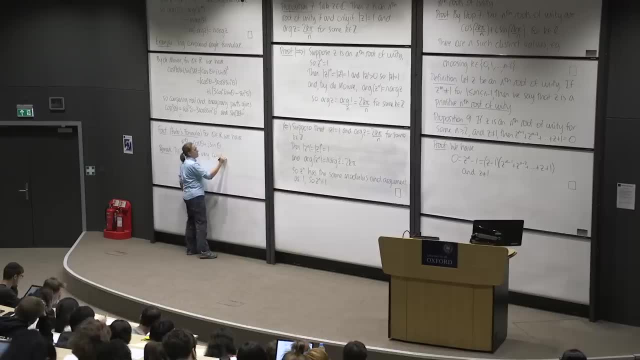 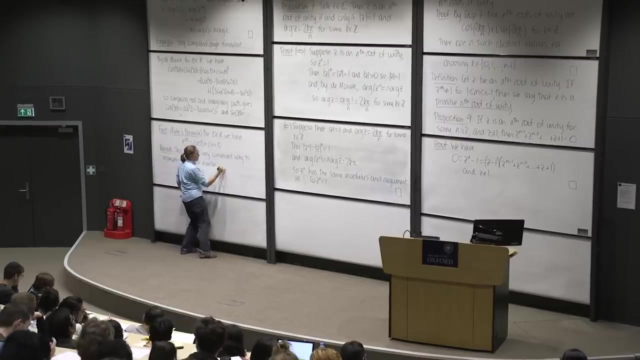 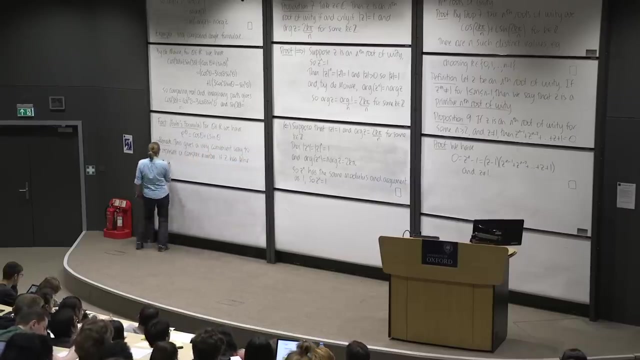 for our purposes. so here is a remark. this gives a very convenient way to represent a complex number. so if z has the modulus of z is r and the argument of z is theta, then z is re to the i theta. when I started learning about complex numbers, 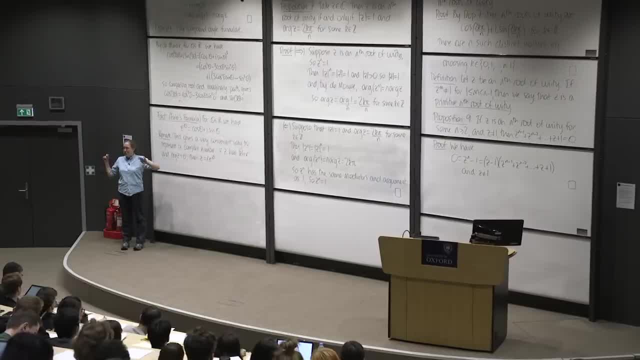 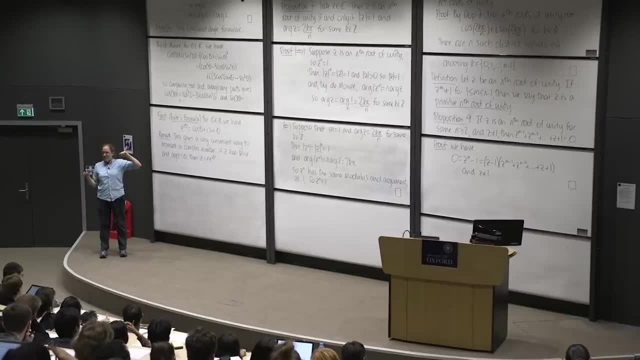 I definitely thought about the most in the a plus b i form and then I think when I was doing a level studying a bit further, I thought about the more in the r times, cos theta plus i sine theta form, and I probably think about the more in this form now. 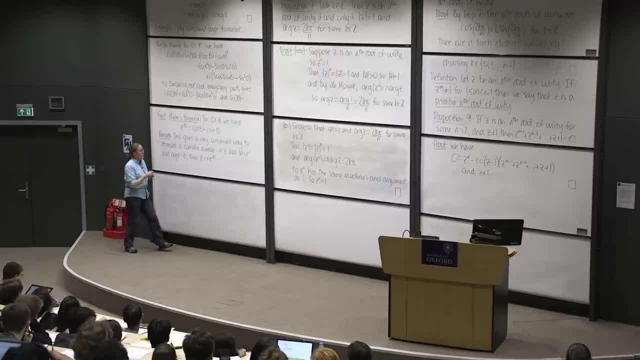 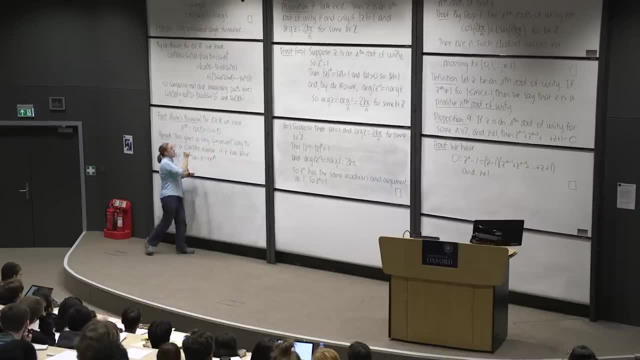 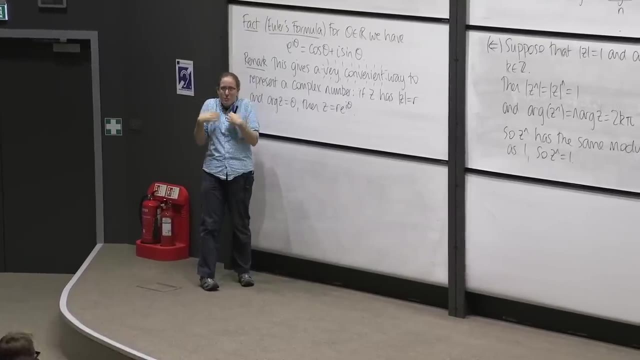 so I wanted to stress that this is very convenient, so I'm going to put flashing neon lights to remind you. so if this is relatively new, it feels a little bit uncomfortable. it feels natural to go back to your old ways of thinking about it. that's what we do when we meet. 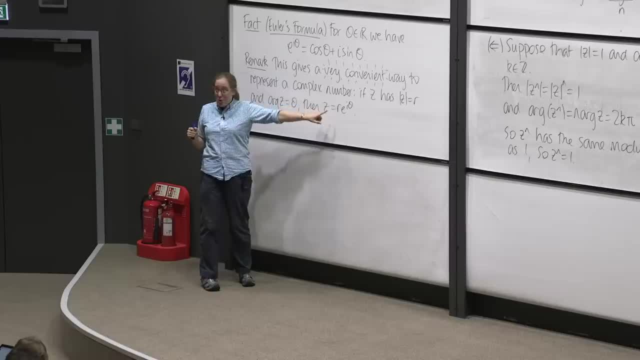 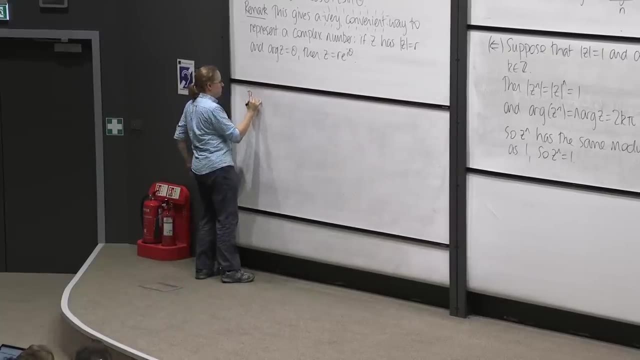 something new is kind of try to see: well, can we keep going with the old way? this has lots of advantages. I really encourage you to look for opportunities to practice working with this way of thinking about it so you become more fluent, for example, proposition 10. so 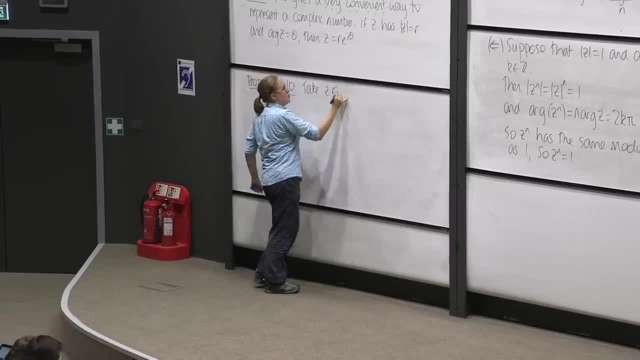 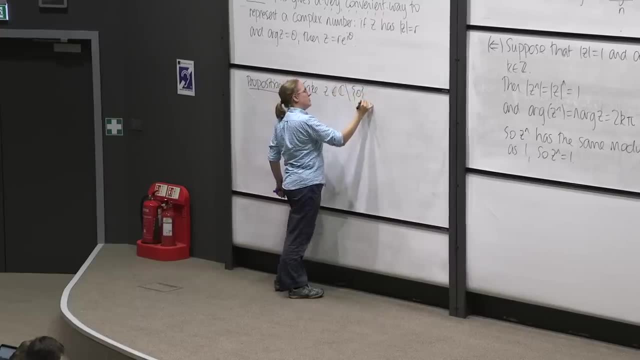 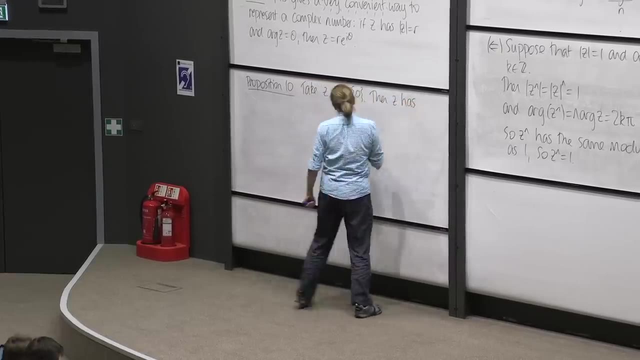 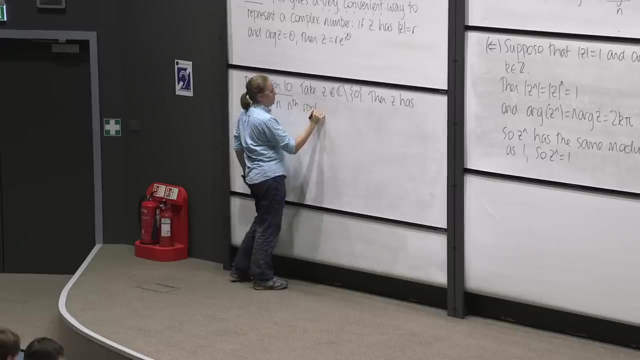 proposition 10 says: take z, a non-zero complex number, and you'll see why I want it to be non-zero. z in c, but not zero. that's a zero. then z has exactly n nth roots. so for any n is greater than or equal to 1. 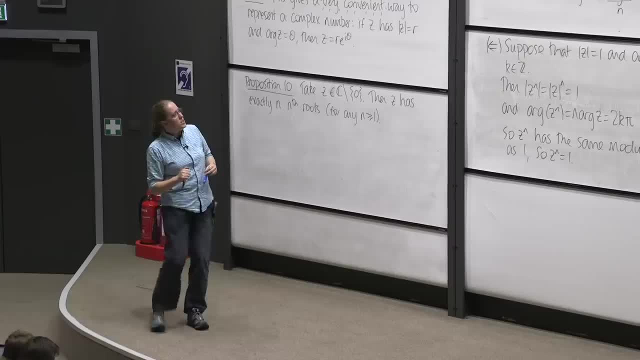 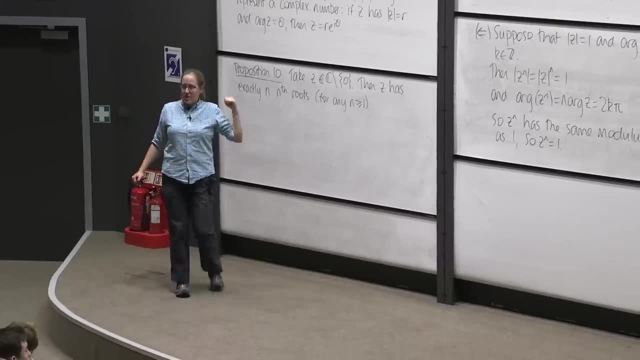 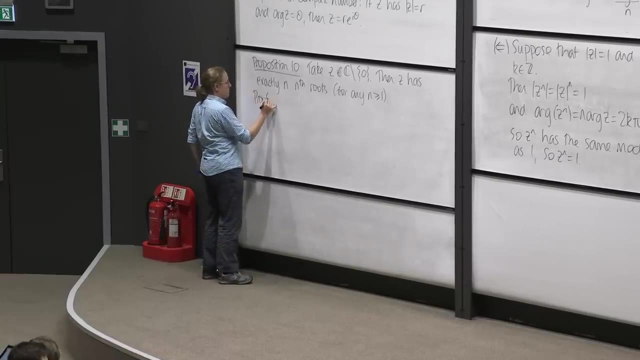 so we thought about roots of 1. right proposition: no, corollary 8, sorry said there are exactly n nth roots of 1. this is generalising to there are exactly n nth roots of any non-zero complex number, which is kind of nice. so let's prove this. 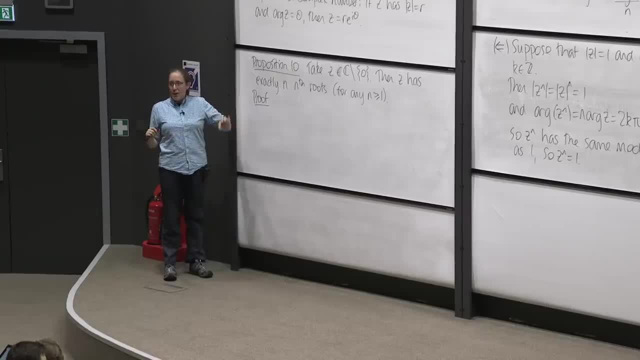 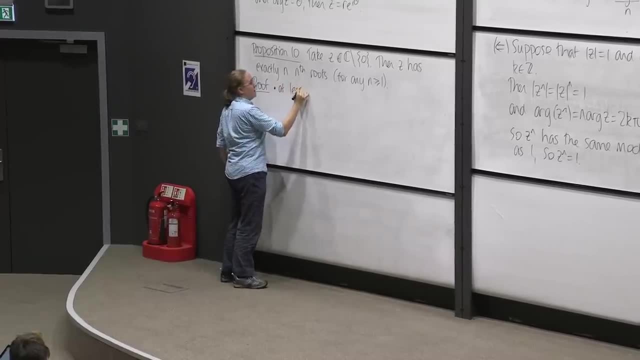 so I'm going to do this in three parts and I'm going to kind of bullet point what the sections are to try to help you see what the structure is clearly. so the first part is that there is at least one nth root. right at the start it's not completely clear. 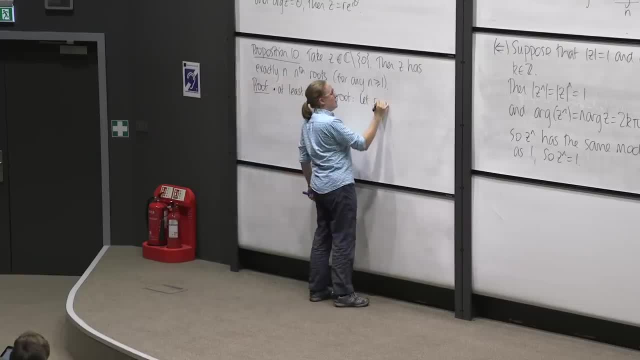 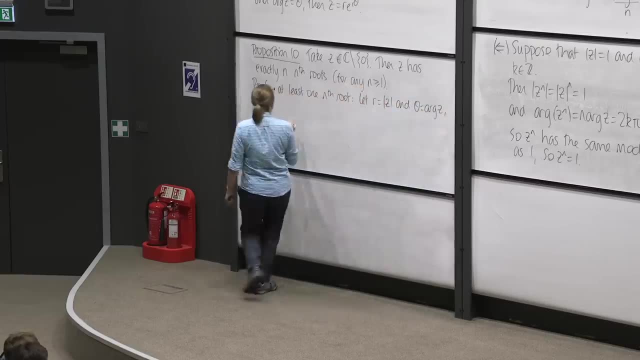 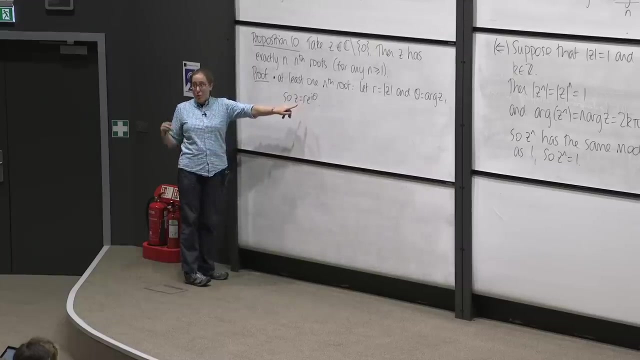 that there is at least one nth root. so if I let r be the modulus of z and theta be the argument of z, so z is r e to the i theta, I can sort of stare at z in this form and guess what an nth root might be. 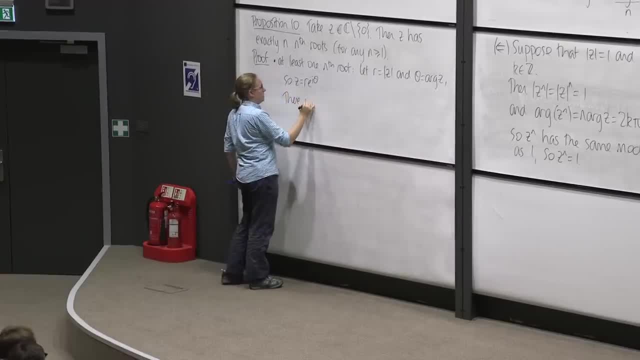 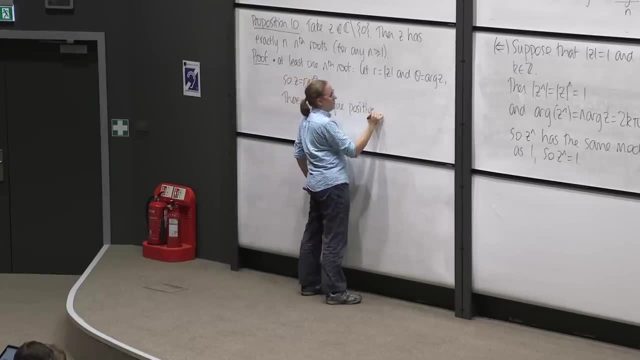 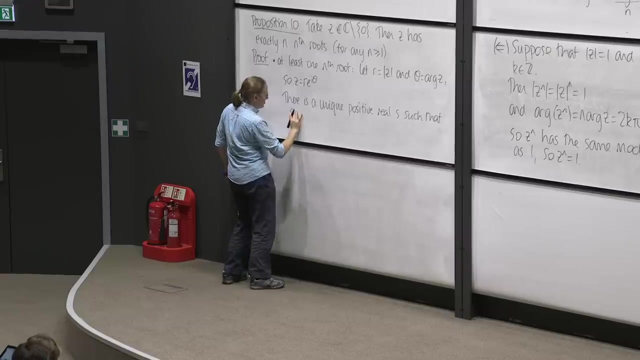 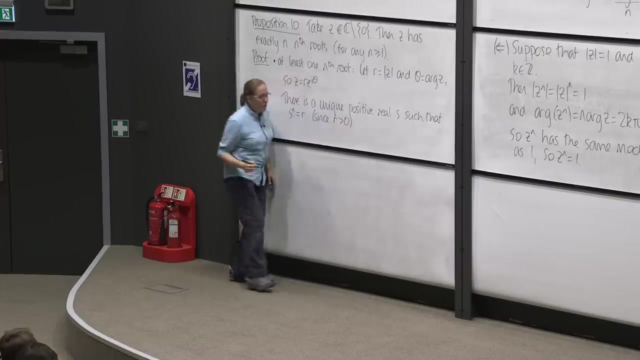 so there is a, in fact unique positive real s, such that s to the, s to the power, n is equal to r. so this is: since r is greater than zero. how do we know this is true? by analysis. so I'll just put c prelims analysis. 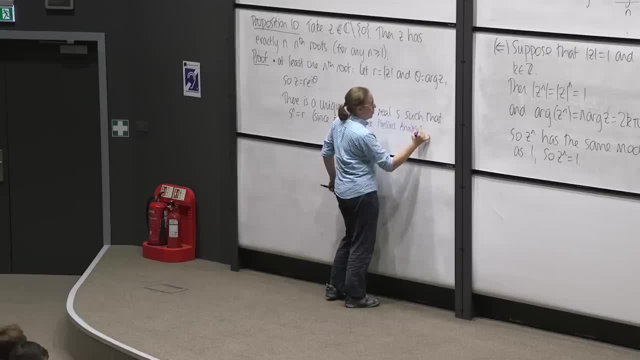 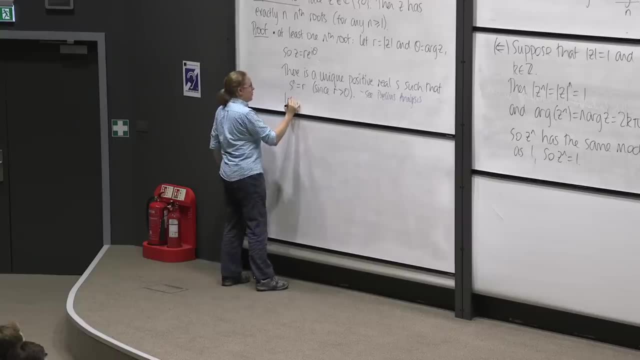 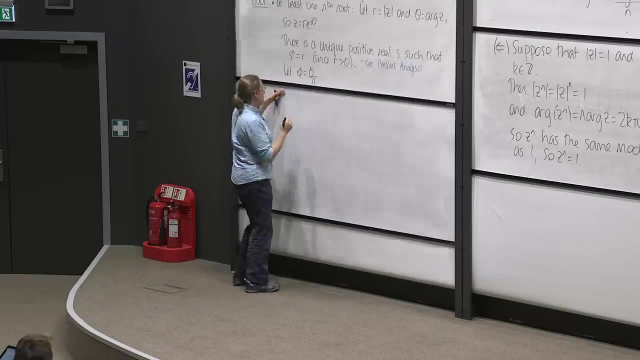 you will think about why you can do this in that course. so that's going to be the modulus of my proposed root. and now I'm going to let phi equal theta over n. where did I start over here? yeah, it's okay. so if I let w be equal. 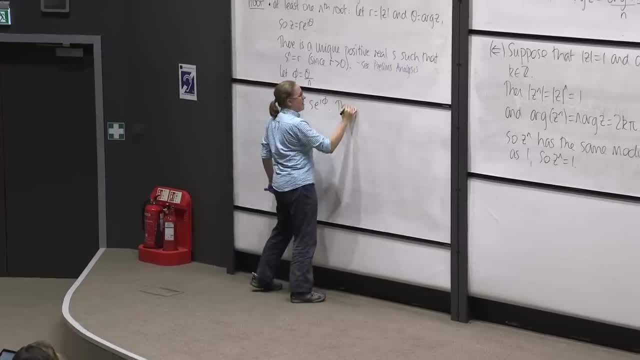 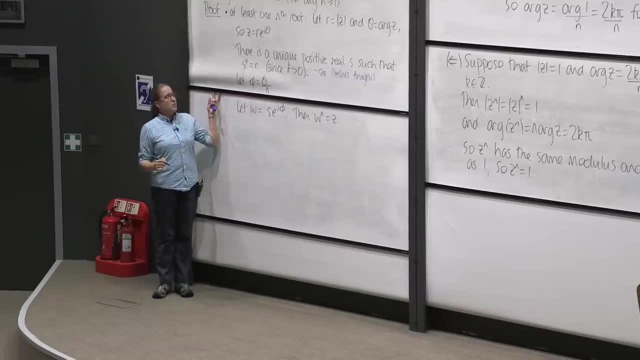 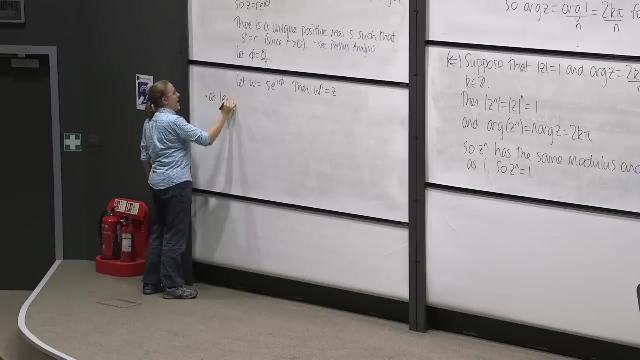 to s, e to the i phi, then w to the n. when you do a quick calculation, you see is equal to z, so there's definitely at least one root. now I'd like to show that there are in fact at least n nth roots. how do you show that there are exactly n of? 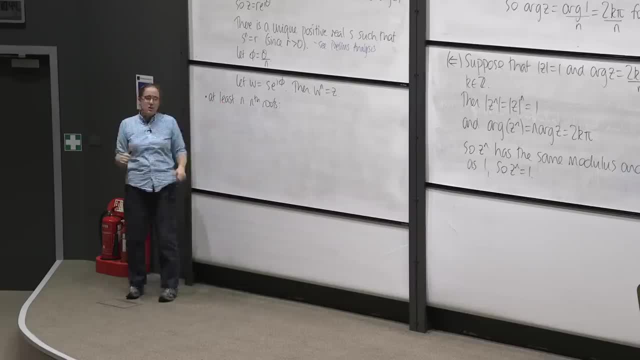 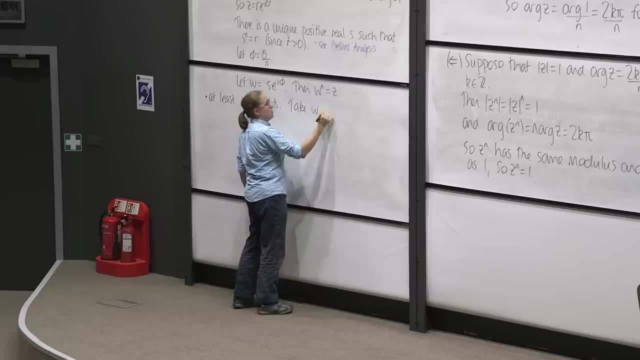 something you show there are at least n of something you show there are at most n of something that could be a useful strategy. so I want to show that there are at least n roots. so I'm going to take w as above. so w is a fixed nth root. 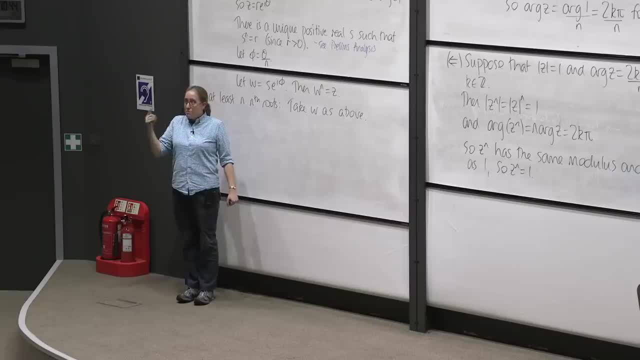 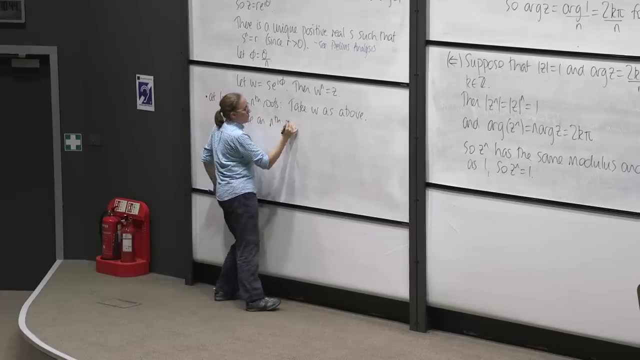 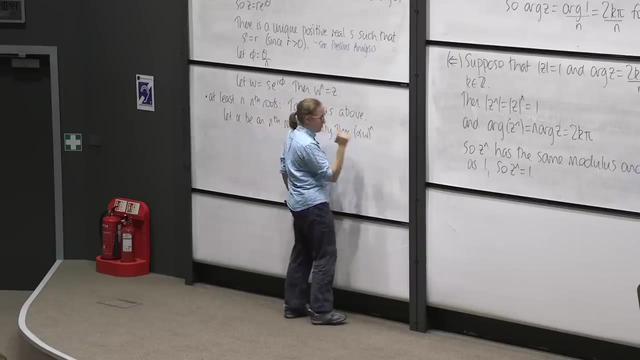 I could get a whole bunch more nth roots by multiplying by an nth root of one. so if I let alpha be an nth root of unity, then you do a quick calculation and you realise that alpha times w to the power n is also equal to z. so alpha w 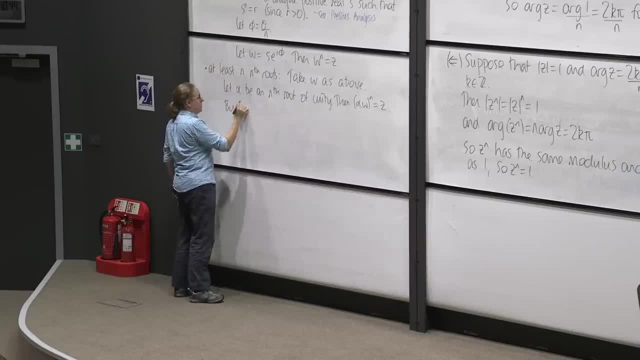 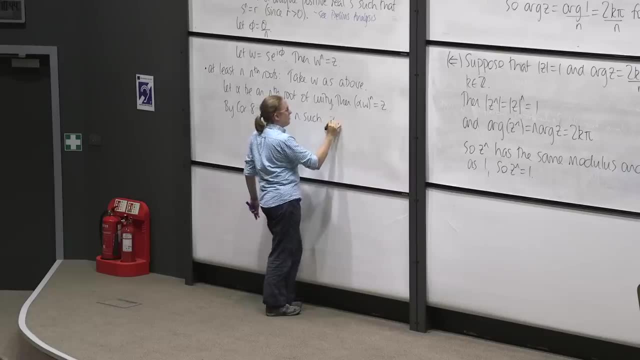 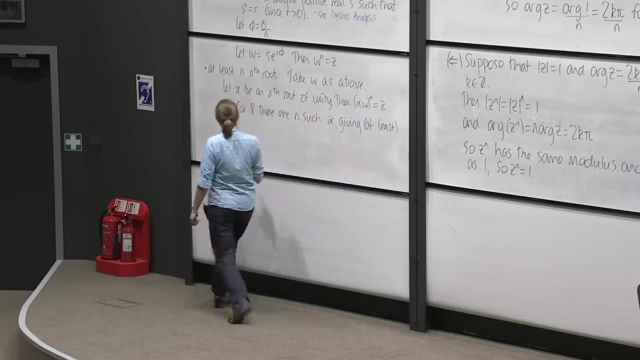 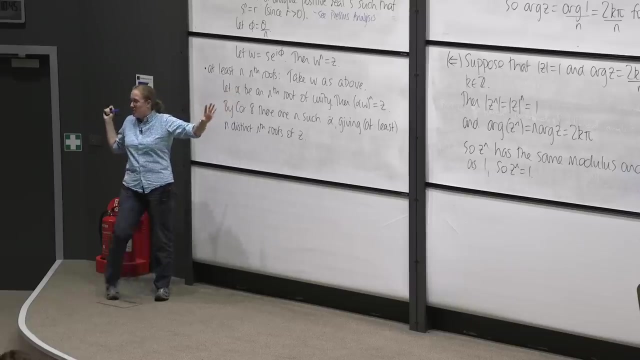 is another root of z, and by corollary eight there are n such alpha giving. well, at least n distinct nth roots of z. so this says I can think of n distinct nth roots of z. we haven't shown that there aren't some more. maybe there are some more that have some other. 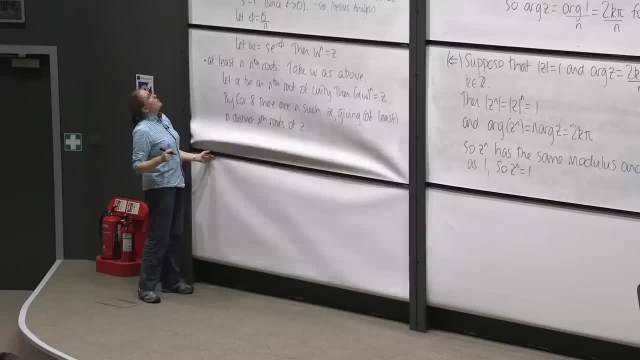 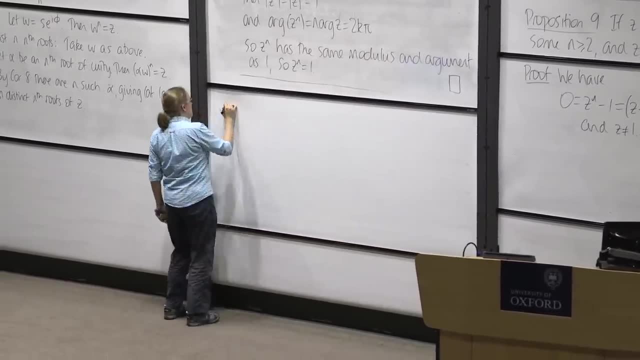 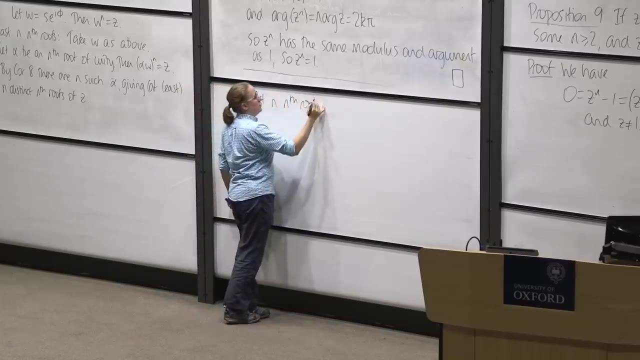 form? of course there aren't. that's what we're about to prove, but that's why we're kind of structuring it like this. so if I carry on over here for the third bullet point, the third bullet says at most n? nth roots. so if I again take w as 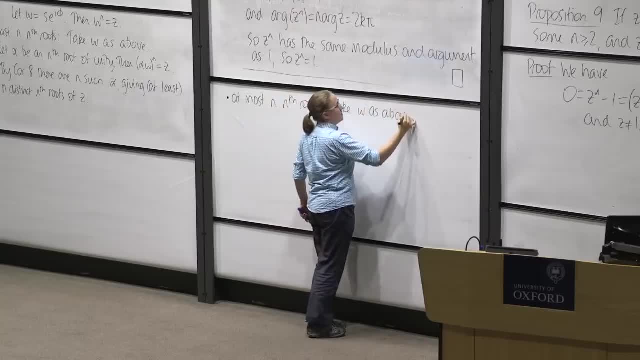 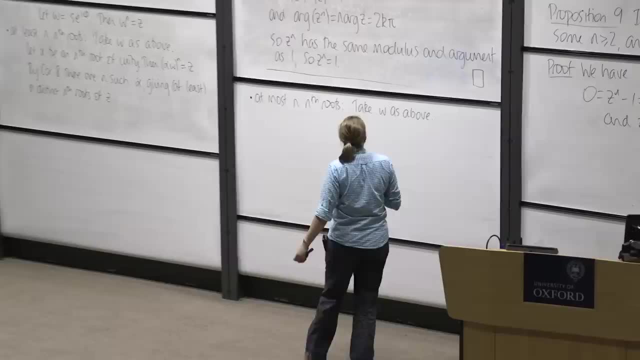 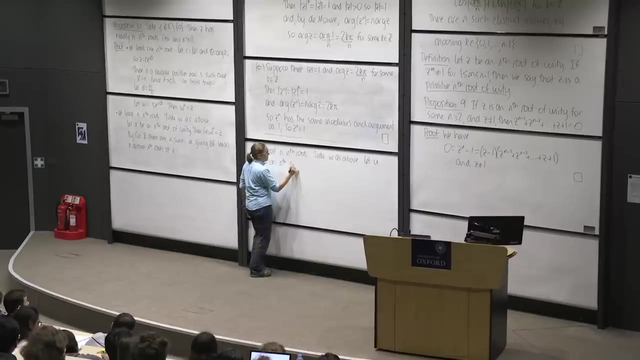 above. so w is my fixed nth root of z. I want to show that any nth root of z must be a root of one times w. that would do it. so if I let u be an nth root of z, then my secret aim, if you like, is to show that u must be. 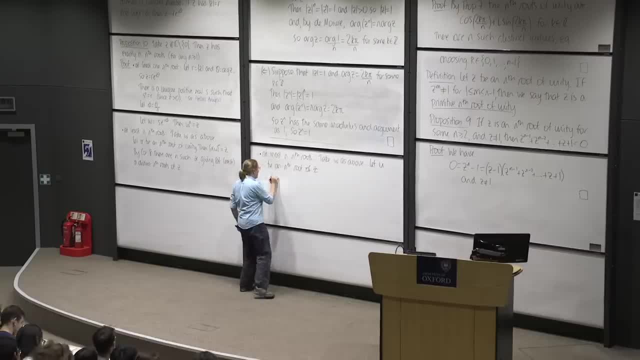 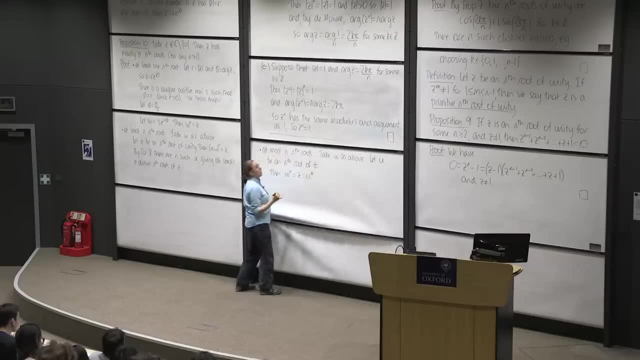 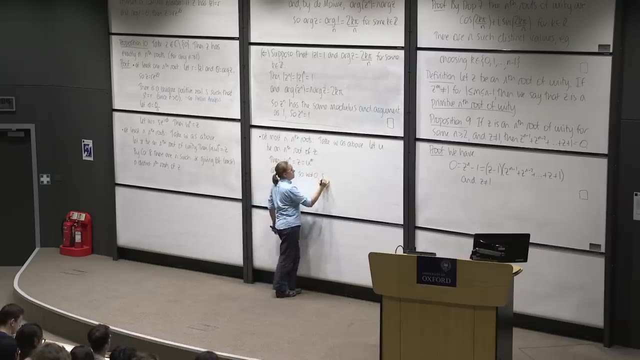 w times some nth root of unity. well, we know that w to the n is z and that's also u to the n. that wasn't a very good n. let me try again. and z is not zero, so w is not zero, so I can do u divided by. 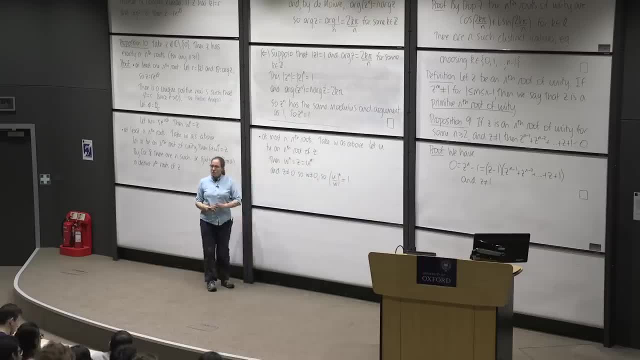 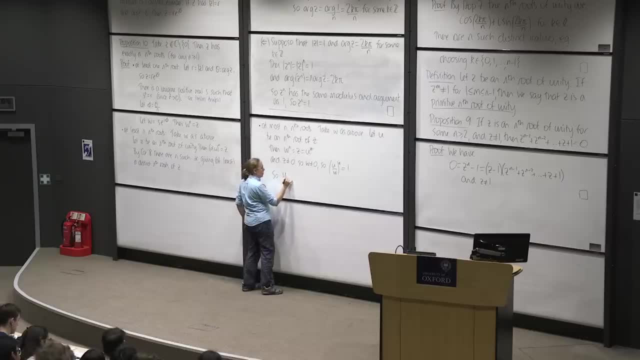 w to the power n, and that's now one right, having got u to the n, and w to the n are the same. if I just rearrange, this says that u over w is an nth root of one and by corollary eight there are n of these. 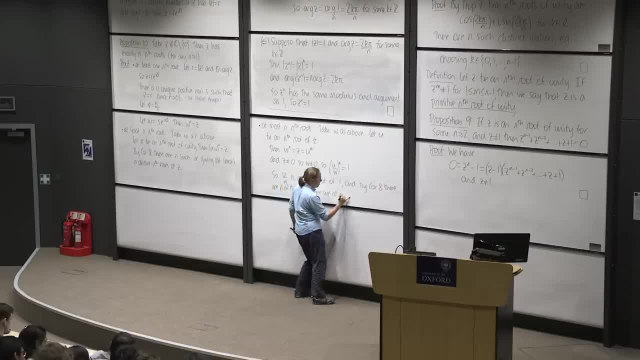 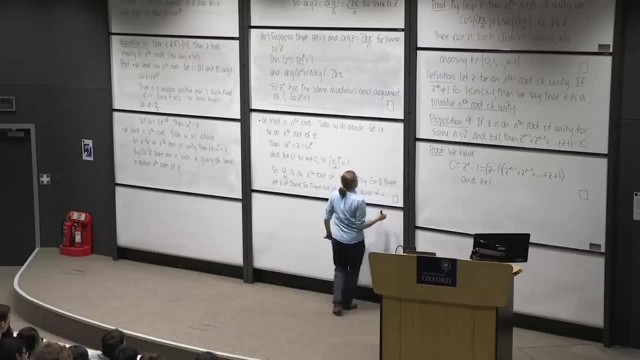 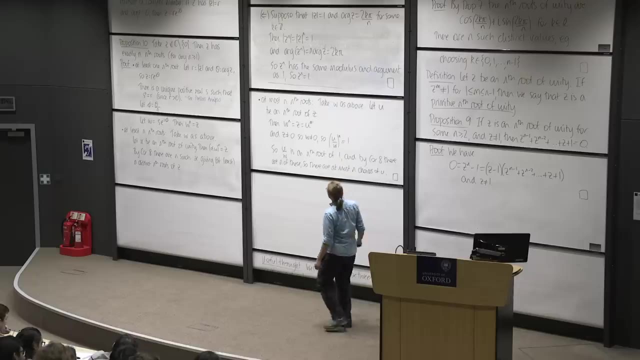 so there are at most n choices of u. so that completes the proof. so it's a little bit fiddly and you might want to kind of think about that in your own time, but hopefully the structure at least makes some kind of sense. so that was thinking about. 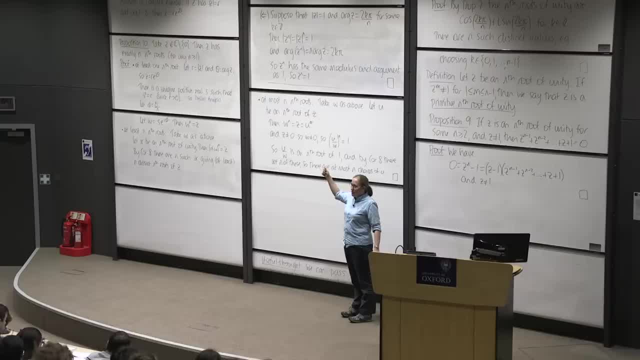 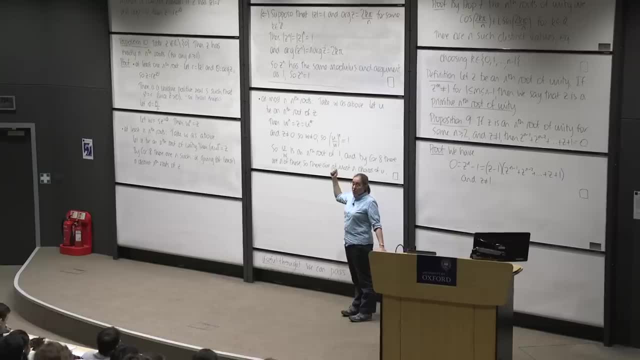 roots of a particular complex number. and that means that we've sort of thought about solutions to the polynomial equation w to the n equals z. we've just counted solutions to that equation. we'd like to know about solutions to polynomials more generally. I said on Monday we could think about solutions to. 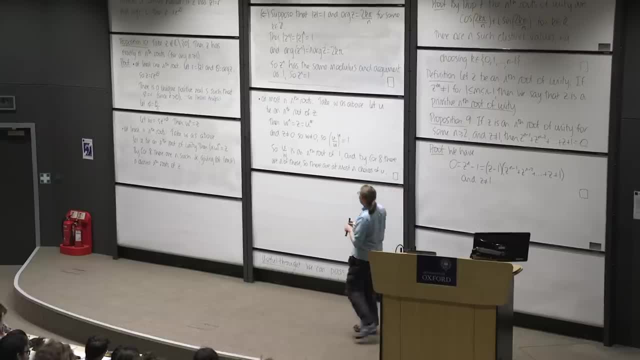 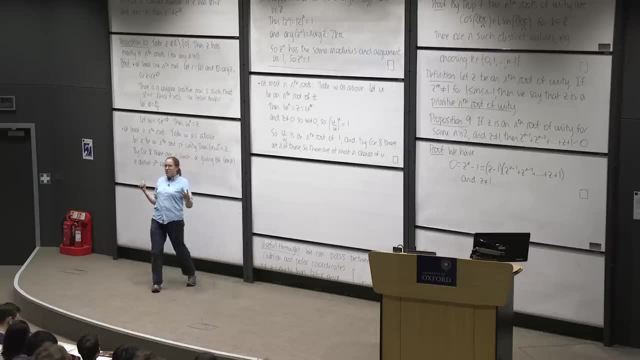 quadratics and we'd like to be able to generalise, and that's what we're going to do now. so the first thing is to show that if you've got a polynomial with complex coefficients, a complex polynomial of degree n, then it can't have too many roots. 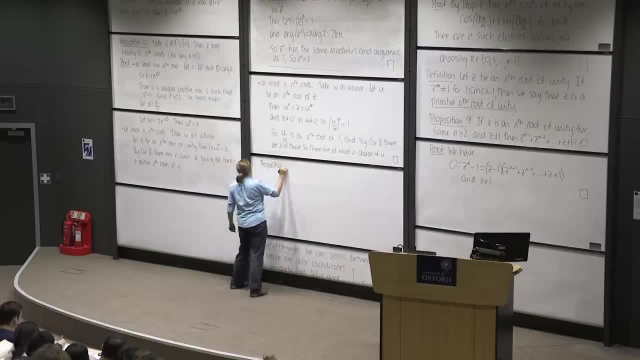 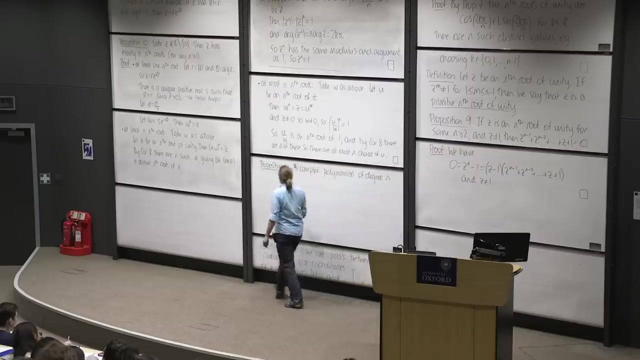 so this is proposition eleven, and this says a complex polynomial, meaning a polynomial with complex coefficients of degree n, has at most n roots. I mean, maybe it has no roots, maybe it has some roots. I'm not making any claims about that in this proposition. all I'm saying is there are at most 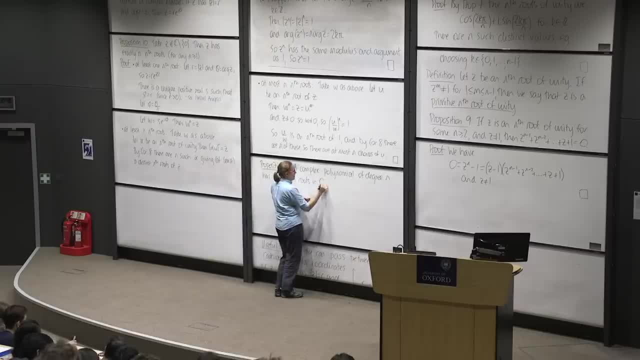 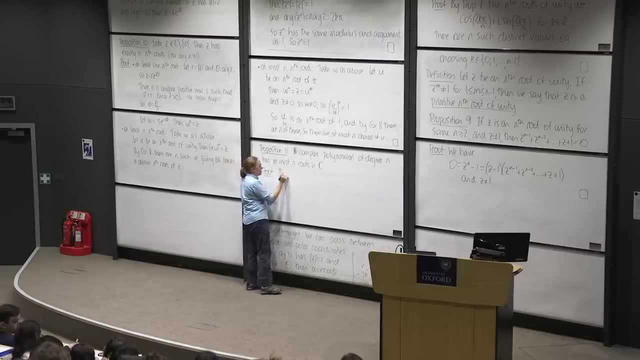 n complex roots, so I mean n roots in c. so let's prove this and my strategy is going to be to use induction on n, the degree of the polynomial, so n is one, for example, as a base case. that's a quick check. I'll let you make sure that you're 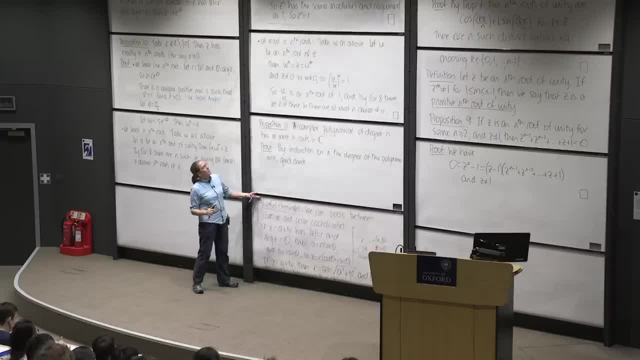 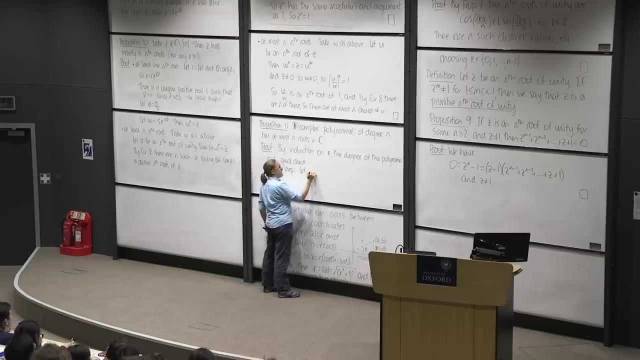 happy to see that a linear polynomial with complex coefficients has at most one root. I feel confident that you can handle that, so let's do the inductive step. so I'm going to let p be a complex polynomial with degree n and I'm going to suppose: 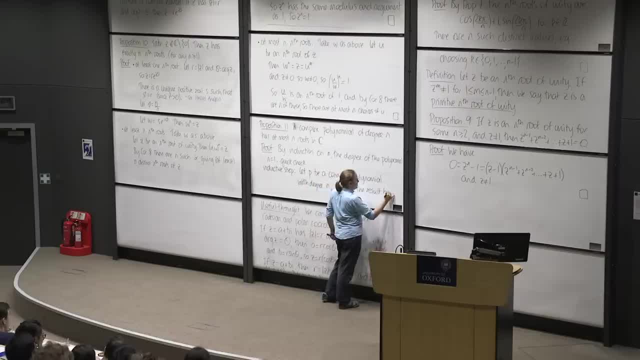 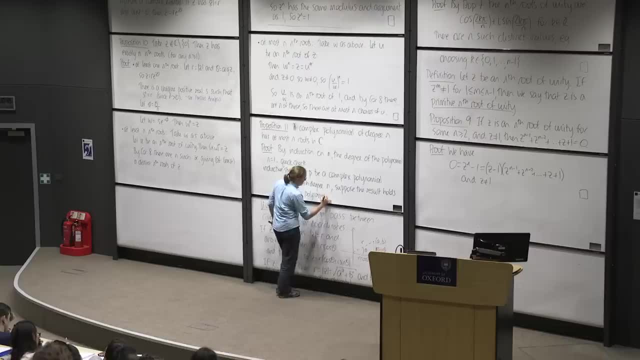 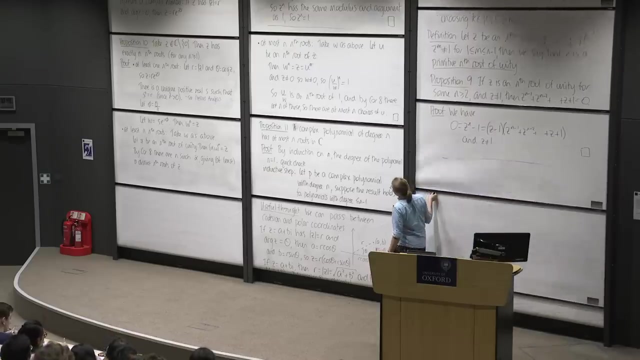 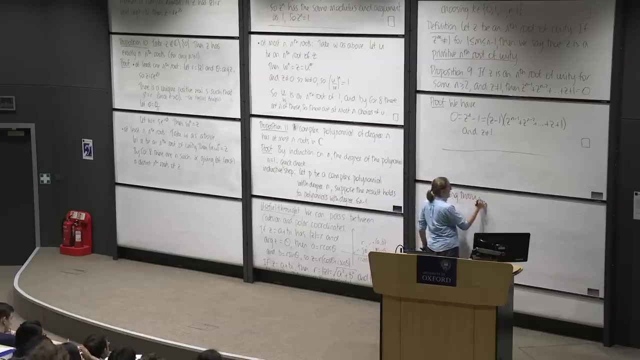 the result holds for polynomials with degree less than or equal to n minus one. that's our inductive hypothesis. so I want to show that the number of roots of p can't be too big, dividing the through by the leading coefficient, the coefficient of z to 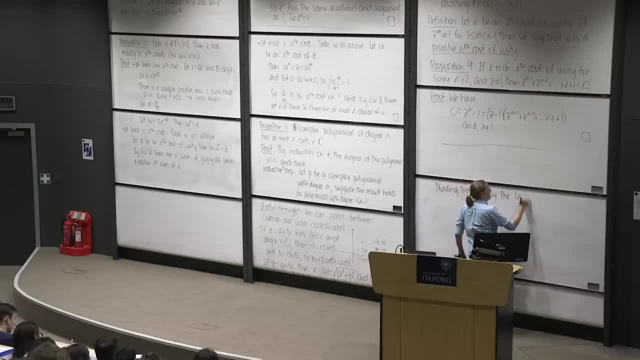 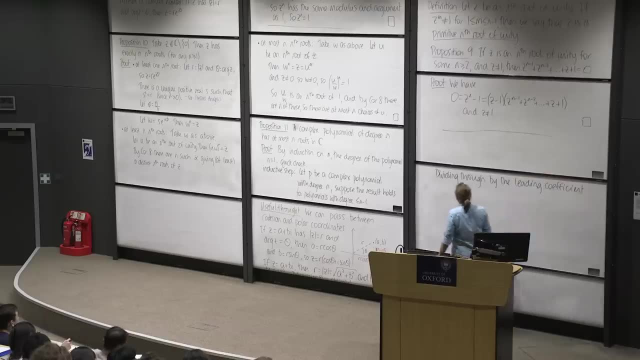 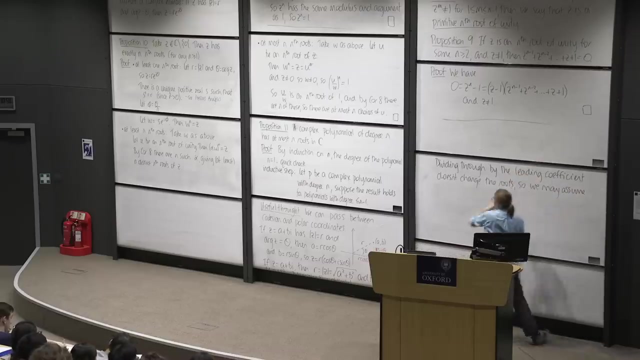 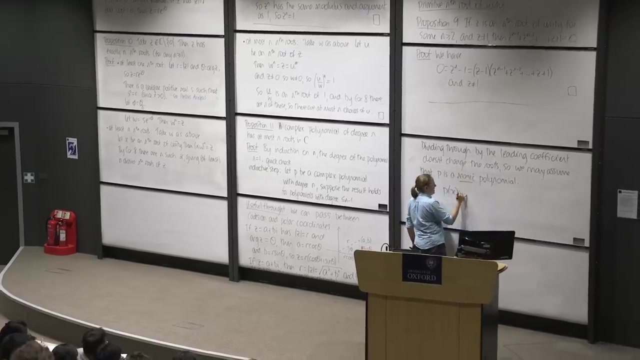 the n, if you like, by the leading coefficient. x to the n maybe doesn't change the roots, and what that means is that we may assume that p is a monic. polynomial monic means it has leading coefficient one, so p looks like p of x is x to the n. 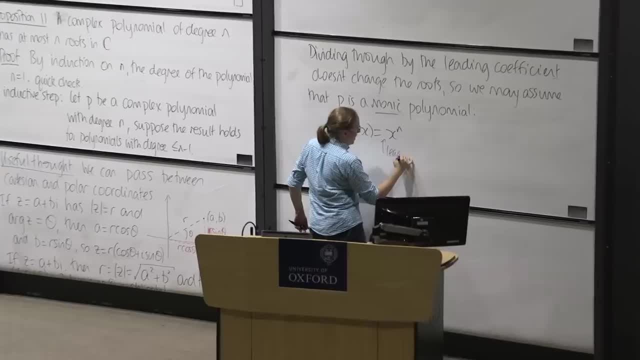 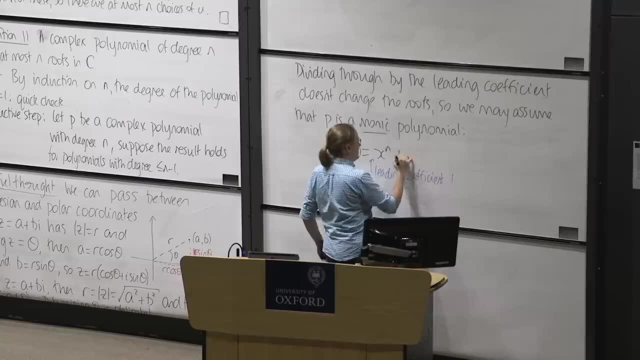 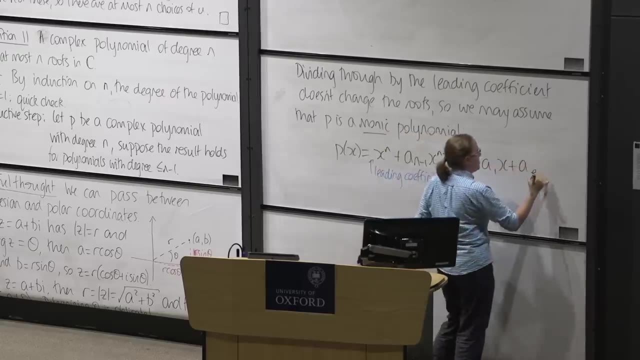 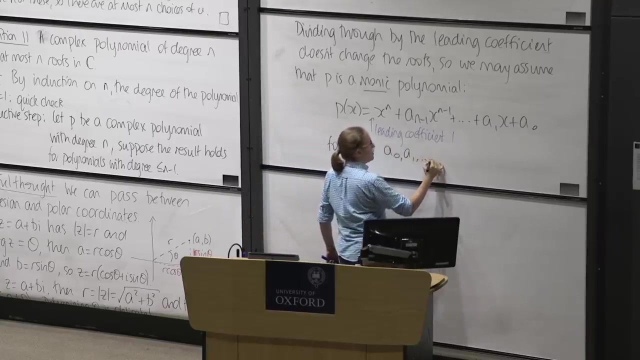 it has leading coefficient one because it's monic, uh plus a n minus one x to the n minus one plus dot dot dot plus a one x plus a zero, for some a zero a one dot dot dot a n minus one in c. I would like you to notice. 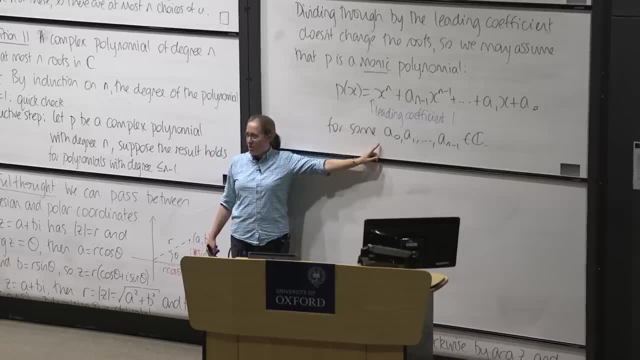 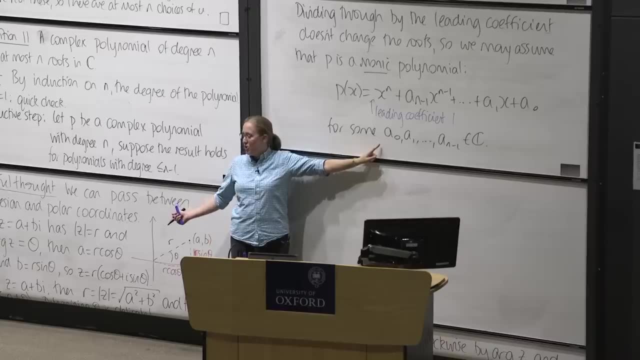 two things about this. one is that I've very carefully introduced what a zero up to a n minus one are. if you turn up at a party and you take your friend along and they don't know the people there, you introduce them right. it's really rude not to, because otherwise people can't. 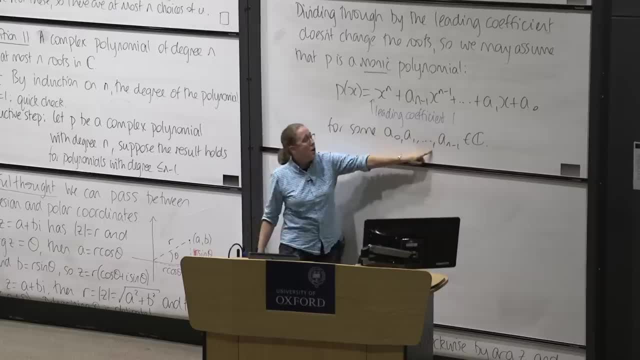 have a kind of sensible conversation. we can't talk about these things without knowing what they are. also notice how I've carefully matched the coefficient with the power, so that it's dead easy to do. I didn't want to start with a zero or a one here, right? 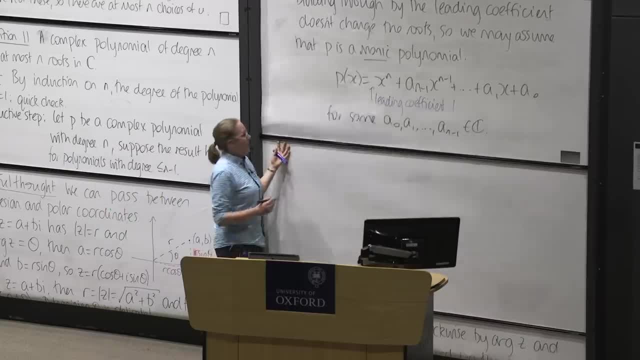 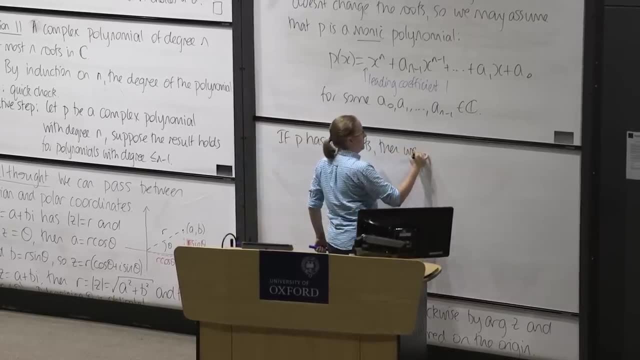 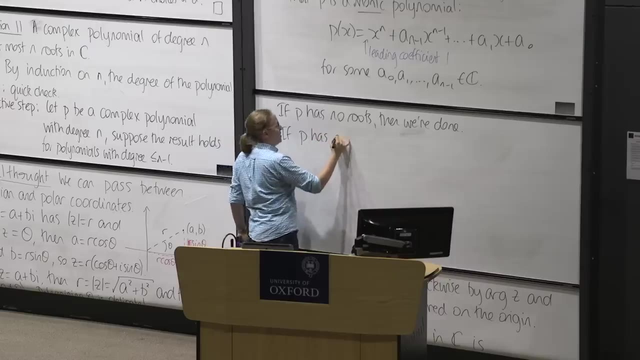 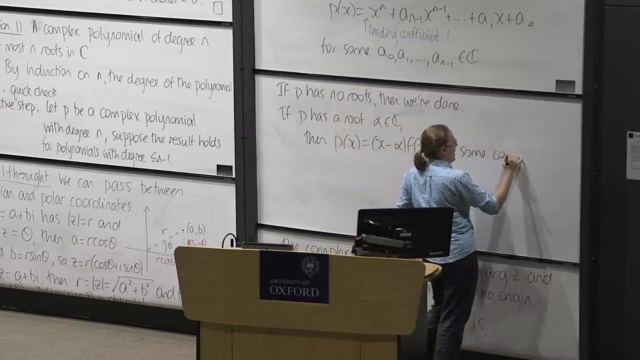 this is a top tip. this will make your life easier. if p has no roots, then we're done. if p has a root, say alpha in c, then p of x is equal to x minus alpha times f of x. for some complex monic polynomial f with degree n minus one. 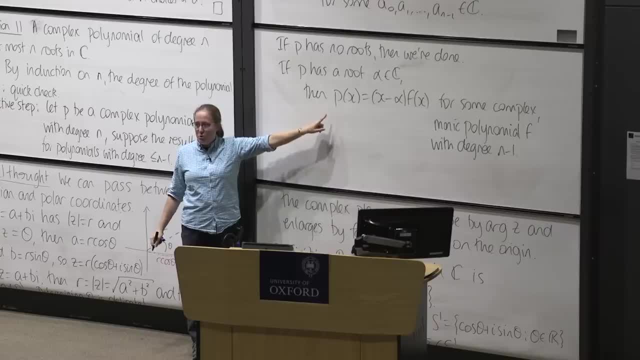 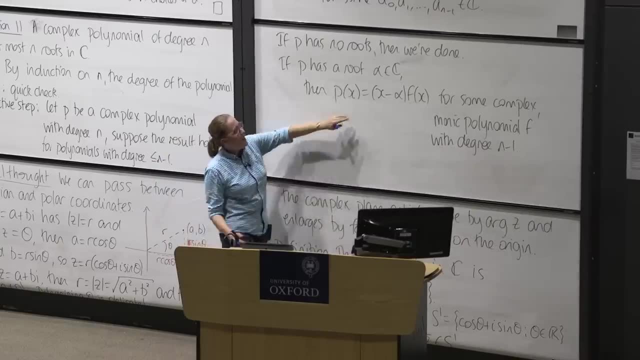 if you haven't seen how to prove this or you're not more to the point, you're not confident you could do yourself. I did put the details in the online notes, so if you want to think about that, you can. what this tells us is that any root of p is 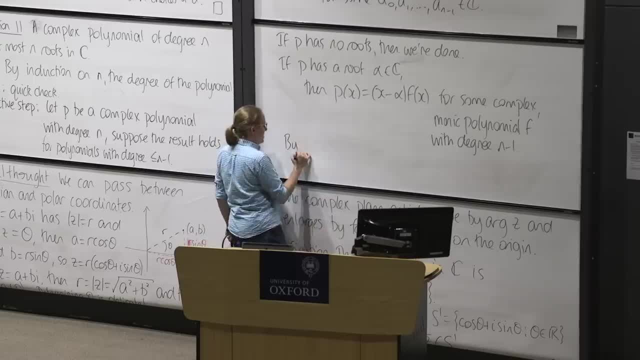 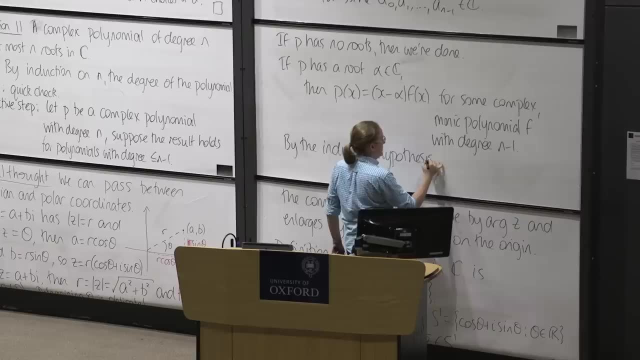 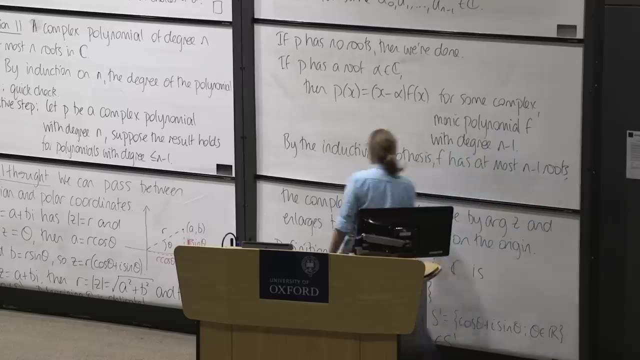 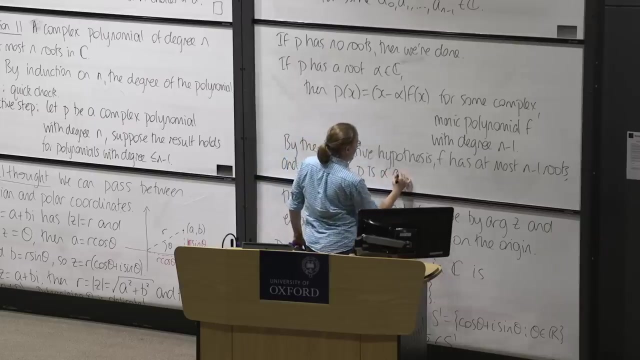 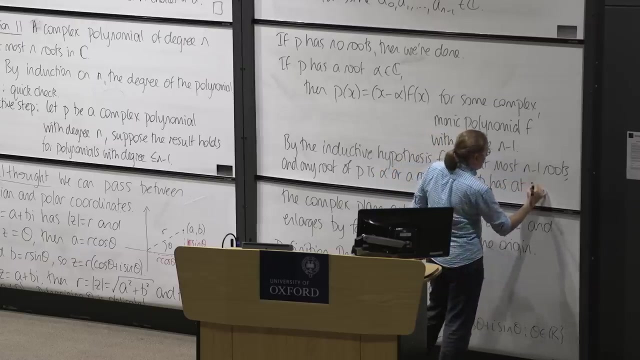 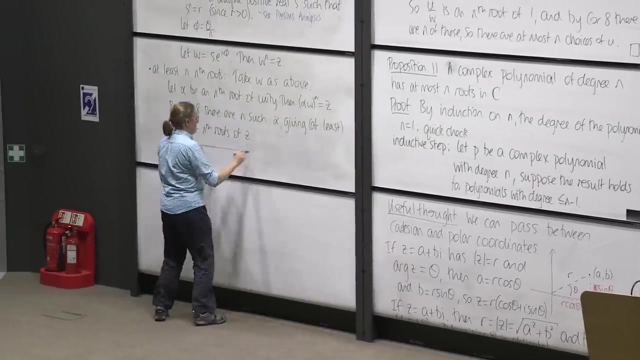 either alpha or a root of f. so by the inductive hypothesis f has at most n minus one roots, and any root of p is alpha or a root of f. so p has at most- ok, I need to carry on over here- p has at most n roots. 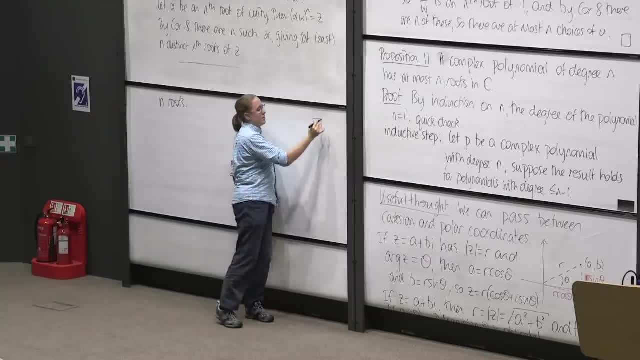 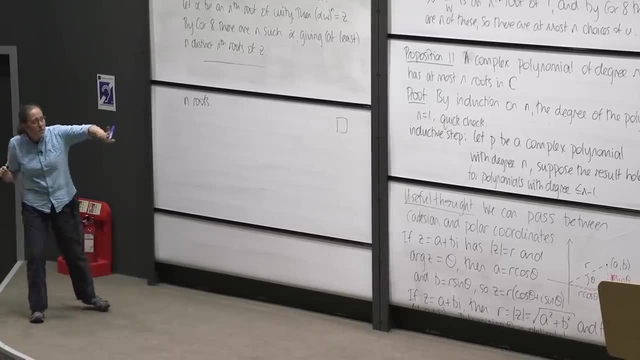 and that completes the induction argument. so proving that a complex polynomial of degree n has at most n roots is not too difficult. I mean, I've gone through that fairly swiftly. you're going to want to look at that in your own time, but it's very doable. 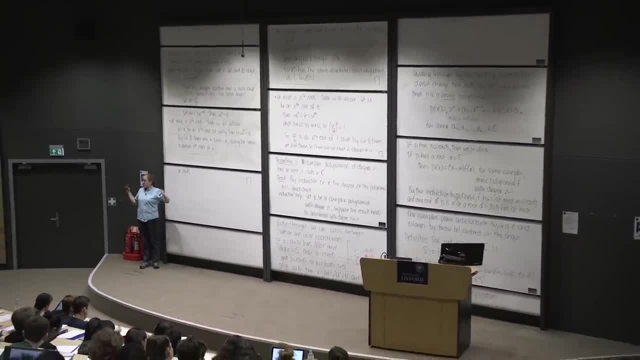 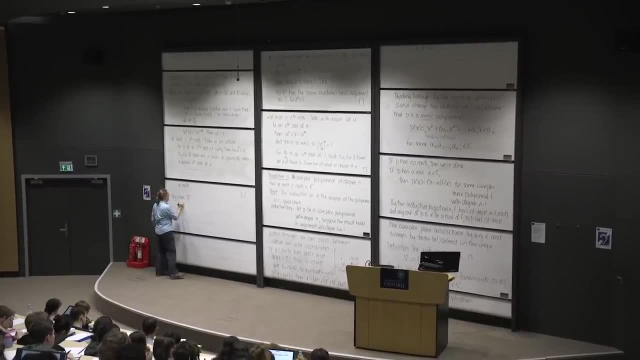 what we'd really like to know is: does it have any roots? does it always have at least one root? does it always have n roots? and the answer is given by theorem twelve, which is super important, and it's called the fundamental theorem of algebra. you should draw some conclusions. 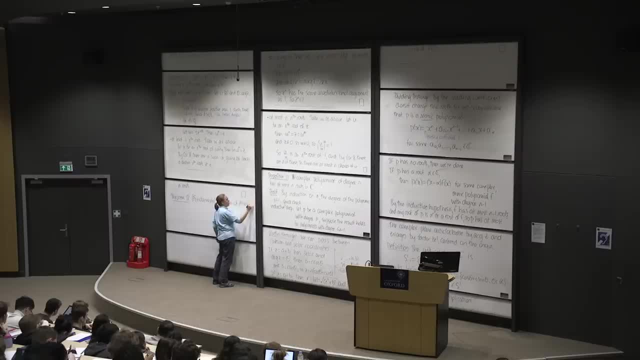 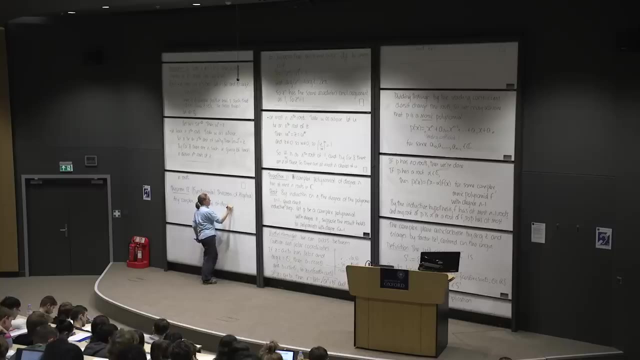 about the importance of this theorem from the fact that it's called the fundamental theorem of algebra. and this says any complex polynomial of degree n has exactly n roots counted with multiplicity. so repeated roots, you have to count the appropriate number of times which, when you sort of think about it, 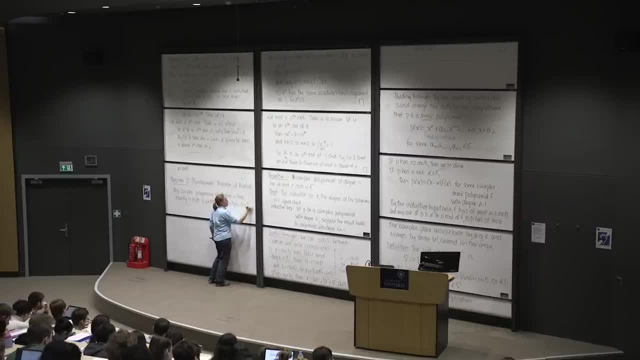 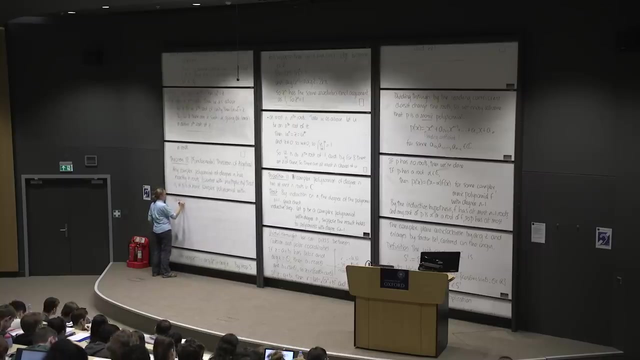 is a relatively natural thing to do. so, that is, if p is well, we may as well focus on a monic, complex polynomial with degree n. then we can factorise: p of x is x minus alpha one up to x minus alpha n for some alpha one.